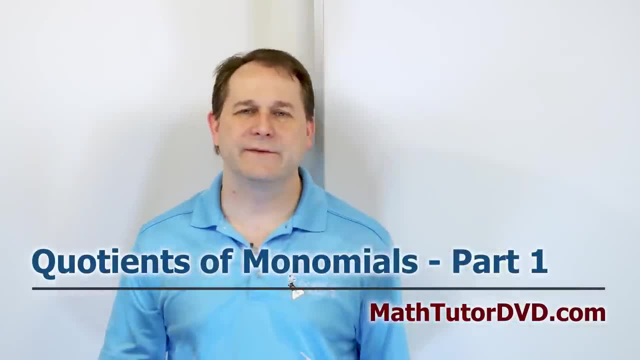 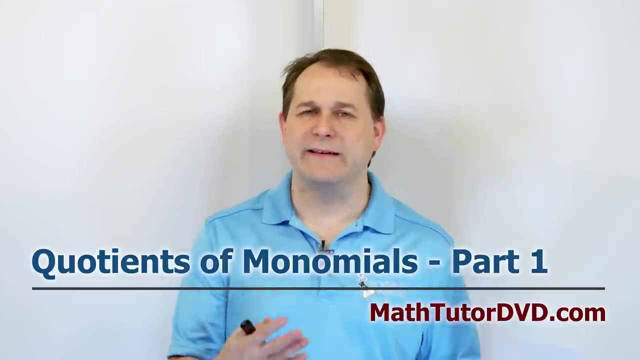 Hello, welcome back to Algebra. The title of this lesson sounds very intimidating, but actually it's very, very simple to understand once we get some problems under our belt. The title that you might see in the textbook for this would be called Quotients of Monomials. 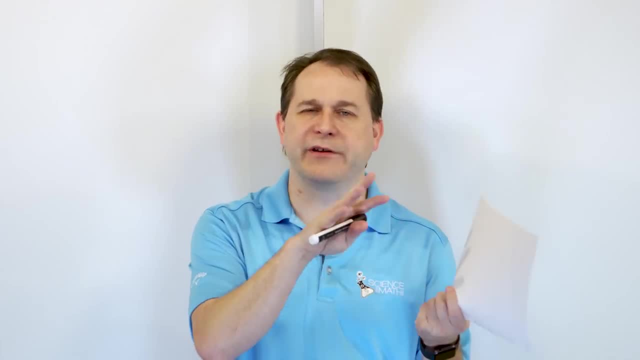 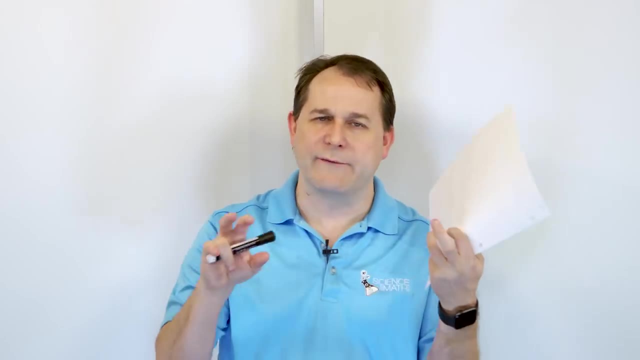 So remember, monomials are long strings of terms that have numbers and also exponents and variables. So we'll have quotients of those guys. We'll be dividing them with the large fractions. on the top of the numerator, We'll have a monomial. on the bottom, We'll 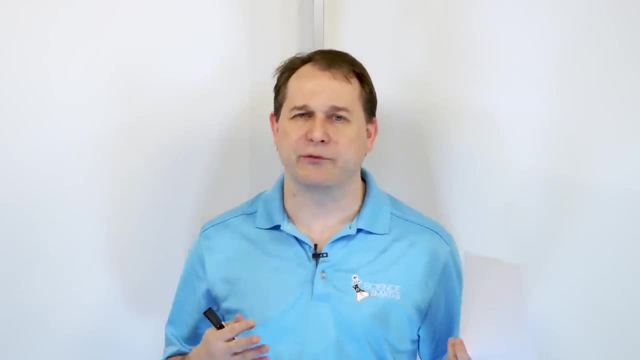 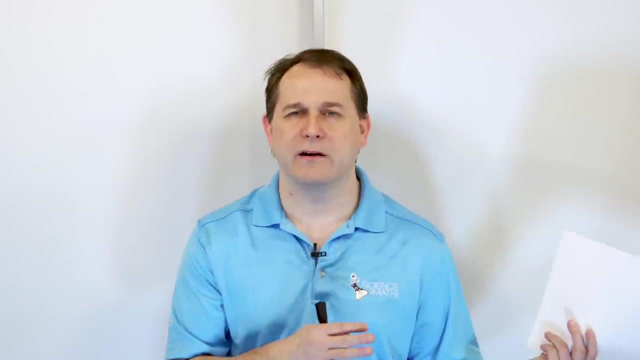 also have another monomial, And so, because we have a lot of exponents running around in these expressions, we'll need to be using the laws of exponents that we've already learned in the past. So if you haven't already gone and learned and understood my laws of exponents, 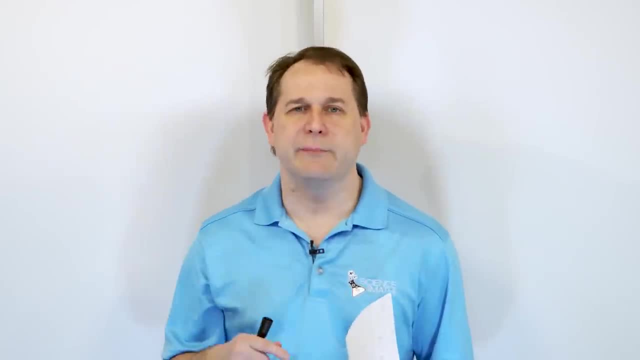 lesson. please do that now. Otherwise what I'm going to do here in the beginning is just do a quick recap of laws of exponents really fast, just to get them on the board, And then we'll be using every one of these laws as we do our problems Now, even though the title 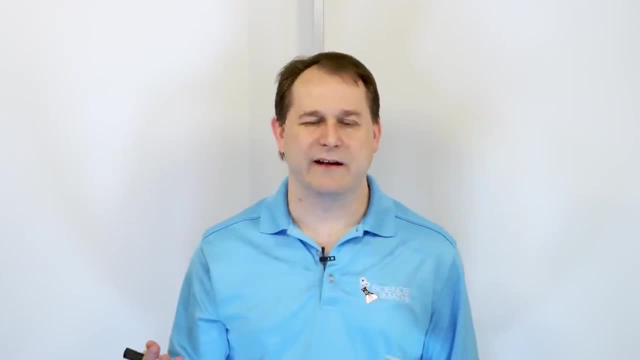 of this could be called Quotients of Monomials. what I like to think of the title, of the title of this lesson, is something a little easier to understand, which would be Simplifying Expressions that Involve Fractions and Exponents. So, lots of fractions, lots of exponents. Let's go. 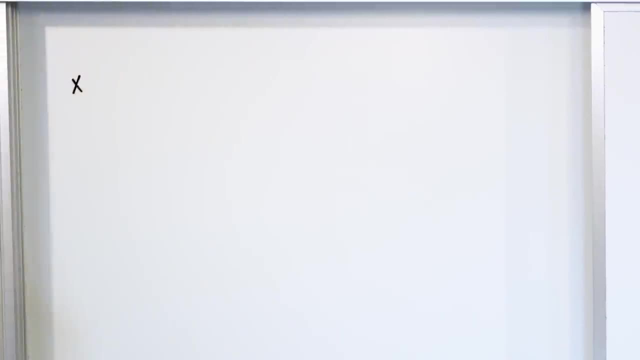 over here and talk about laws of exponents. So the very first law of exponents that we typically talk about is when you have a variable raised to a power- In this case let's just call it the second power times- a variable with the same exact base raised to a different. 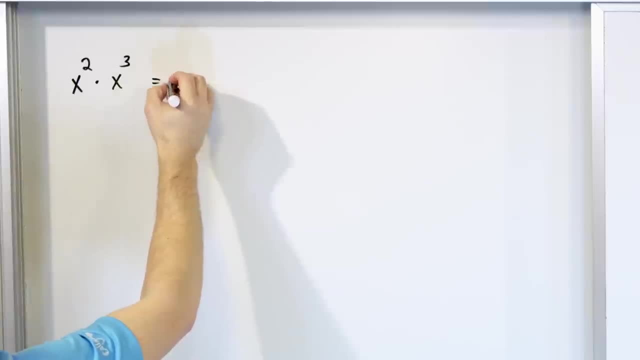 power. So same base, different numbers. So what we do here is we add these together, Two plus three. here We add them, which is x to the fifth power. This should come as no surprise, And the reason this works is because this is x times x and this is x times x times x, So they're all multiplied together. 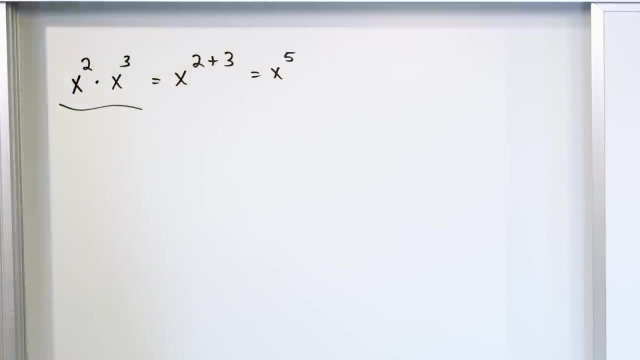 and there's five of them And that's why we add them together. So that's what happens when you have two terms multiplied together with the same base. Now we turn our attention What happens when we divide terms. So, for instance, if we have x to the third divided. 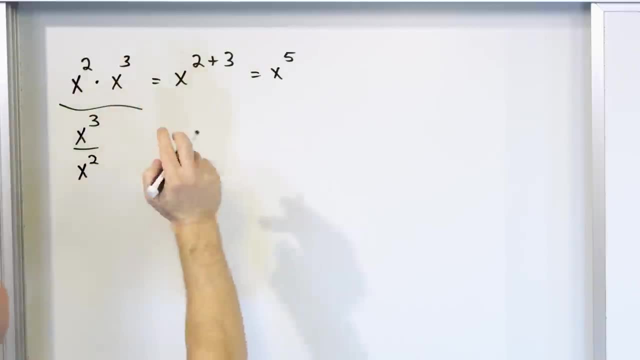 by x squared, The exponents in this case. Well, in this case, what do we do? We take the top exponent and we subtract the bottom exponent from it, So three minus two, which, as you all know, is x, to the first power which, as you all know, is just x. So it's very simple to see. 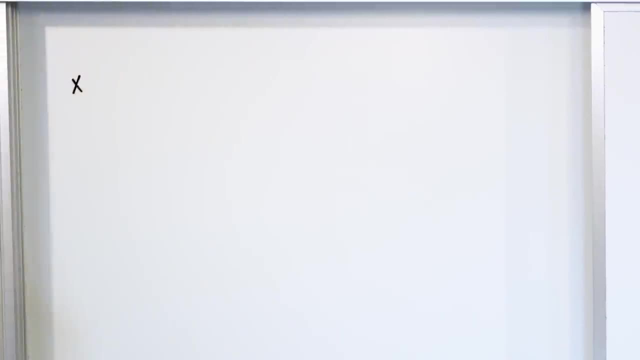 over here and talk about laws of exponents. So the very first law of exponents that we typically talk about is when you have a variable raised to a power- In this case let's just call it the second power times- a variable with the same exact base raised to a different. 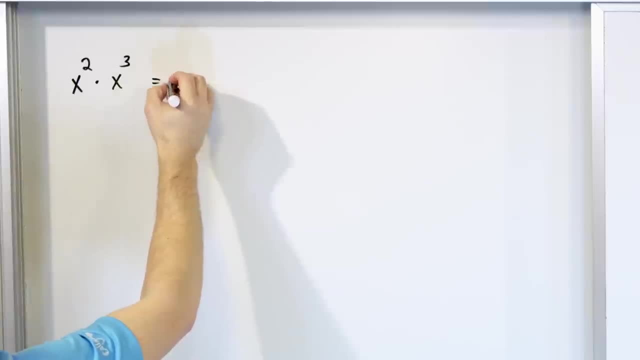 power. So same base, different numbers. So what we do here is we add these together, Two plus three. here We add them, which is x to the fifth power. This should come as no surprise, And the reason this works is because this is x times x and this is x times x times x, So they're all multiplied together. 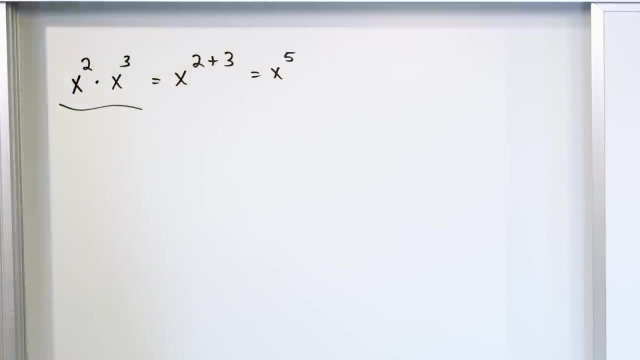 and there's five of them And that's why we add them together. So that's what happens when you have two terms multiplied together with the same base. Now we turn our attention What happens when we divide terms. So, for instance, if we have x to the third divided. 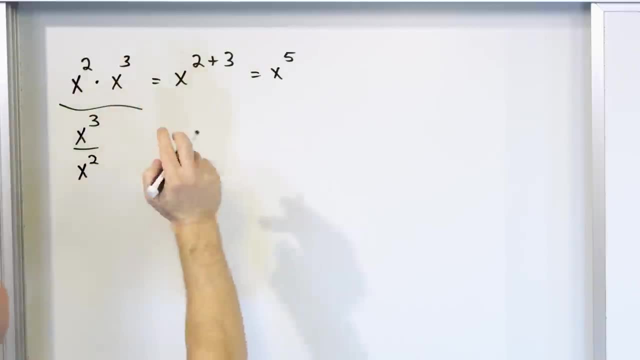 by x squared, The exponents in this case. Well, in this case, what do we do? We take the top exponent and we subtract the bottom exponent from it, So three minus two, which, as you all know, is x, to the first power which, as you all know, is just x. So it's very simple to see. 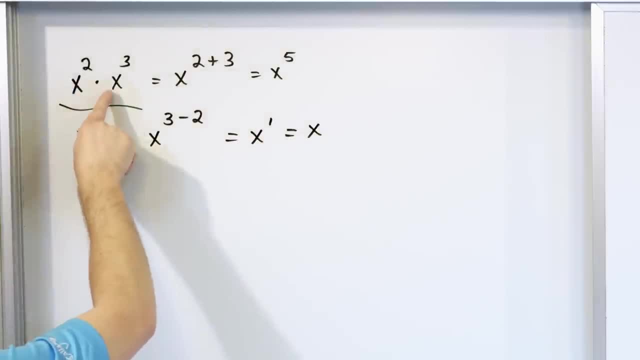 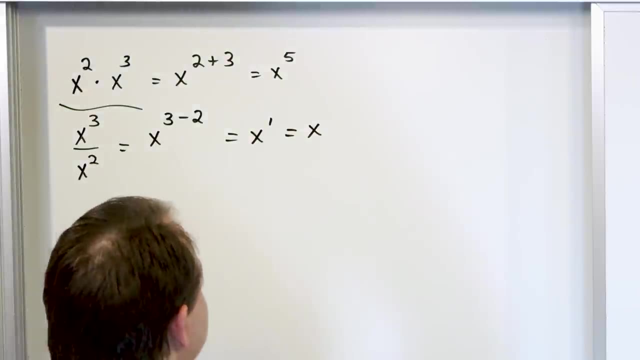 the symmetry here, once you get it all in one place, When you have the same base, different exponents, you multiply, you just add the exponents. When you divide, you subtract the exponents. Now, in general terms over here, I'll put another column here, general, And this is: 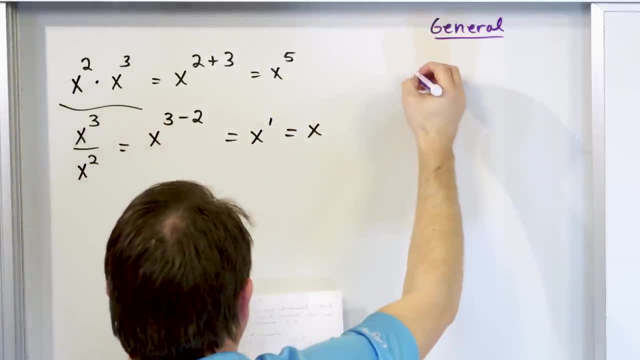 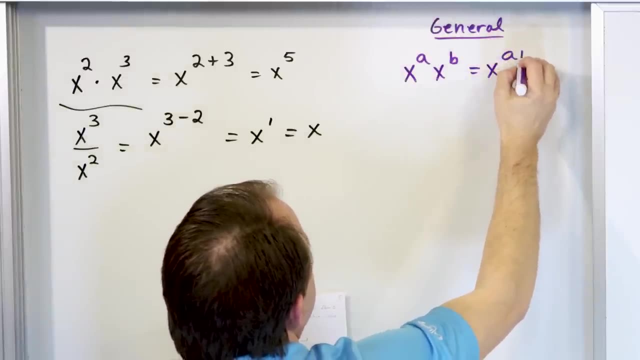 what you might see in a textbook. So for this first rule, what you might see in a textbook would look a little more formal. It might say: x to the a times, x to the power of b equals x to the a plus b. All this means is we add the exponents, just like I'm showing you with. 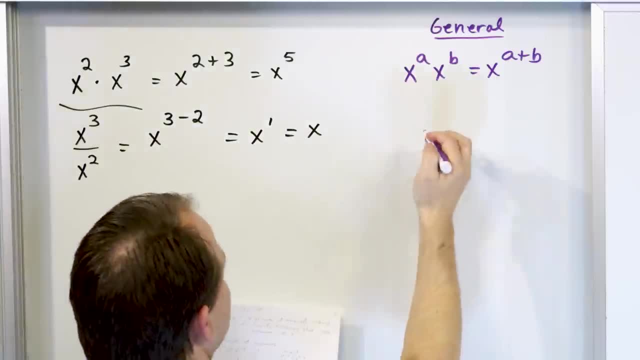 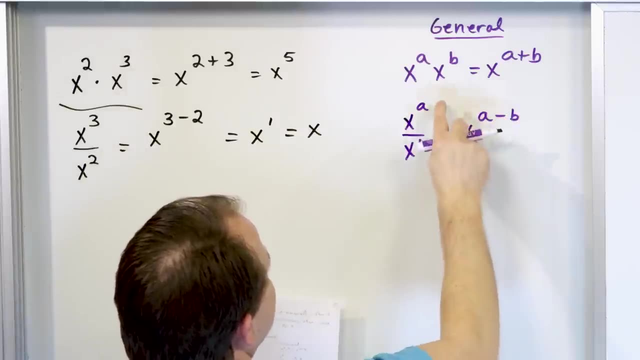 the numerical examples, and this one, again showing a little more formality, would be: x to the a divided by x to the b equals x to the a minus b. You're just subtracting the exponent's top minus bottom. Now just to take a little bit of aside The reason this actually 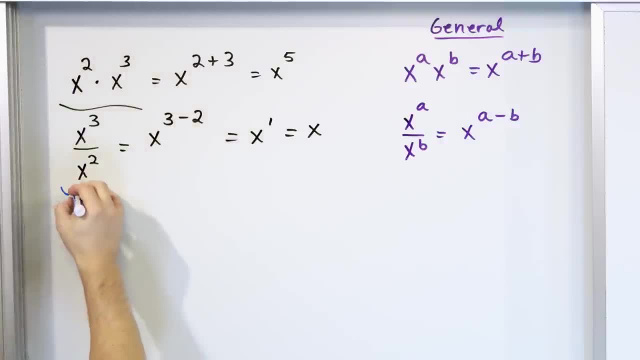 The reason I'm going to go into this- because we'll use it during our problems here- is the following: The numerator here is really written as x times x times x- There's three of them right- And the denominator is x times x. 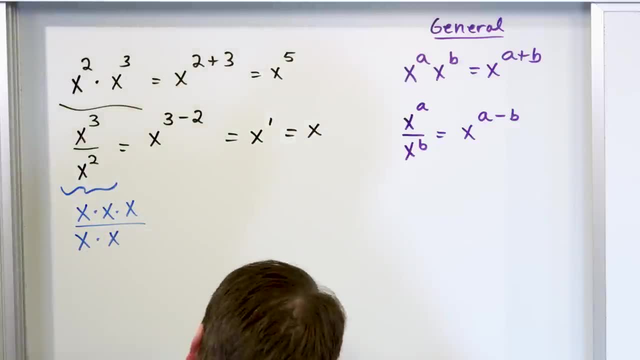 There's two of them. So since you have a lot of multiplication going on in the top and the bottom with the same variable, you can cancel terms. We have an x common to this x, so they divide away. We say things cancel in algebra when they're on top and bottom. 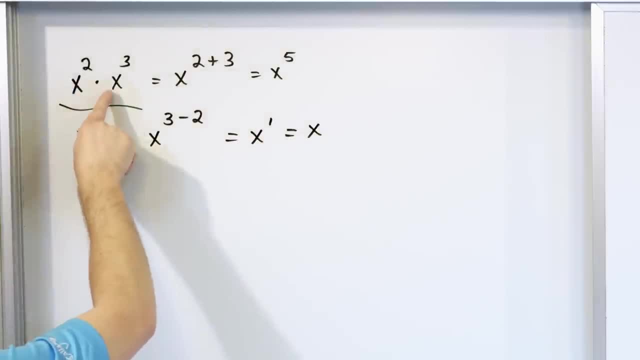 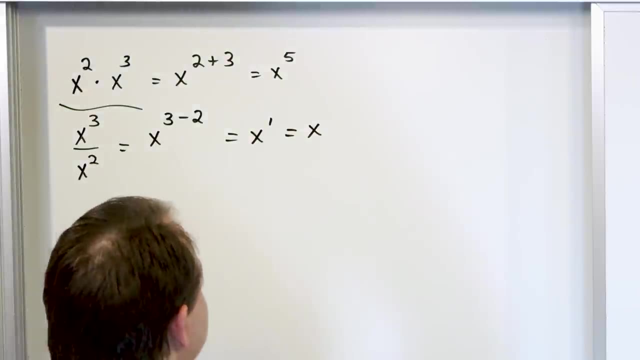 the symmetry here, once you get it all in one place, When you have the same base, different exponents, you multiply, you just add the exponents. When you divide, you subtract the exponents. Now, in general terms over here, I'll put another column here, general, And this is: 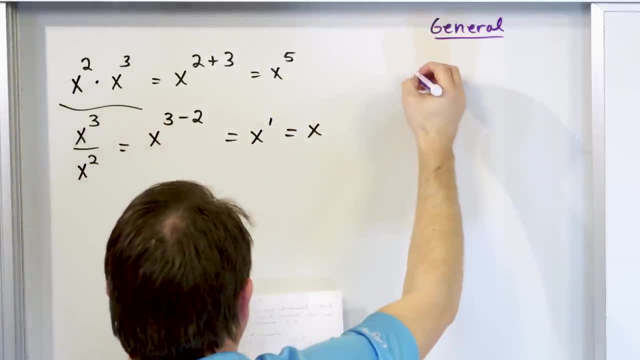 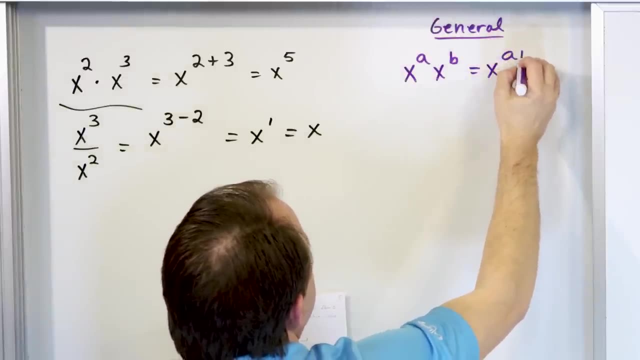 what you might see in a textbook. So for this first rule, what you might see in a textbook would look a little more formal. It might say: x to the a times, x to the power of b equals x to the a plus b. All this means is we add the exponents, just like I'm showing you with. 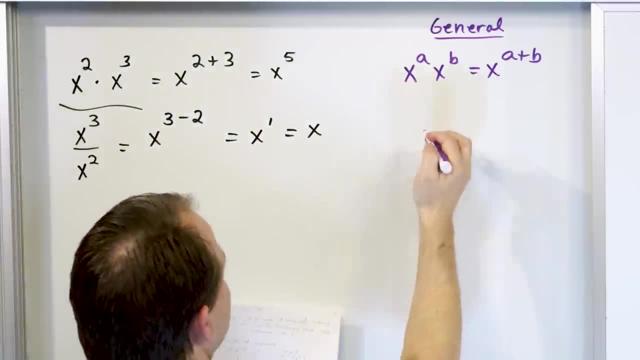 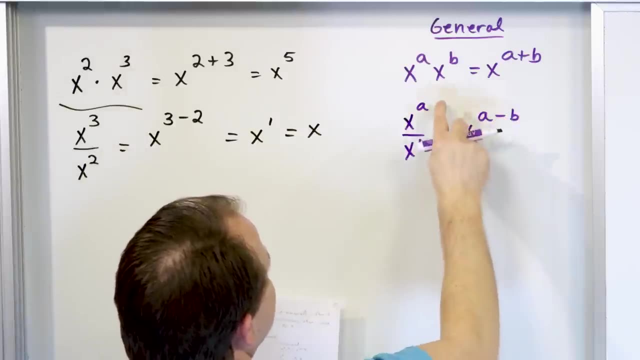 the numerical examples, And this one, again showing a little more formality, would be: x to the a divided by x to the b equals x to the a minus b. You're just subtracting the exponent's top minus bottom. Now just to take a little bit of aside the reason. 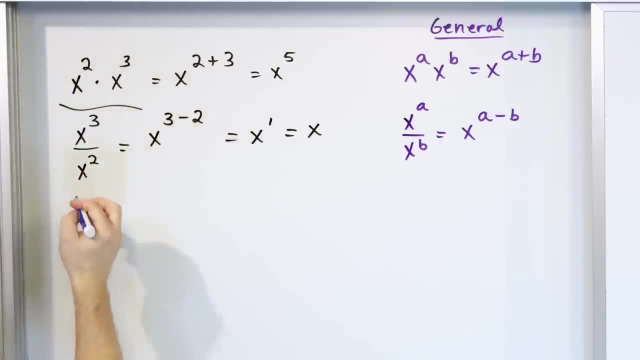 this actually works is because you can just take the top and the bottom exponents and divide them. The reason I'm going to go into this- because we'll use it during our problems here- is the following: The numerator here is really written as x times, x times. 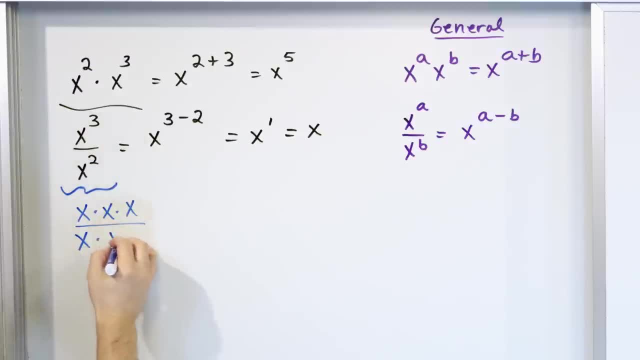 x. There's three of them right, And the denominator is x times x. There's two of them. So, since you have a lot of multiplication going on in the top and the bottom with the same variable, you can cancel terms. We have an x common to this x, so they divide away, You know. 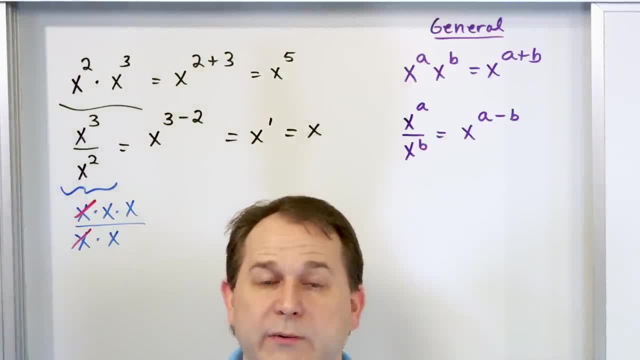 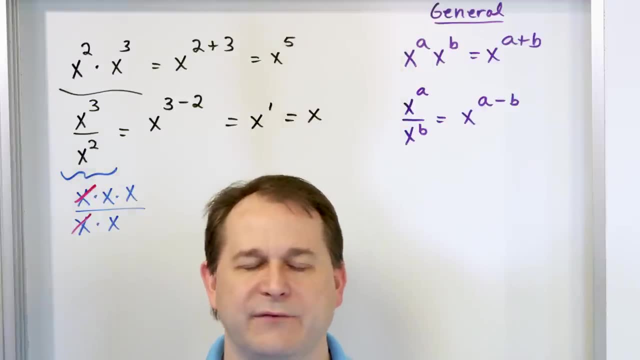 we say things cancel in algebra when they're on top and bottom, But really what's happening is you divide them away. x divided by x is 1.. Just like 2 divided by 2 is 1.. Or 17 divided by 17 is 1.. So this x divided by this x is: 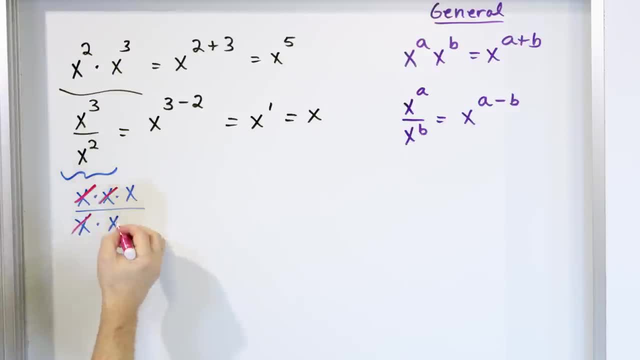 1, so they disappear, Or they don't disappear, they go to 1.. This one cancels with this one also. so all you have left is that x. So notice that what's really happening, no matter how you represent it. if you think of it as multiplication with canceling, you get an answer. If you 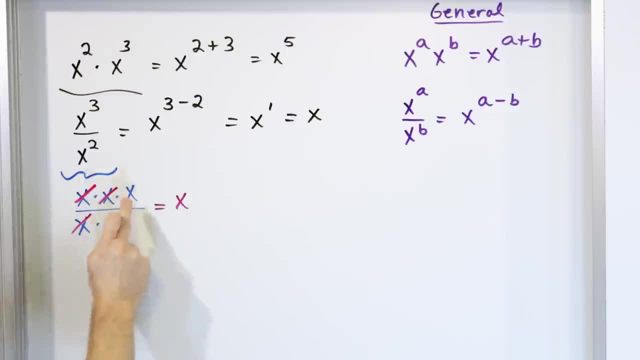 think of it as taking the top minus the bottom, which is really what you're doing. you're taking the top minus the bottom to give you what's left over. either way works And we will use both ways of thinking about it. We'll talk about these as we do our problems, But essentially you subtract the exponents. 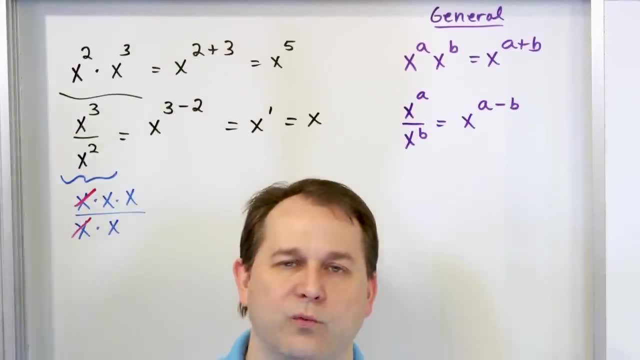 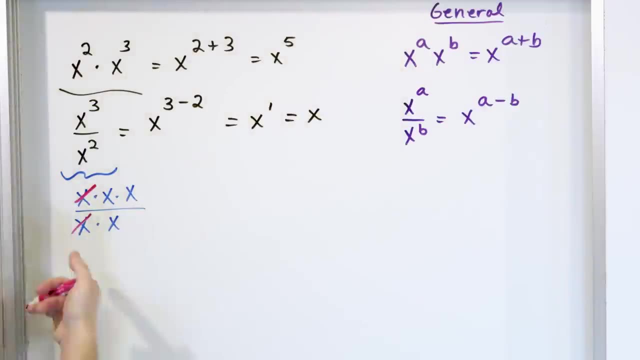 But really what's happening is you divide them away. x divided by x is 1,, just like 2 divided by 2 is 1, or 17 divided by 17 is 1.. So this x divided by this x is 1,. so they disappear. 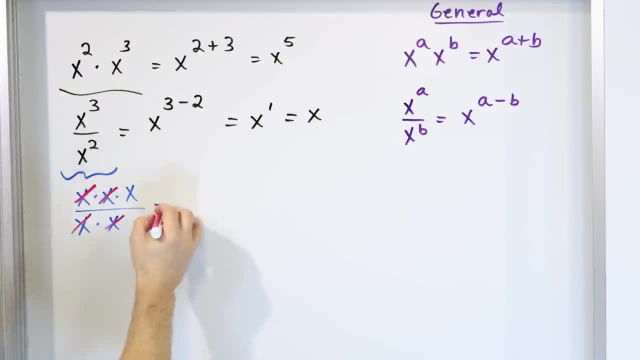 Or they don't disappear, they go to 1.. This one cancels with this one also. so all you have left is that x. So notice that what's really happening, no matter how you represent it. if you think of it as multiplication with canceling, you get an answer. 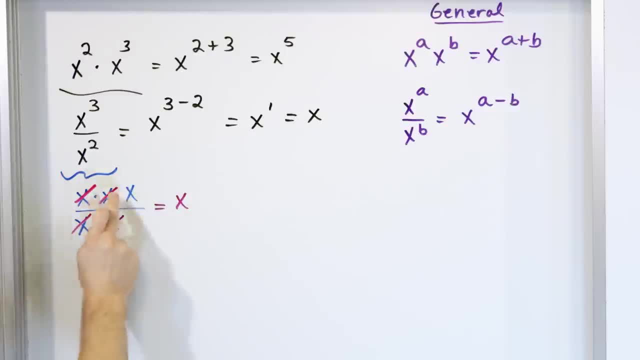 If you think of it as taking the top minus the bottom, which is really what you're doing. you're taking the top minus the bottom to give you what's left over. either way works, And we will use both ways of thinking about these. 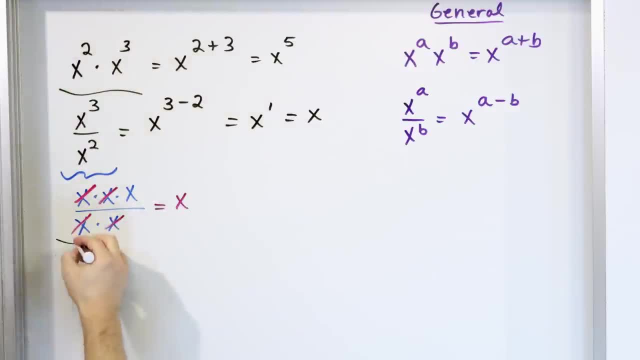 as we do our problems. But essentially you subtract the exponents. That's kind of the simplest way to think about it. Now, what if we have a product of two different variables, x times y, and we raise that to an exponent? 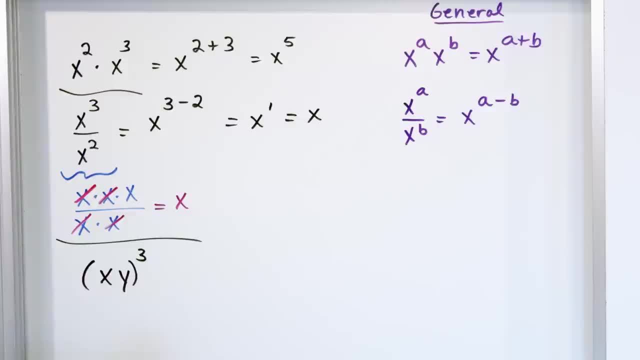 So what happens is this exponent gets applied to each term, almost like it's distributed in as follows: x to the third, y to the third. You take the exponent, you multiply it, or I shouldn't say you multiply it- you apply that exponent to every term in there. 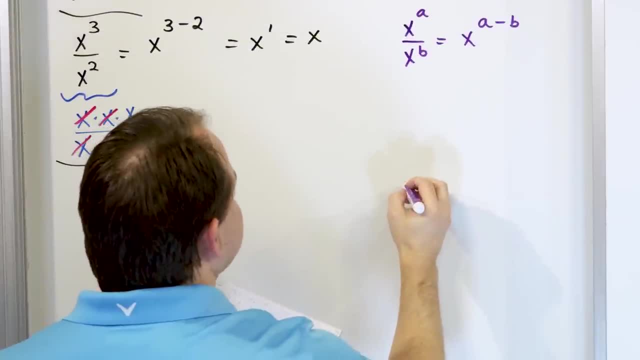 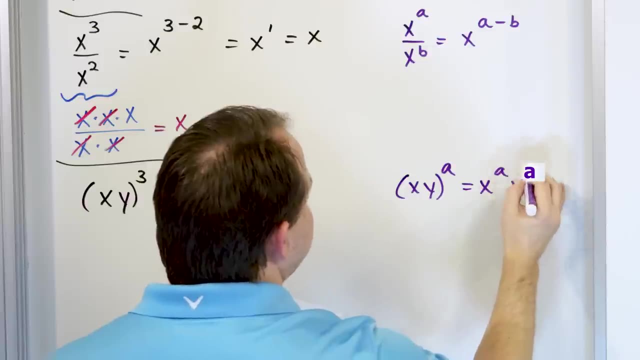 And then if you had to generalize this over here, the way you would see it on a textbook would be x times y to the a power, would be x to the a power times y to the b power, taking that exponent and applying it to everything inside, to every term inside. 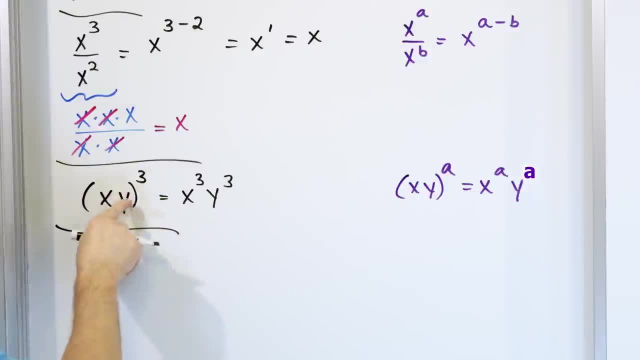 Now this is what happens when you're applying this to two different things: on the inside. What if you have an actual exponent like x squared, but then you raise that to another outside power? So what ends up happening? What's happening is you take these exponents. 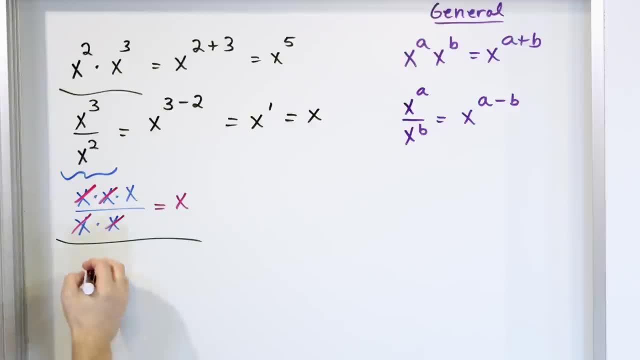 That's kind of the simplest way to think about it. Now, what if we have a product of two different variables, x times y, and we raise that to an exponent? So what happens is this exponent gets applied to each term, almost like it's distributed in as follows: x to 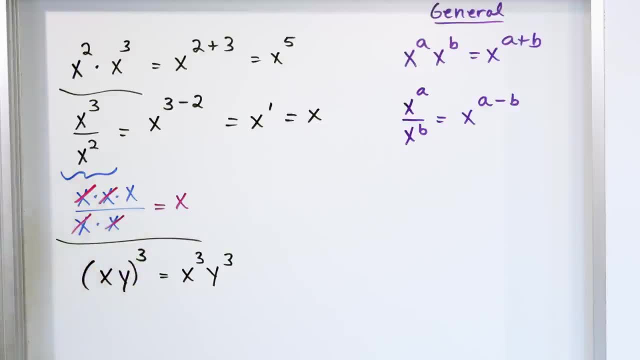 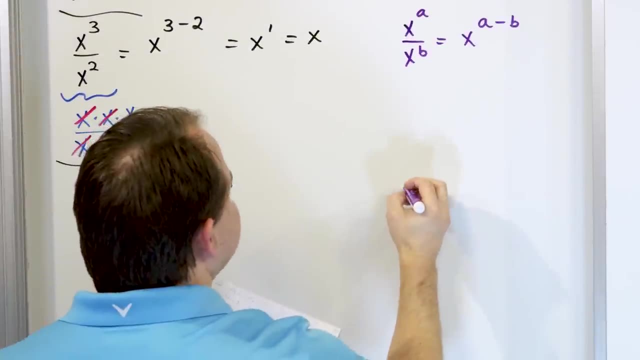 the third y to the third. You take the exponent and you multiply it, Or I shouldn't say you multiply it. You apply that exponent to every term in there. And then if you had to generalize this over here, The way you would see it on a textbook would be x times y to the. a power would be x to. 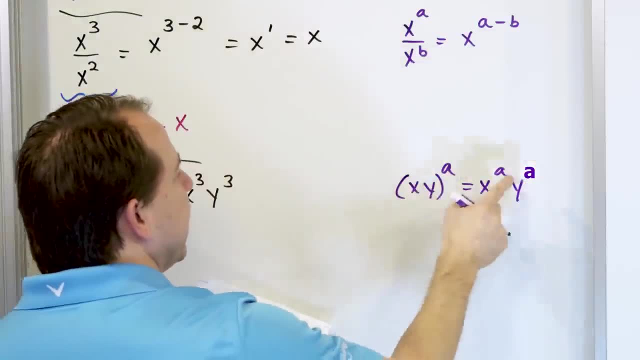 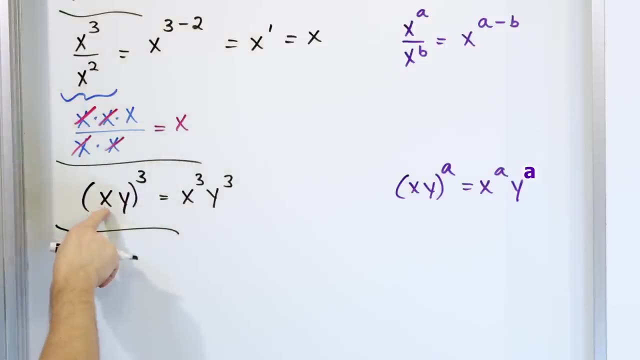 the a power times y to the b power, taking that exponent and applying it to everything inside, to every term inside. Now, this is what happens when you're applying this to two different things on the inside. What if you have an actual exponent like x squared, but then you raise that to another? 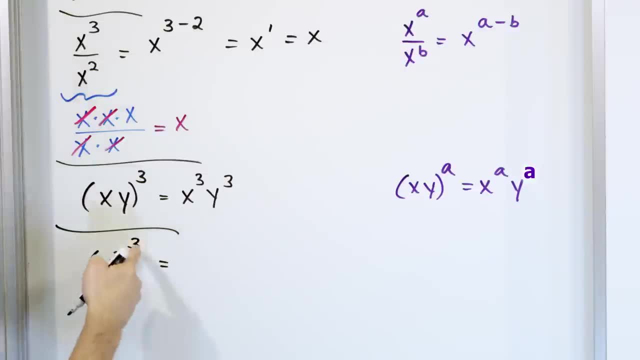 outside power. So what ends up happening is you take these exponents and you multiply them together. So what you're going to get is x to the two times three, which is x to the sixth power. So, exponent raised to an exponent, you get x to the sixth power, And 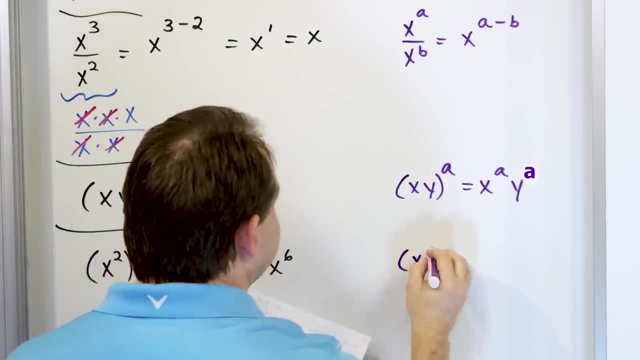 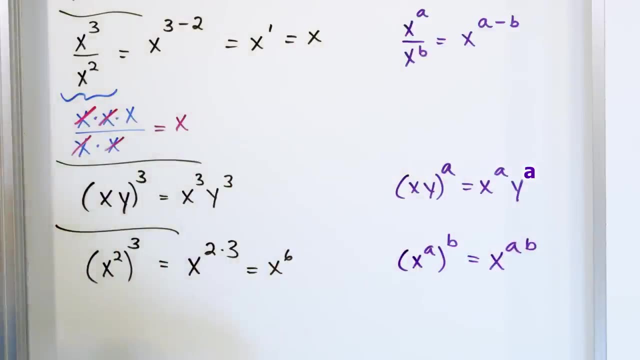 then if you were going to go over here and write that a little more formally, it would be x to the a. raised to the b, power is x to the a b. Now, all of these things I'm writing down on the board kind of quickly, And that's because 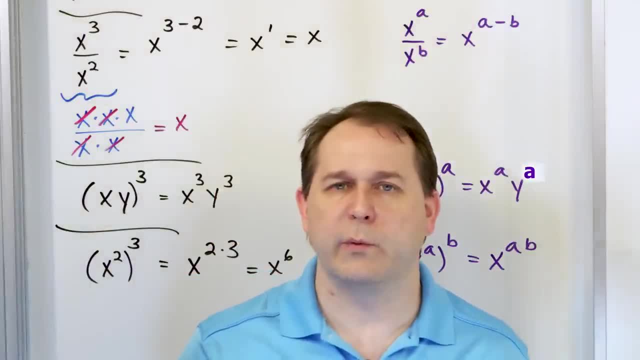 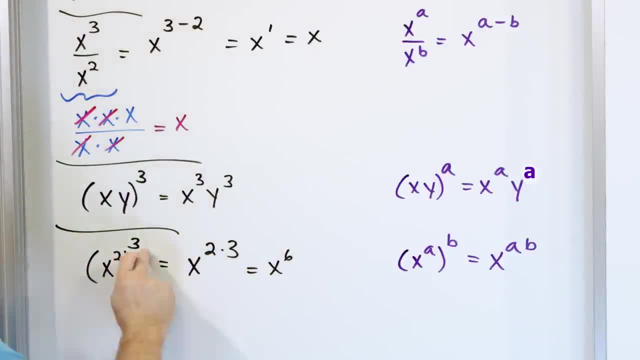 the exponents work and how it cancels that it comes out to always be multiplying these two exponents here. So if this all seems foreign, go back and watch the other lesson. I'm just trying to get them on the board so that we can kind of reference them during this lesson. 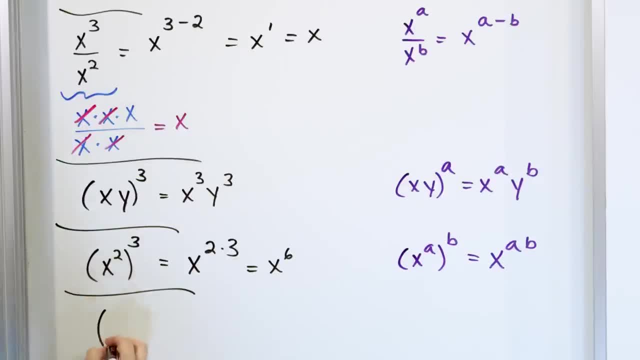 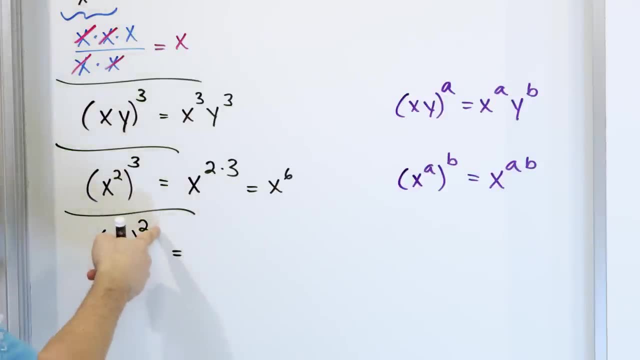 here. The last one I'm going to have is if we have a fraction x over y and we raise it to a power- in this case, let's say, to the second power- what happens is we take this exponent, just like we did here, and we apply it to everything inside. but we have to apply. 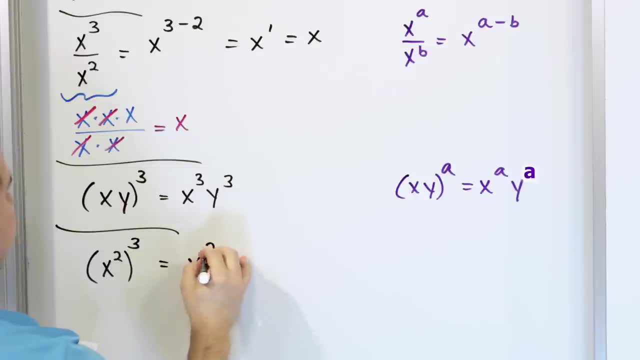 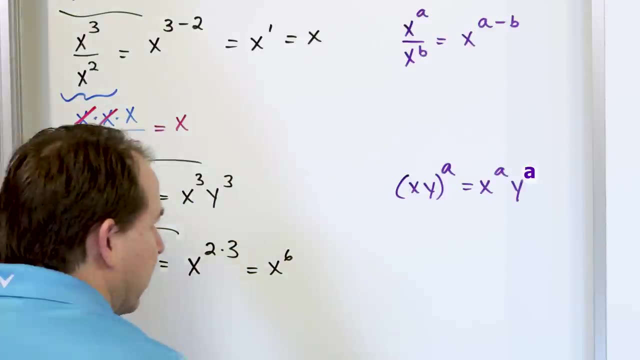 and you multiply them together. So what you're going to get is x to the 2 times 3, which is x to the 6th power. So, exponent raised to an exponent, you get x to the 6th power. And then, if you were going to go over here, 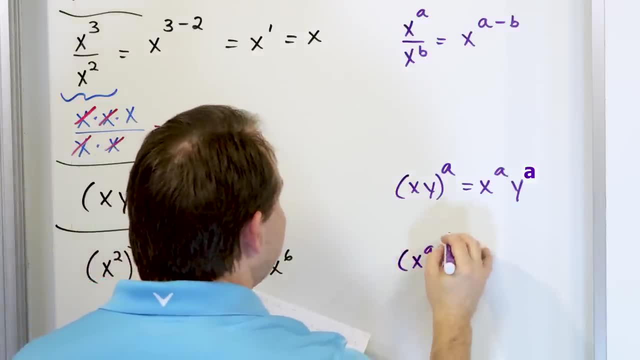 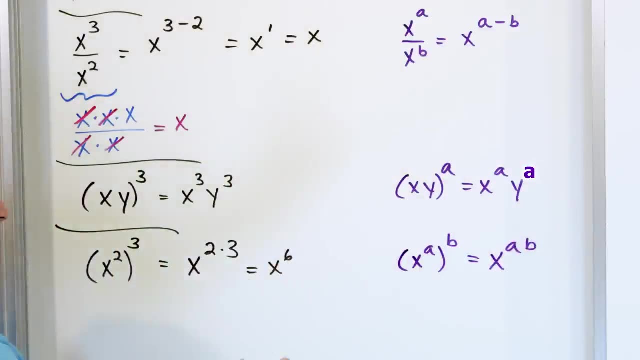 and write that a little more formally. it would be x to the a. raised to the b, power is x to the a b. Now, all of these things I'm writing down on the board kind of quickly and that's because I've had an entire lesson in exponent laws where we 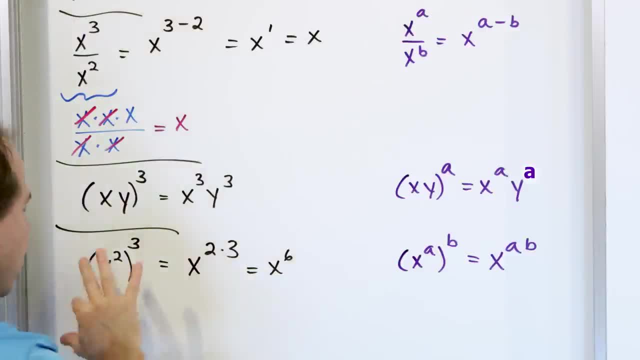 blew all of this stuff out And I can show you by writing down how the exponents work and how it cancels that it comes out to always be multiplying these two exponents here. So if this all seems foreign, go back and watch the other lesson. 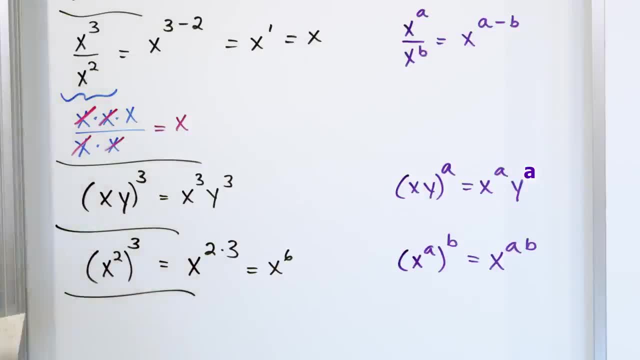 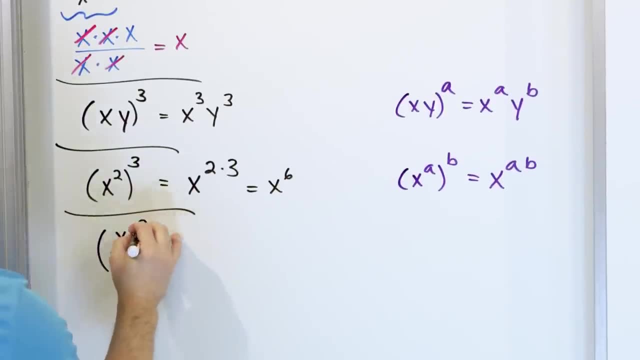 I'm just trying to get them on the board so that we can kind of reference them during this lesson here. The last one I'm going to have is if we have a fraction x over y and we raise it to a power, in this case, 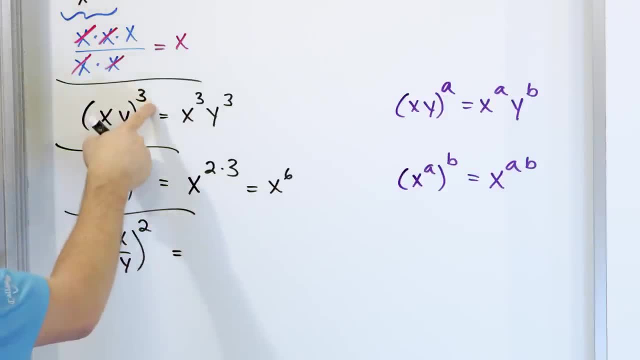 let's say to the second power. What happens is we take this exponent, just like we did here, and we apply it to everything inside, but we have to apply it to the top separately from the bottom, So the square gets applied to the top. 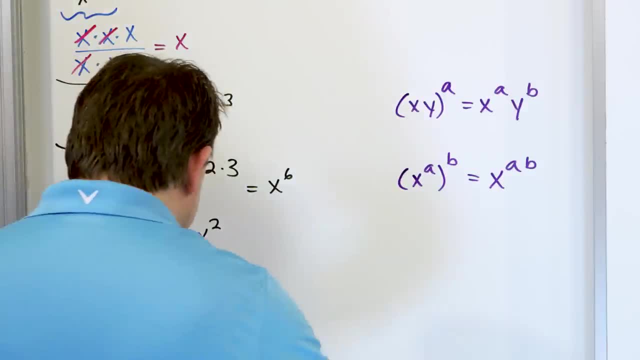 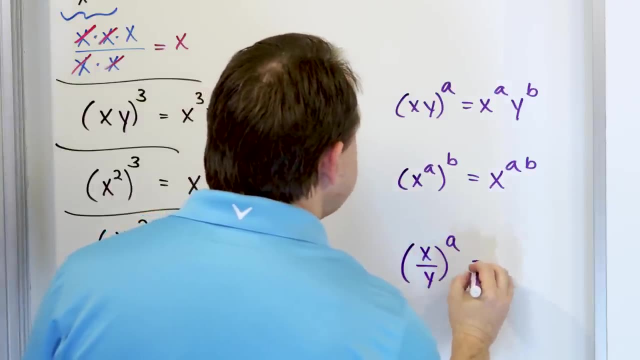 the square gets applied to the bottom, just like this. So if you wanted to write that down a little more mathematically, then you would say: x over y raised to the power of a, is x to the a over y to the a. 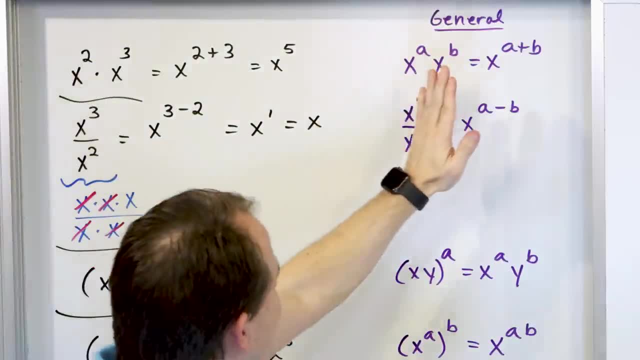 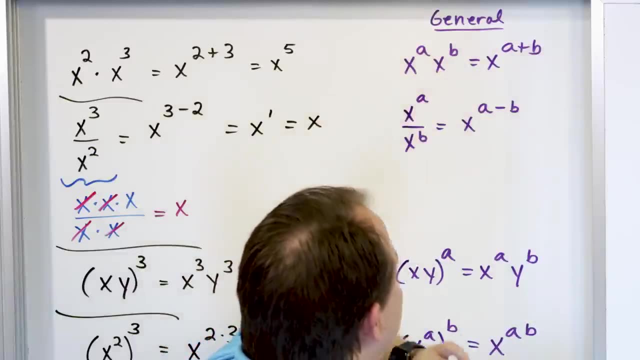 So again, just really quickly, you have two things multiplied. Let's go to the general column. Since we explained it with numbers, we'll go to the general column. You have two bases that are the same with different exponents. You just add the exponents if they're multiplied together. 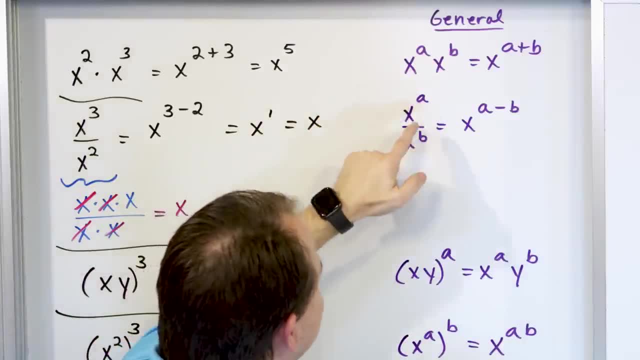 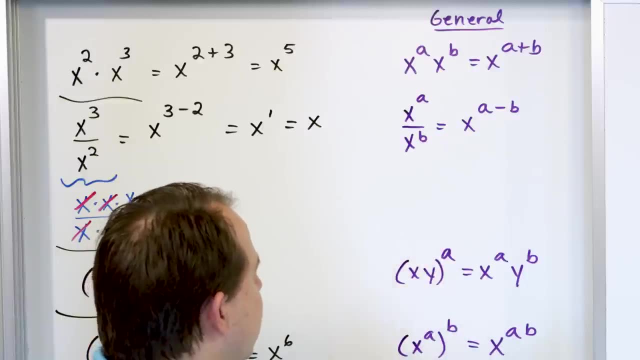 If those things are divided, then you just have the same base and you subtract top minus bottom to get the new exponent. If you have two things multiplied together with an exponent on the outside, you kind of distribute this And actually I have a typo here. 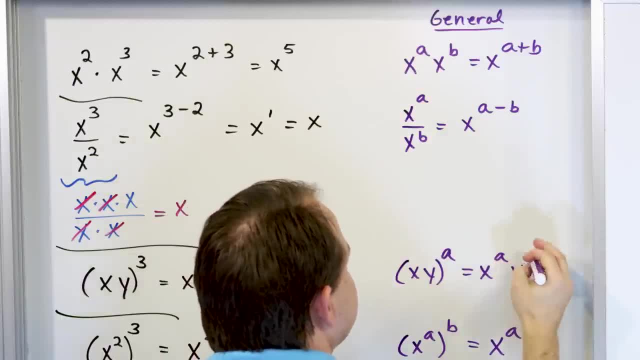 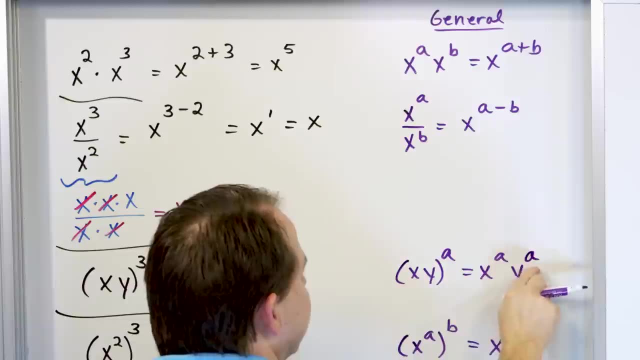 This is going to be x to the a, xy to the a as well. Sorry about that. You take this a and apply it to the x. You take the a and you apply it to the y. You get x to the a, y to the a. 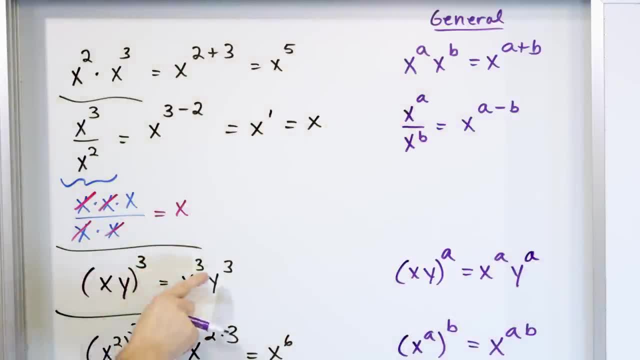 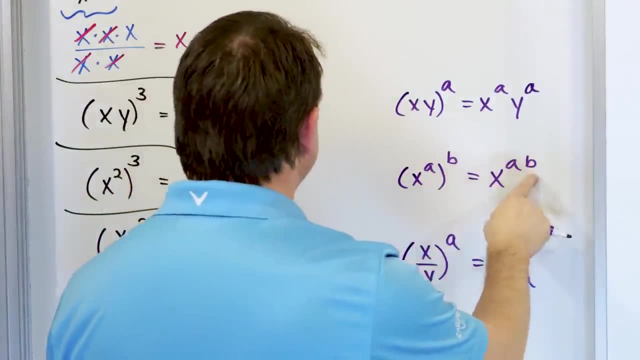 So that would be the general term, just the way we have it. here is exactly the 3 going in there. Sorry about the typo. And then for this one, when we have a power raised to a power, we just multiply the two things, just like we did the 2 times 3. 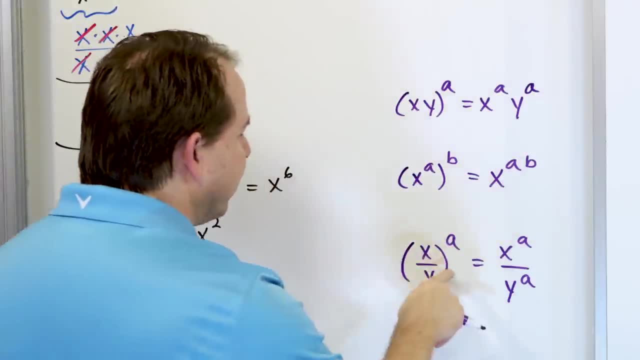 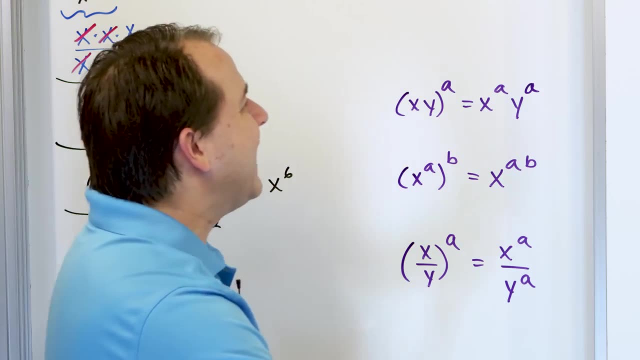 giving us the 6.. And then, when we have an exponent applied to a fraction, we have to apply it to the top and to the bottom of the fraction. Now that we have all of these on the board, we want to jump right into the concept of simplifying. 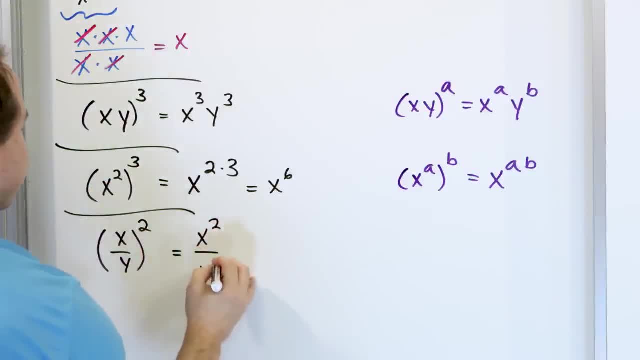 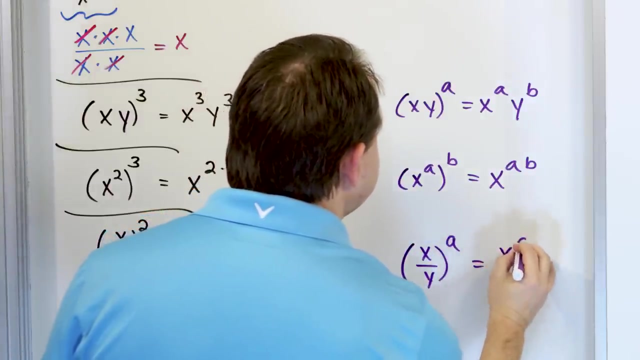 it to the top separately from the bottom. The square gets applied to the top, the square gets applied to the bottom, just like this. So if you wanted to write that down a little more mathematically, then you would say: x over y, raised to the power of a, is x to the a over y to the a. So again, just really quickly. 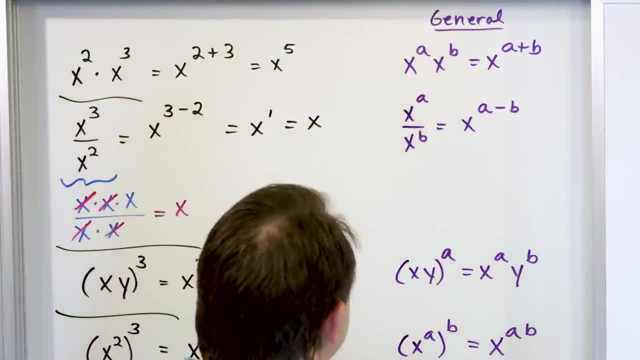 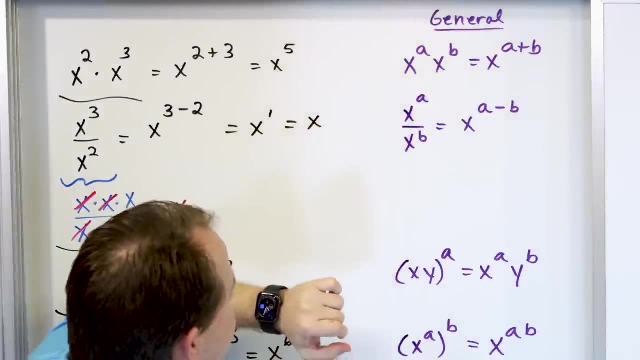 you have two things multiplied. Let's go to the general column. Since we explained it with numbers, we'll go to the general column. You have two bases that are the same with different exponents. You just add the exponents if they're multiplied together. 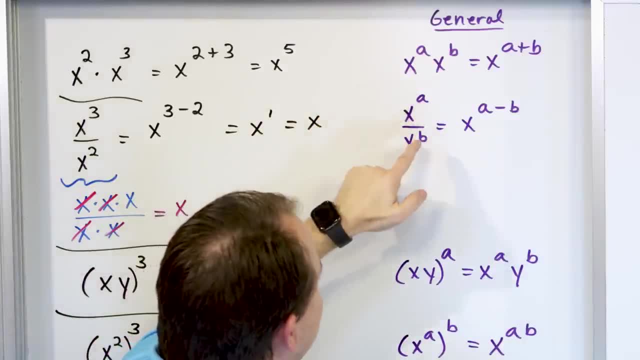 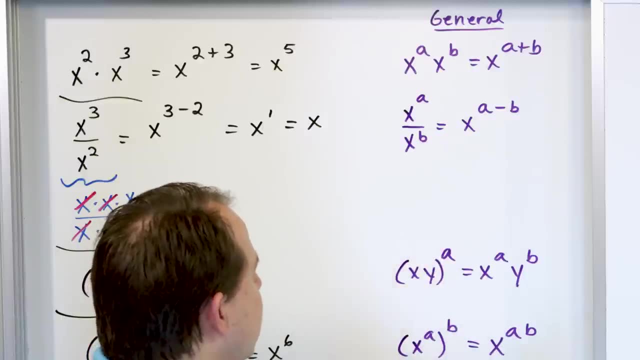 If those things are divided, then you just have the same base and you subtract top minus bottom to get the new exponent. If you have two things multiplied together with an exponent on the outside, you kind of distribute this and actually I have a typo here. This is going: 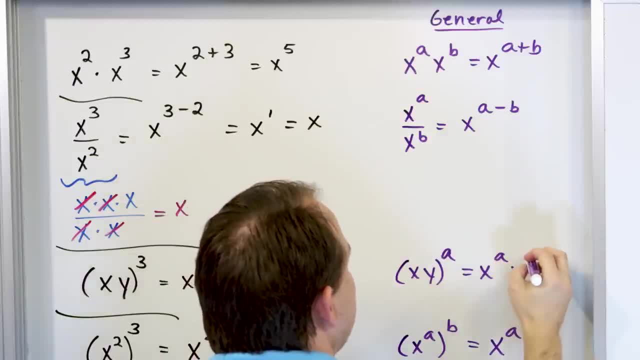 to be x, x to the a, x, y to the a as well. Sorry about that. You take this a and apply it to the x. you take the a and you apply it to the y. you get x to the a, y to the. 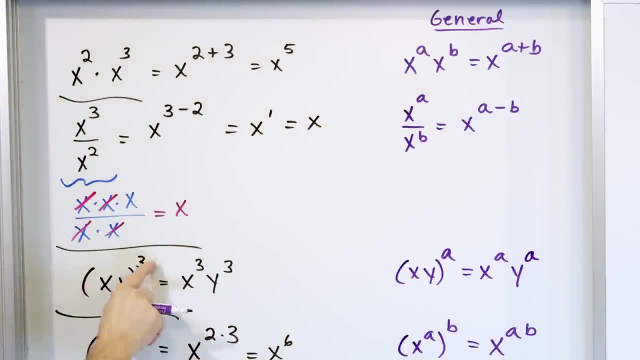 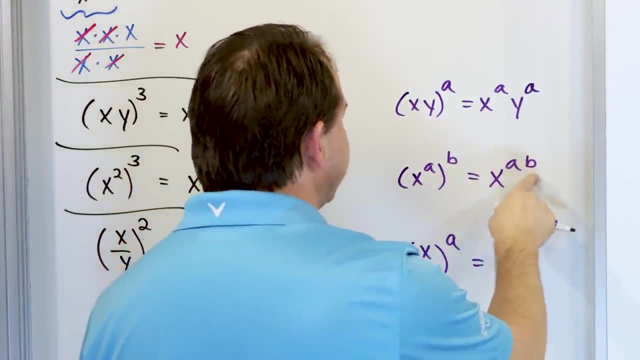 a. So that would be the general term, just the way we have it here. So exactly the three going in there. Sorry about the typo. And then for this one, when we have a power raised to a power, we just multiply the two. 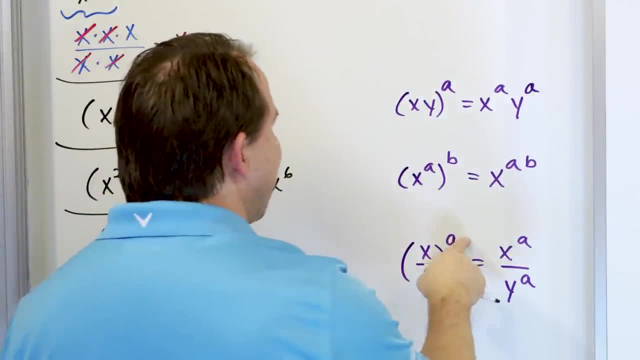 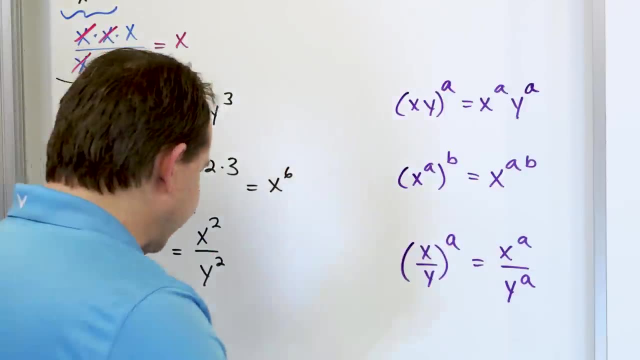 things just like we did: the two times three, giving us the six, And then, when we have an exponent applied to a fraction, we have to apply it to the top and to the bottom of the fraction. All right, now that we have all of these on the board, we want to jump right. 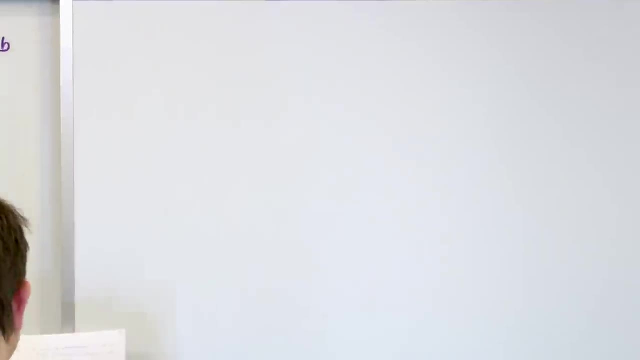 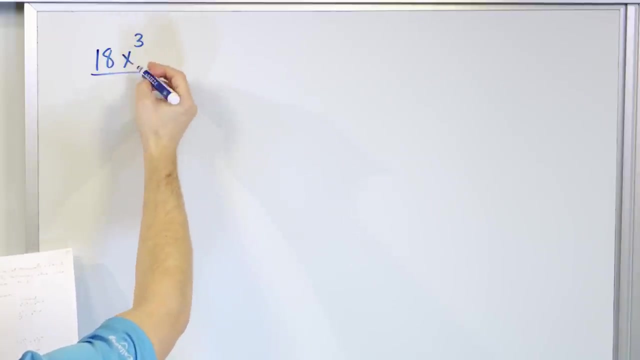 into the concept of simplifying these quotients of monomials. So let's say you had a problem that looked like this: Eighteen x to the third power divided by six x. All right, so what you have here. what I'm going to do is I could start scratching through. 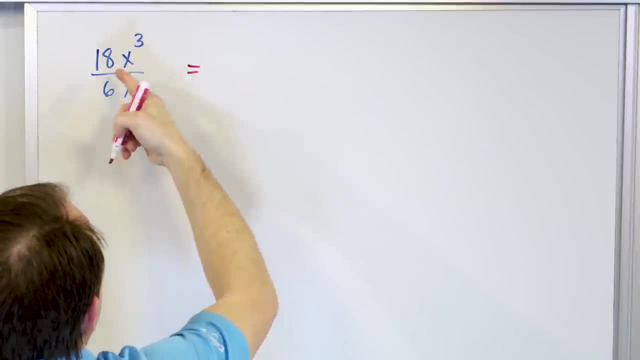 and all this stuff and marking it up. but what I want to do is write it over again so I don't kind of mess up the original thing that I wrote down: Eighteen x to the third over six x. So the first thing you do is you look at the numbers and you realize that six 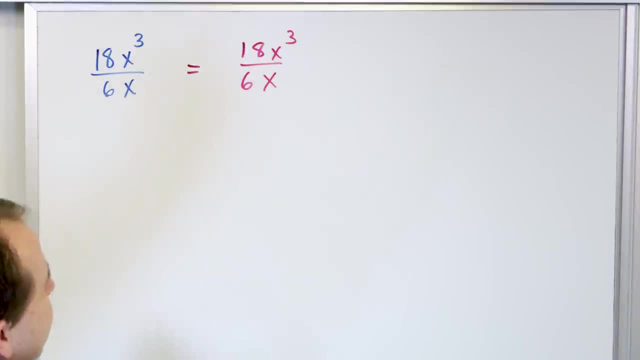 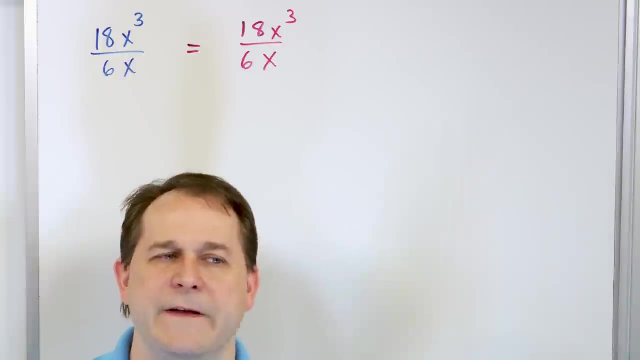 times three is eighteen and six times one is six. So another way of thinking about it is: any time you have numbers on the top and the bottom of a fraction, you always want to simplify that fraction. Just think about something like this: You're simplifying fractions. Any time you have a fraction, you always think about what. 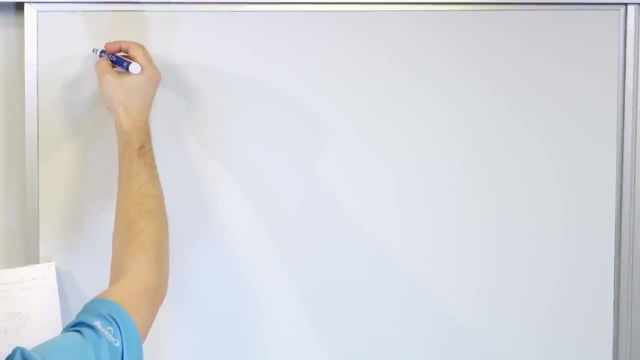 these quotients of monomials. So let's say you had a problem that looked like this: 18x to the third power divided by 6x. all right, So what you have here, what I'm going to do, 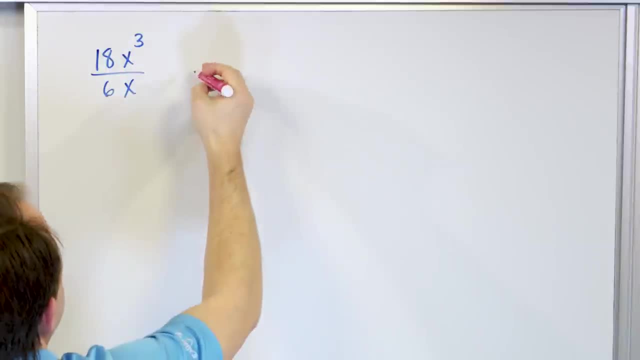 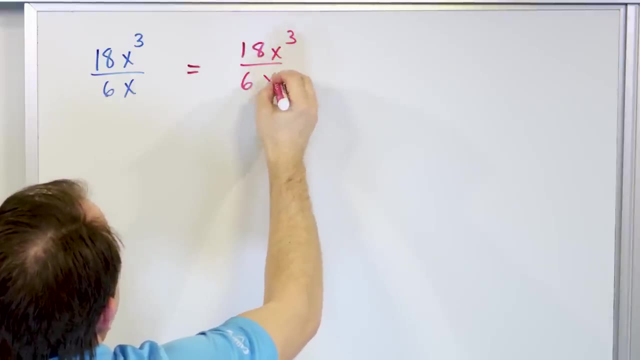 is. I could start scratching through and all this stuff and marking it up, But what I want to do is write it over again, so I don't kind of mess up. the original thing that I wrote down: 18x to the third over 6x. 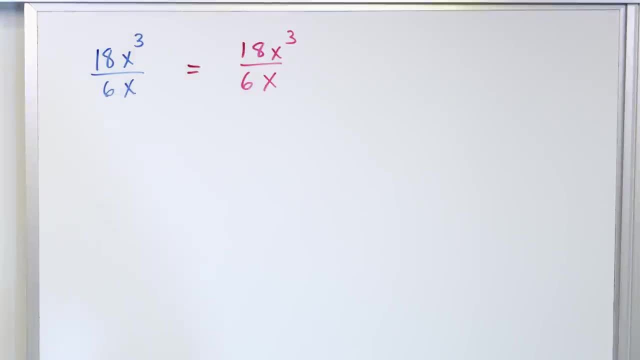 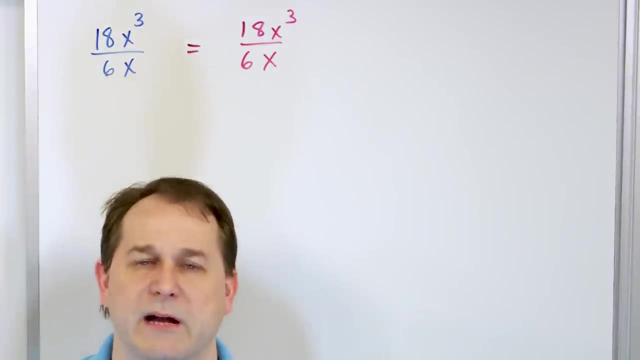 So the first thing you do is you look at the numbers and you realize that 6 times 3 is 18 and 6 times 1 is 6.. So another way of thinking about it is: anytime you have numbers on the top and the bottom, 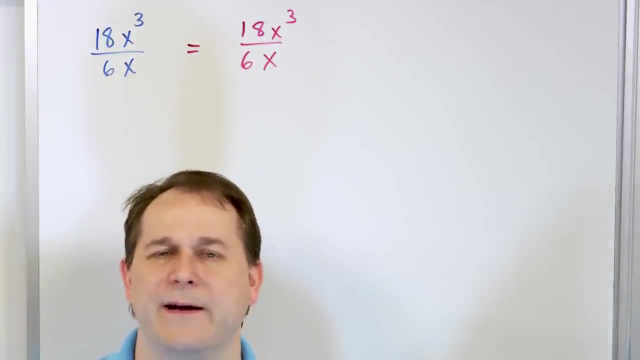 of a fraction, you always want to simplify that fraction. Just think about simplifying fractions. Anytime you have a fraction, you always think about what can I divide the top and the bottom by What is the largest thing I can divide the top? 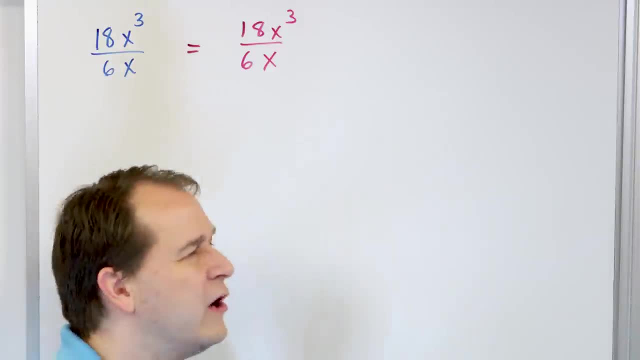 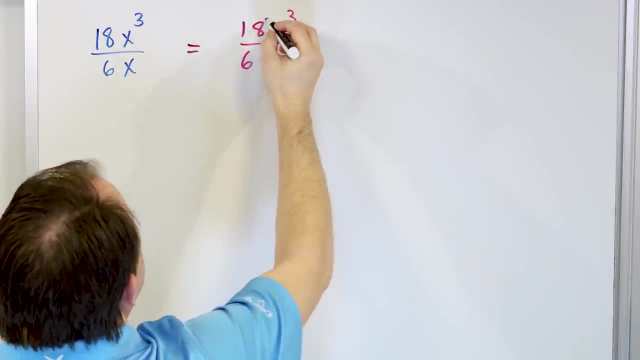 and the bottom by to simplify that fraction into lowest terms. So here I know I can divide the top by 6 and the bottom by 6, because they're both divisible by 6.. That's the biggest thing. So 18 divided by 6 is 3, so you strike it out. 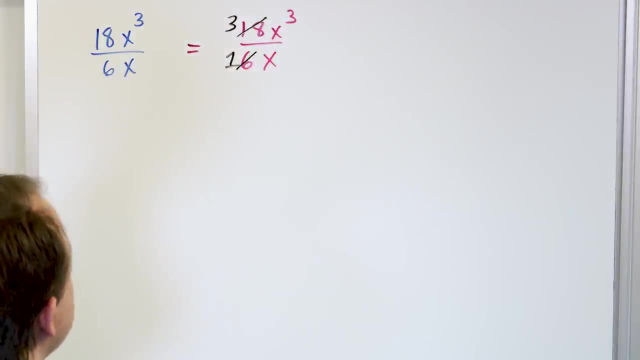 and put a 3, and 6 divided by 6 is 1.. So what's going to happen is when I rewrite the problem again, I'm just going to have a 3 and a 1 here instead of the 18 and the 6.. 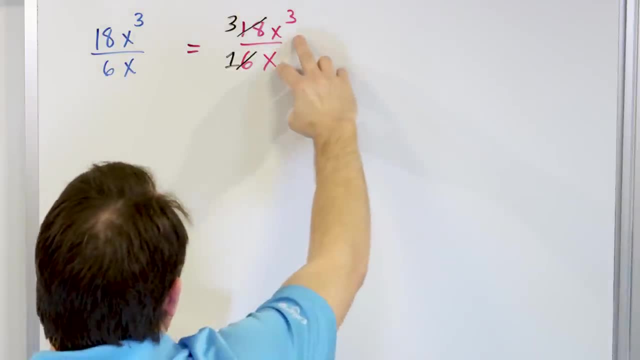 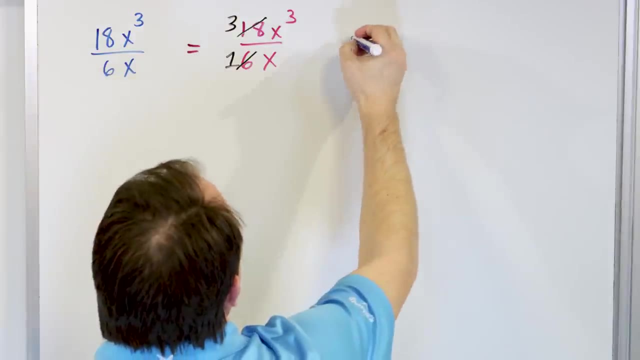 And then I look over here at the exponents and there's a couple of ways you can think about it. Let me go ahead and write the next part of the answer down, I guess. So what I'm going to have is I'm going to have a 3 here. 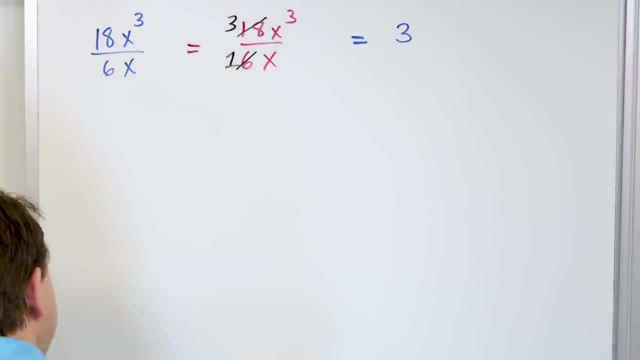 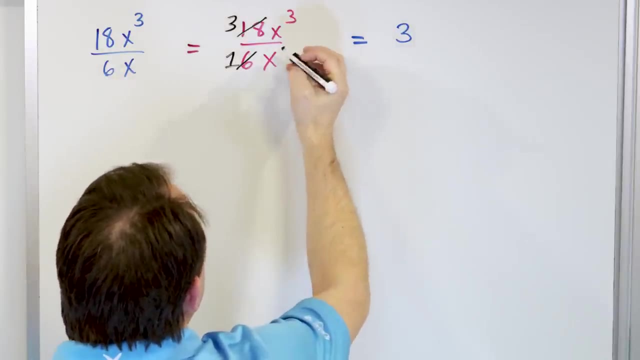 and then I'm going to have to figure out what to deal with here. Now, what you need to look at is commonality in the top and the bottom. I have three x's on the top- x times x, times x- and I have one on the bottom. 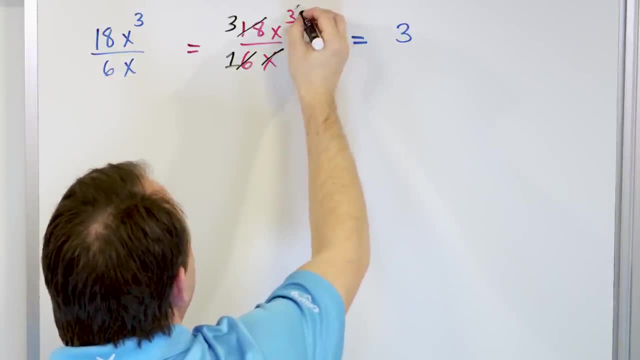 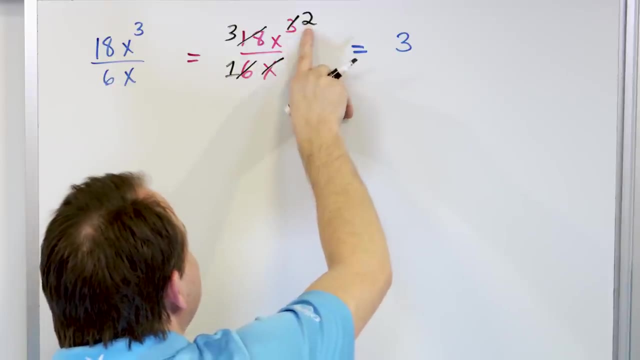 So this one x can cancel with one of them up here, but that'll leave two behind. So I strike through only the 3, rewriting it as a 2, letting me know that this single x canceled with only one of these, leaving me two behind. 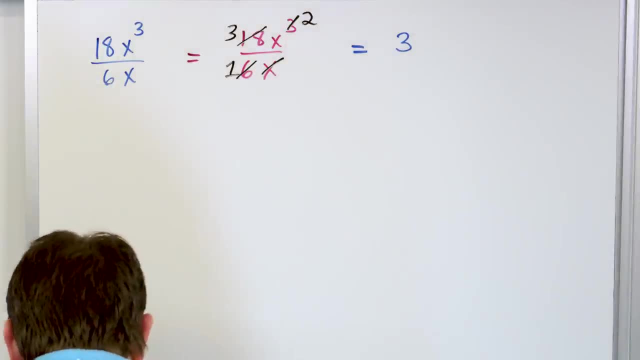 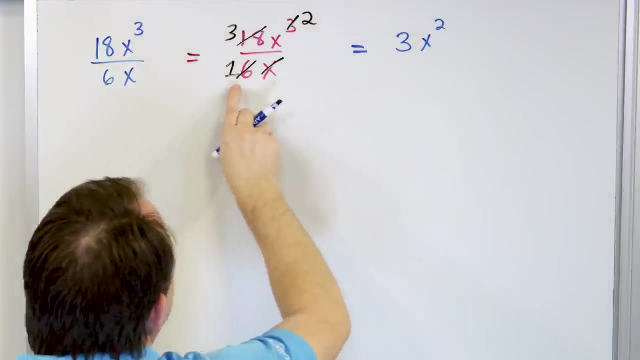 So then, when I rewrite the problem, I come over here and I say, well, all I have is a 3.. I still have an x here. and I have it to the second power On the bottom. I have a 1 here, but I struck through this x. 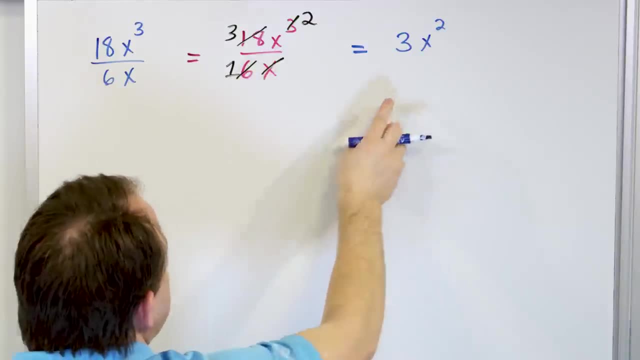 so there's really nothing else on the bottom, It's just a 1.. OK, And so I don't have to write a 1 here. So the answer I get is 3x squared. Now again, I told you, there's always. 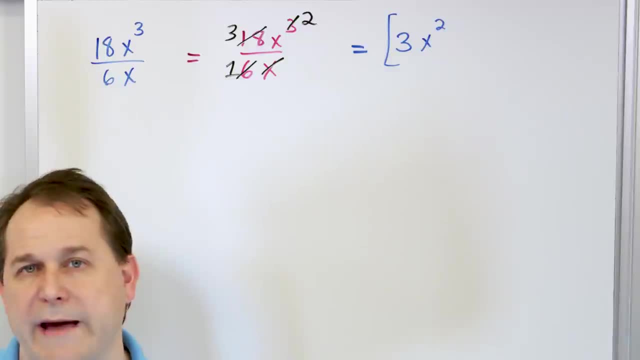 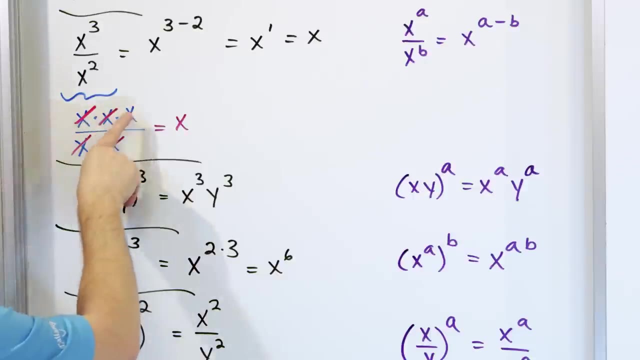 more than one way to solve problems in algebra, so you need to start thinking about different ways to think about it. So the first way- the way we did it here- was the idea that when you have exponent on the top and exponent on the bottom, what you're doing, 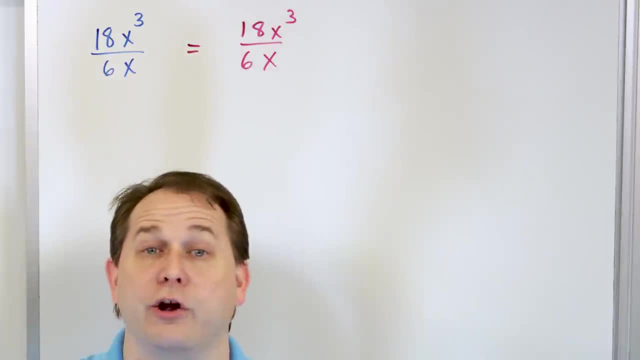 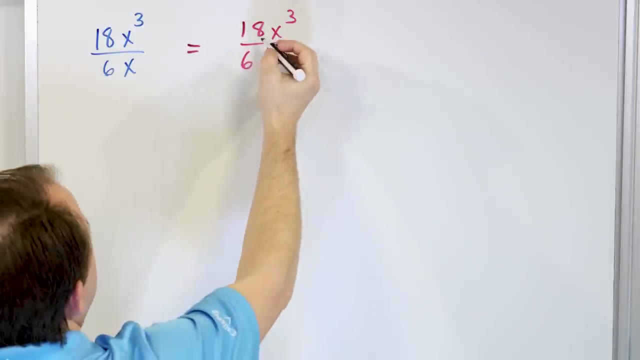 can I divide the top and the bottom by? What is the largest thing? I can divide the top and the bottom by to simplify that fraction into lowest terms. So here I know I can divide the top by six and the bottom by six, because they're both. 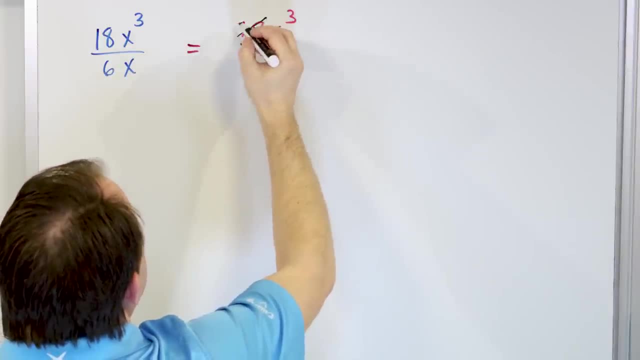 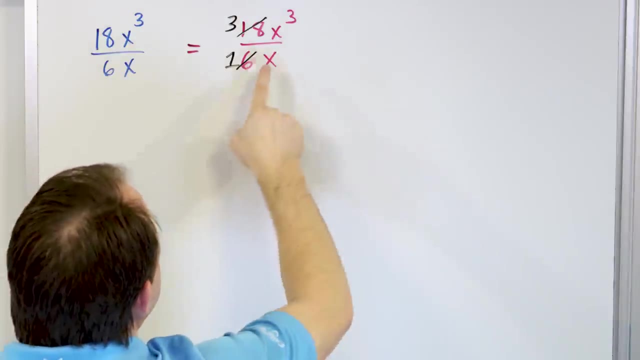 divisible by six. That's the biggest thing. So eighteen divided by six is three. so you strike it out and put a three and six divided by six is one. So what's going to happen is, when I rewrite the problem again, I'm just going to have a three and a one here instead. 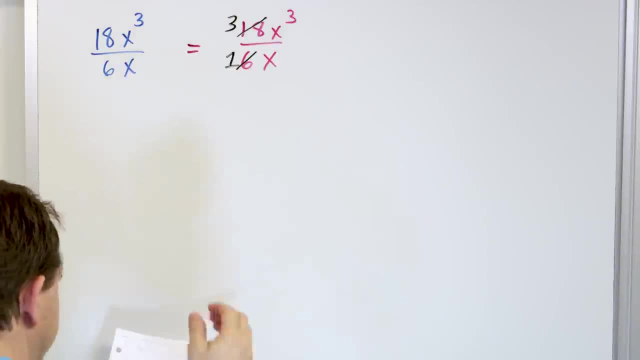 of the eighteen and the one, And then I look over here at the exponents and there's a couple of ways you can think about it. Let me go ahead and write the next part of the answer down, I guess. So what I'm going to have is I'm going to have a three here and then I'm going to have to figure. 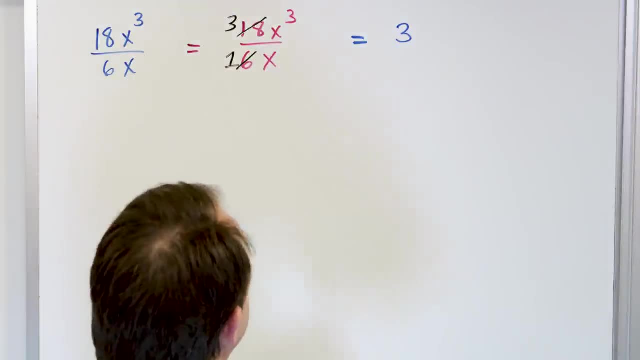 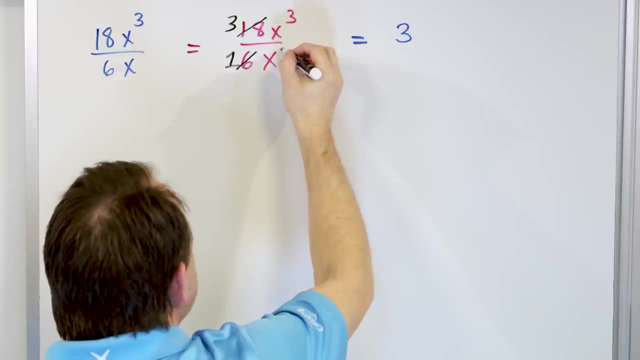 out what to deal with here. Now, what you need to look at is commonality in the top and the bottom. I have three x's on the top- x, times x, times x- and I have one on the bottom. So I only have one on the bottom, so this one x can cancel. 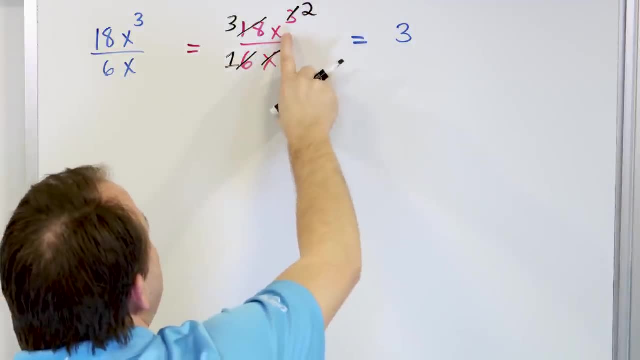 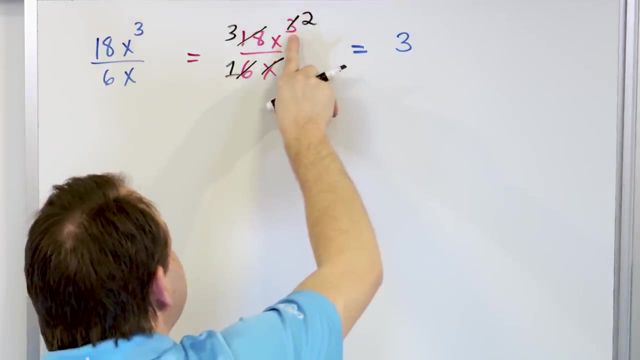 with one of them up here, but that'll leave two behind. So I strike through only the three, rewriting it as a two, letting me know that this single x cancelled with only one of these, leaving me two behind. So then, when I rewrite the problem, I come over here and I say: 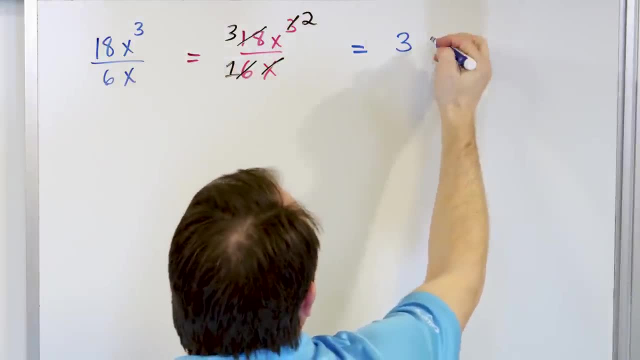 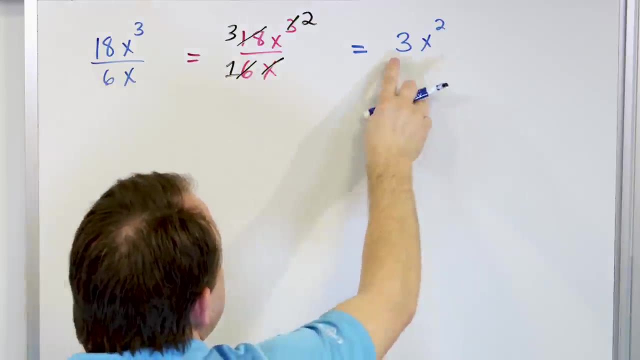 well, all I have is a three. I still have an x here and I have it to the second power On the bottom. I have a one here, but I struck through this x. so there's really nothing else on the bottom, it's just a one, and so I don't have to write a one here. So the answer. 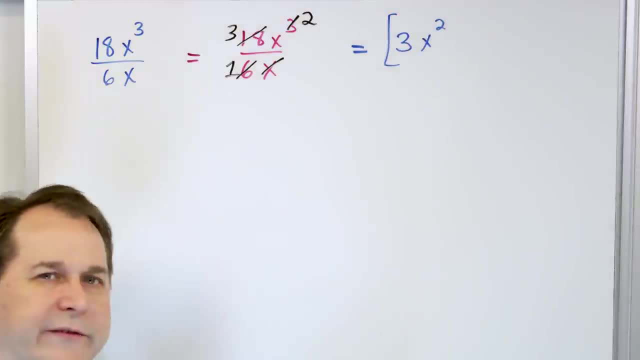 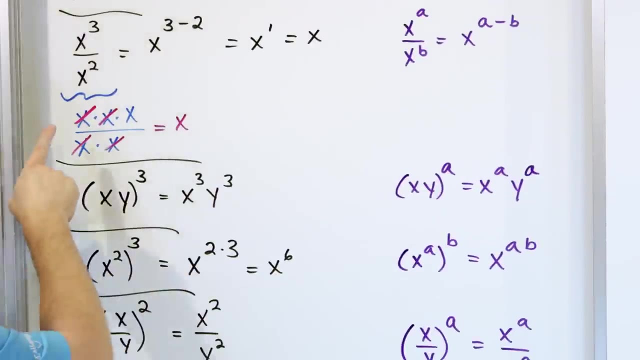 is three x squared. Now again, I told you there's always more than one way to solve problems in algebra, so you need to start thinking about different ways to think about it. So the first way, the way we did it here, was the idea that when you have exponent on 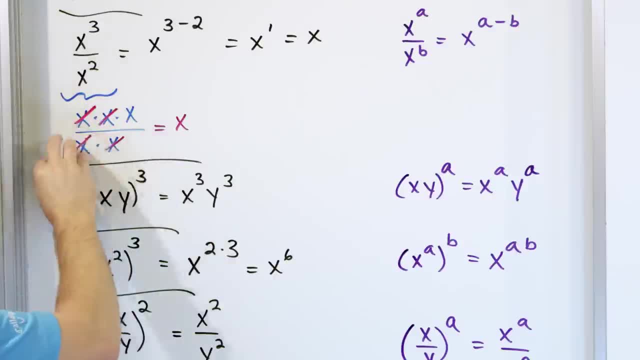 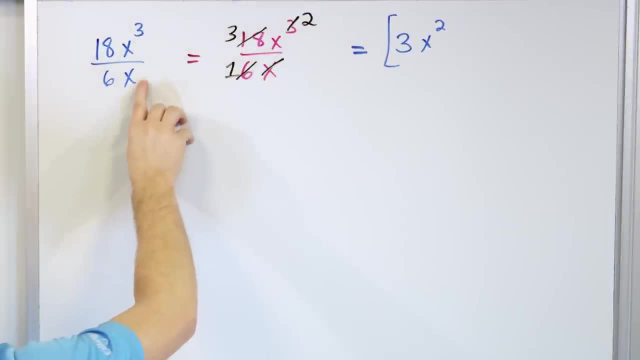 the top and exponent on the bottom. what you're doing is you're slicing through all of the commonality because they're dividing away. So in this case we had three x's on the top and we had one on the bottom, So we can only strike through the one on the bottom and 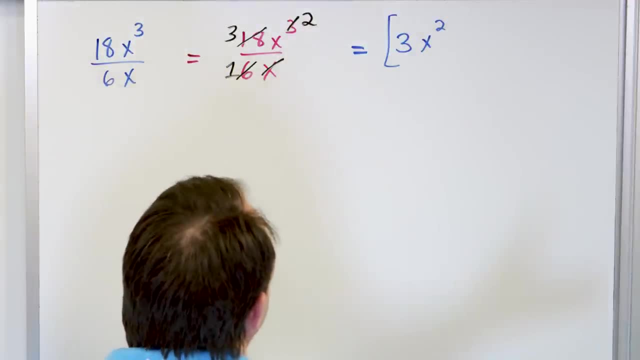 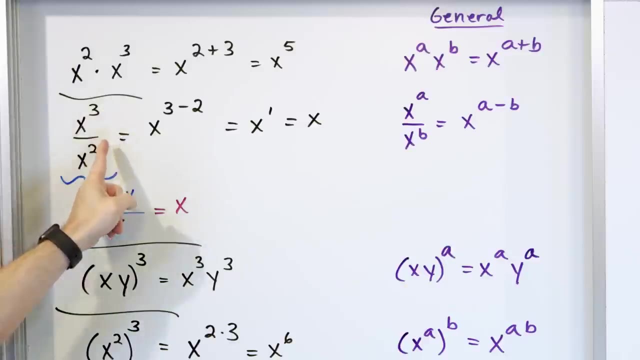 we only could strike through one on the top, leaving two behind. That's why we got a better answer. But notice, another way you can think about it is remember the exponent. law for division is we just subtract the exponent. So we have exactly the same concept over here. 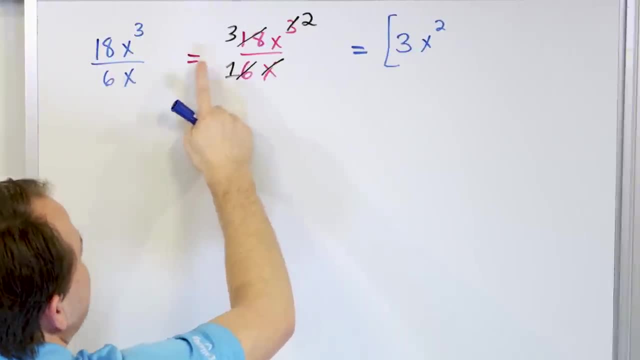 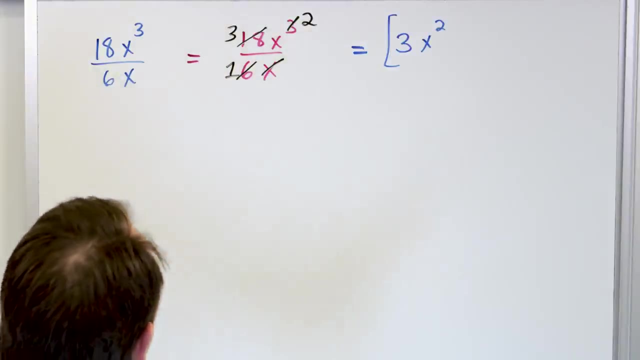 Three minus two is one. in this example, Three minus one means the exponent will be two, So there's really multiple ways to do it. I can strike through like this, which is what I typically do in my problems, or I can just look at it and say: well, the new exponent. 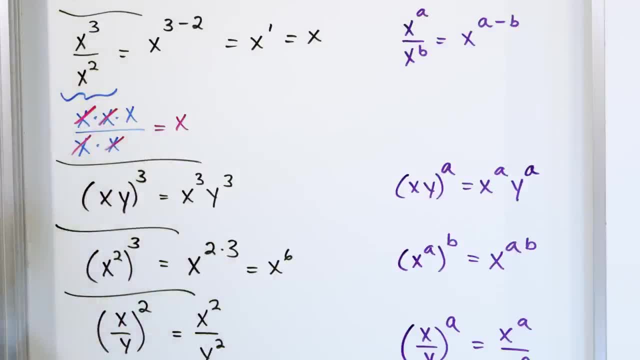 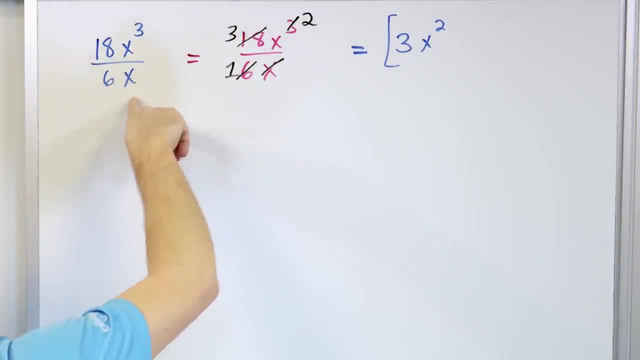 is you're slicing through all of the commonality because they're dividing away. So in this case we had three x's on the top and we had one on the bottom, So we can only strike through the one on the bottom and we only could strike through one on the top. 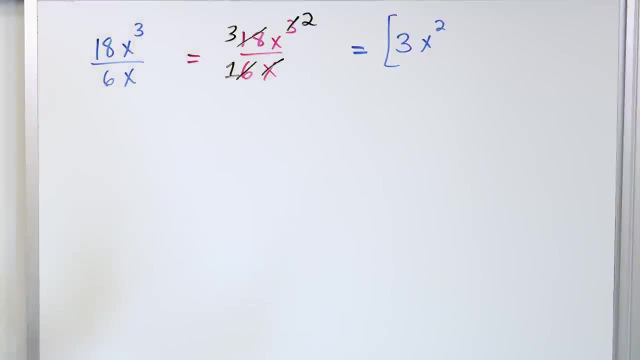 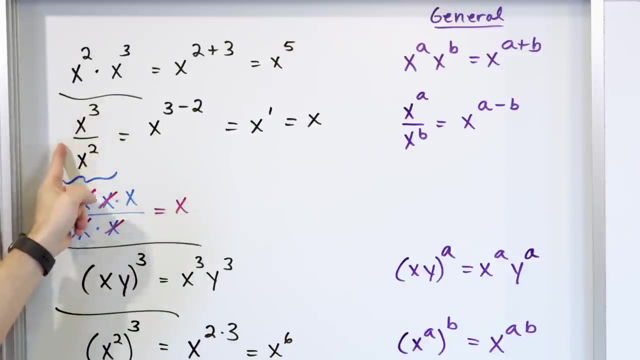 leaving two behind. That's why we got our answer. But notice, another way you can think about it is: remember the exponent. law for division is we just subtract the exponent. So we have exactly the same concept over here. 3 minus 2 is 1 in this example. 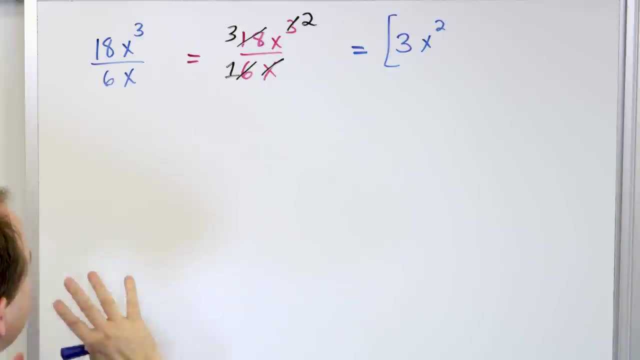 3 minus 1 means the exponent will be 2. So there's really multiple ways to do it. I can strike through like this, which is what I typically do in my problems, or I can just look at it and say: well, 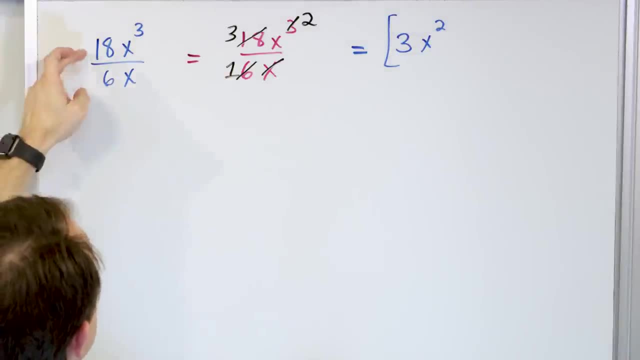 the new exponent has to be subtracted. 3 minus 1 is 2.. And then the 18 divided by 2.. OK, The 18 divided by the 6 gives you 3.. All right, So that's just the first problem. 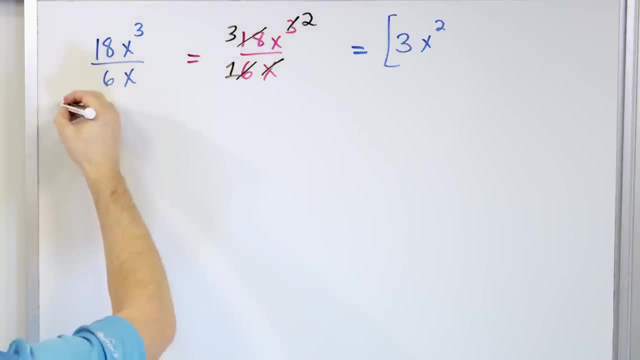 We're going to get to a lot more complicated things, But these are important concepts because soon we're going to have lots of variables and lots and lots of exponents to deal with. So what if we had, for the next problem, negative 12? 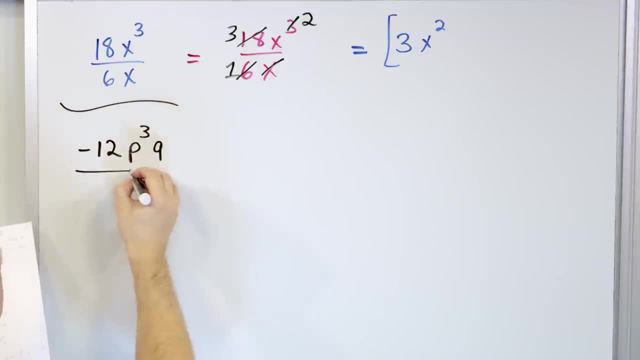 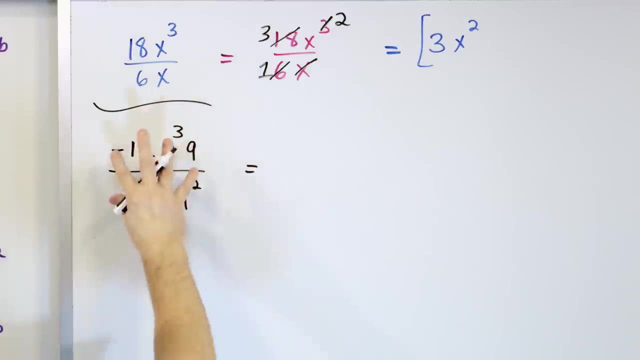 p to the third power times q, all divided by 4. p to the second power, q squared. And as I said, I don't want to mark up my original problem. I'm going to do a lot of rewriting in this lesson. You may or may not do that on your paper. 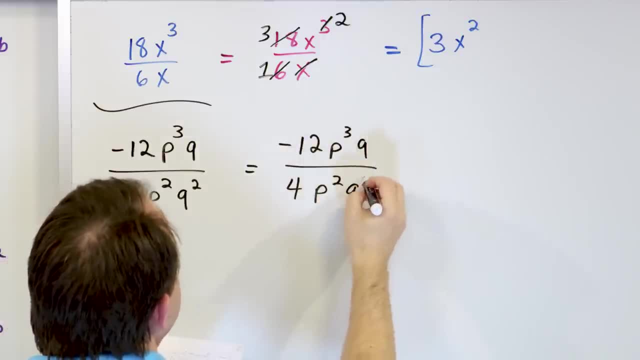 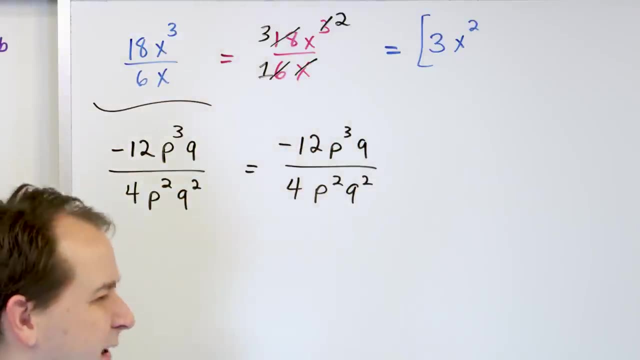 But I always write it down again, because here's the problem: If you start scratching up the thing you write down, then it's going to look like this: It's going to be marked up and you'll never be able to see what you started with. 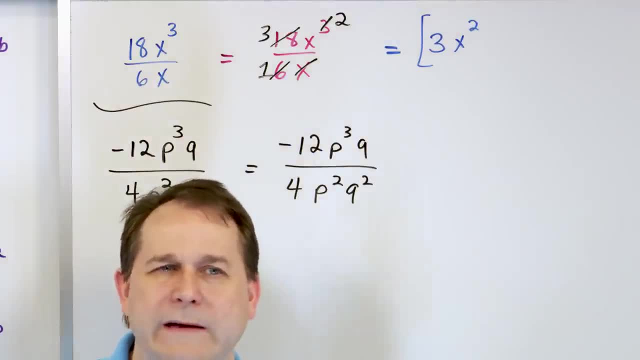 Besides, I'm using colored markers, But when you're using a pencil there's no color there, So it's hard to see what you wrote down initially. So write it down again before you start messing around with it. So we talk about the numbers first. 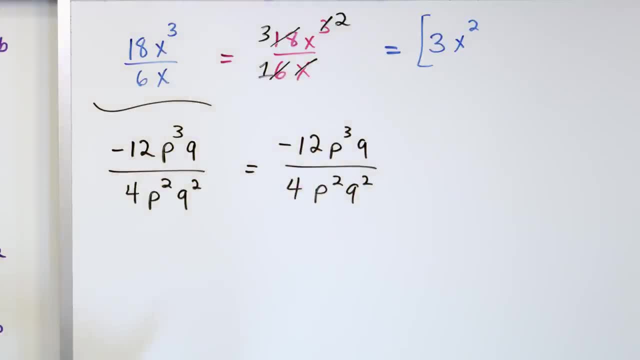 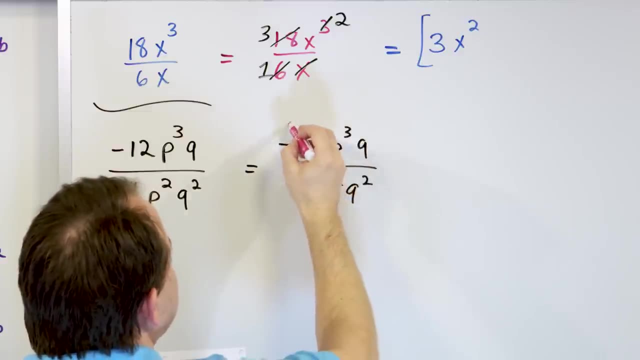 I know you all know that 12 divided by 4 is 3.. But I want you to think about: We're dividing the top and the bottom by some common number, So we'll divide. the 12 divided by 4 is going to give me 3.. 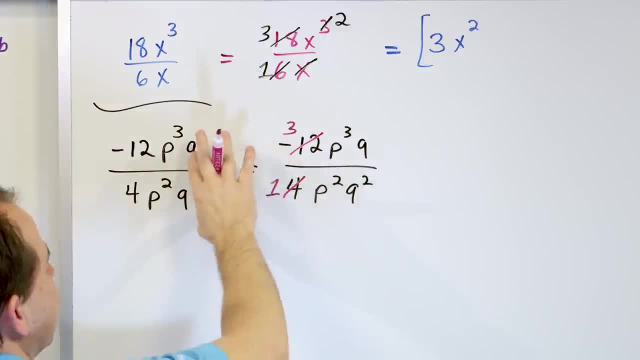 And the 4 divided by 4 is going to give me 1.. The negative doesn't divide away with anything. It's still there, So we still have a negative, But this 12 becomes a 3, and the 4 becomes a 1.. 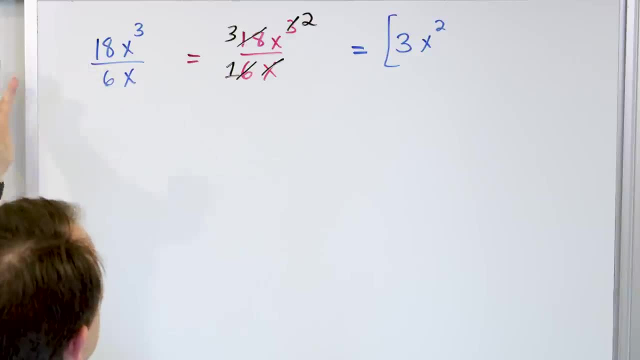 has to be subtracted. Three minus one is two, And then the 18 divided by the six gives you three. So that's just the first problem. We're going to get to a lot more complicated things, but these are important concepts because soon we're going to have lots of variables and 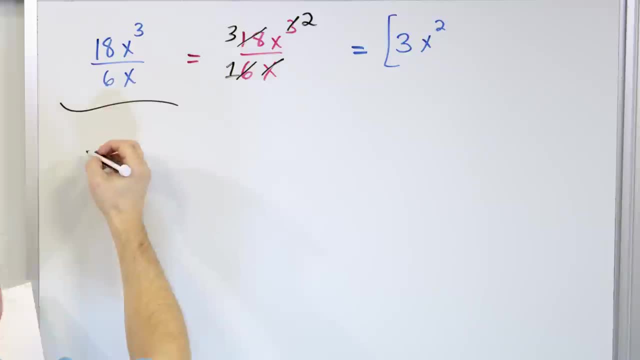 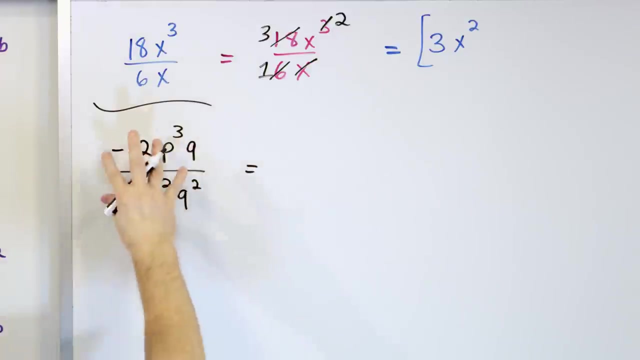 lots and lots of exponents to deal with. So what if we had, for the next problem, negative 12 p to the third power, times q all divided by four? p to the second power, q squared. And as I said, I don't want to mark up my original. 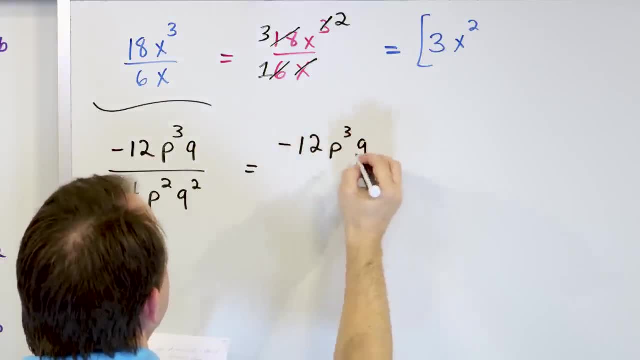 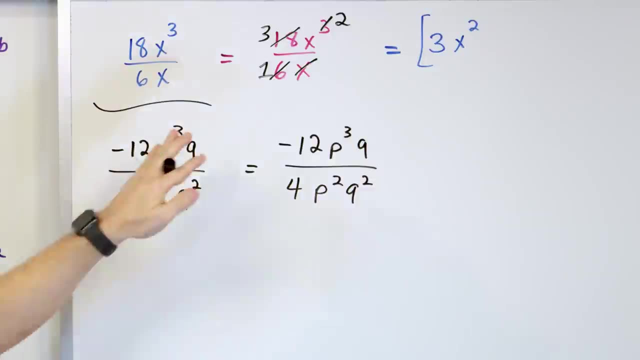 problem. so I'm going to do a lot of rewriting in this lesson. You may or may not do that on your paper, But I always write it down again. because here's the problem: If you start scratching up the thing you write down, then it's going to be. it's going to look like this. It's going to: 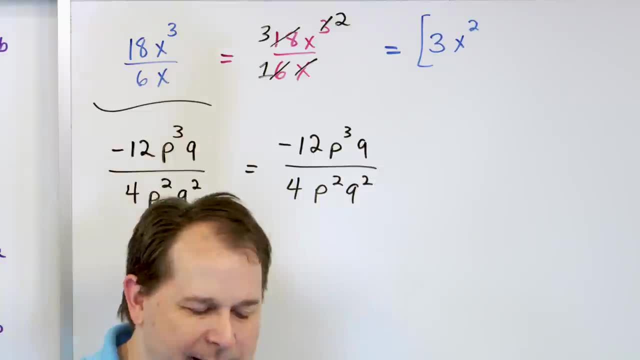 be marked up and you'll never be able to see what you started with. Besides, I'm using colored markers, but when you're using a pencil you can't really. there's no color there, So it's hard to see what you wrote down initially. So write it down again before you start messing. 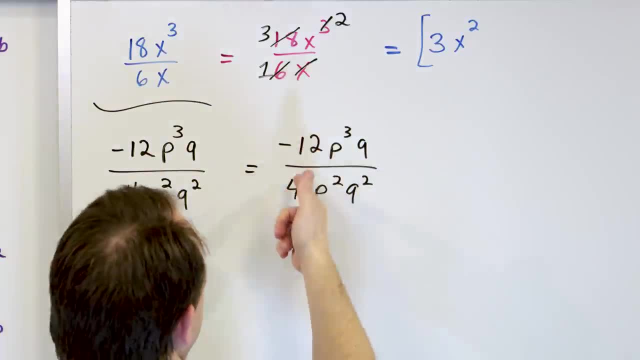 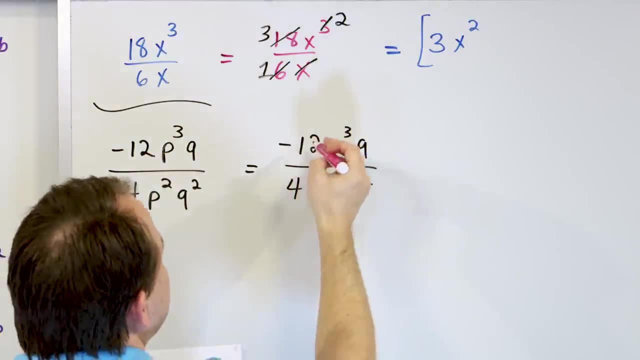 around with it. So we talk about the numbers first. I know you all know that 12 divided by four is three, but I want you to think about dividing the top and the bottom by some common number. So we'll divide the- uh, the 12 divided by four is going to give me three, and the four 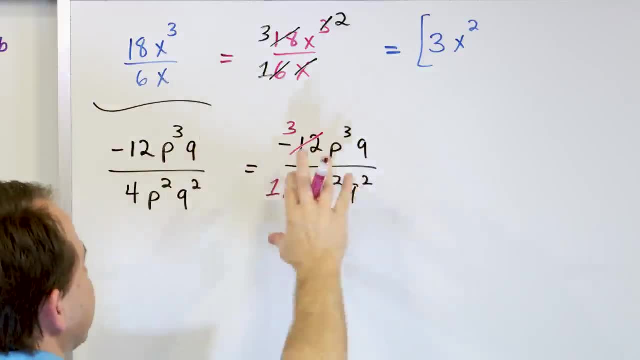 divided by four is going to give me one. The negative doesn't divide away with anything. It's still there. So we still have a negative. but this 12 becomes a three and the four becomes a one. And then we look at the p's. So we say what's going to happen? here We have 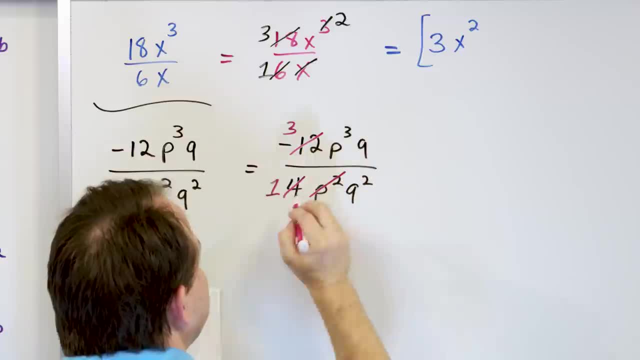 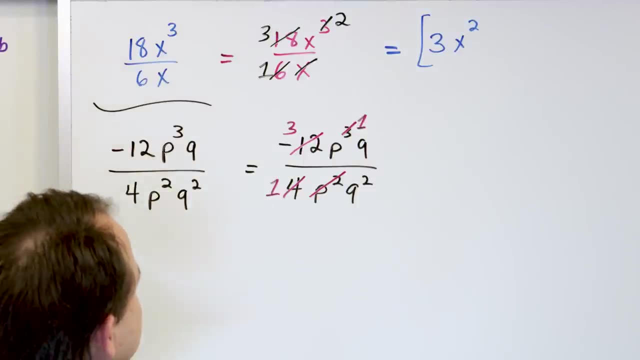 two p's here and we have three p's on top, So we can use both of those p's to cancel with two of them up here, but it's still going to leave a one behind, So I put a little one there to let me know. 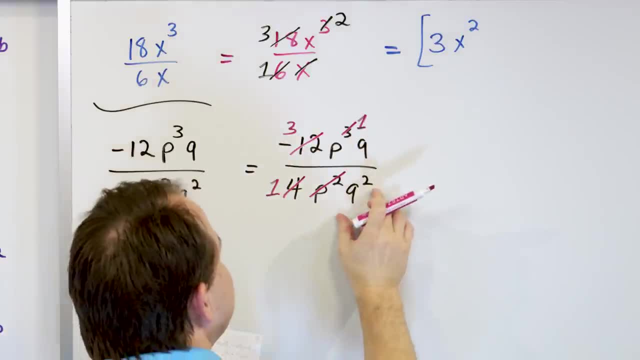 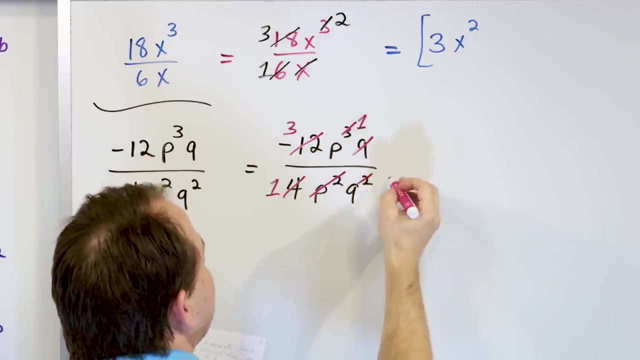 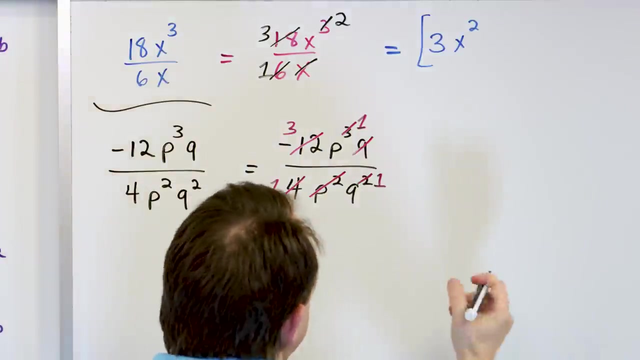 This p still has a first power right. And then the q's. here I have one q on the top and two q's on the bottom, So one q from the top can cancel with one from the bottom, leaving one behind. So you see, you get lots of markups here which can be hard to read, but you know. 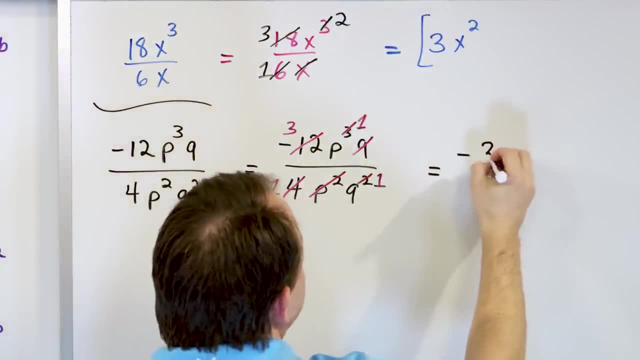 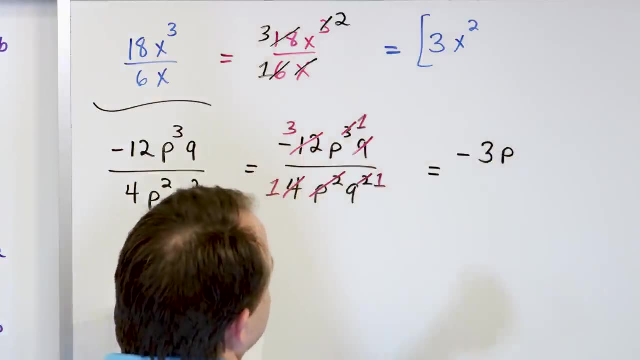 that's the way it goes. So you still have a negative, you have a three here, And then what you have is on the top: you have a p to the first power, So I don't need to write the first power, right. 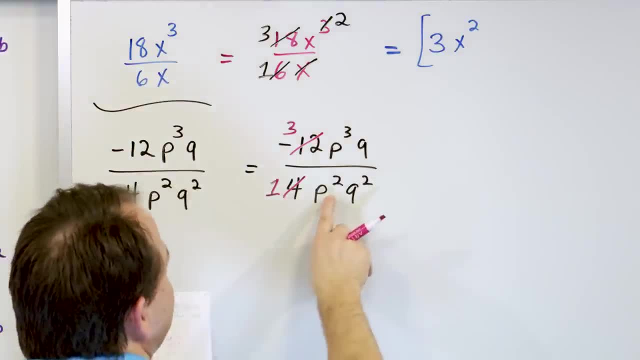 And then we look at the p's So we say what's going to happen here? We have two p's here and we have three p's on top, So we can use both of those p's to cancel with two of them. 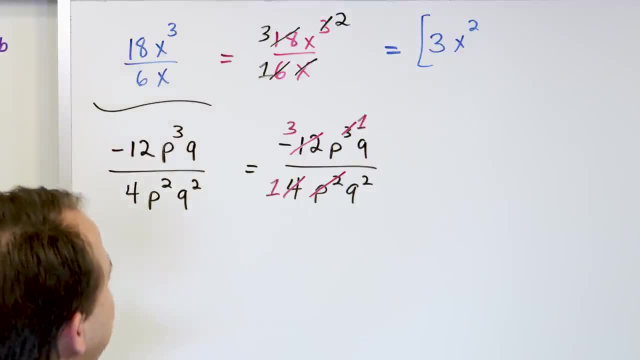 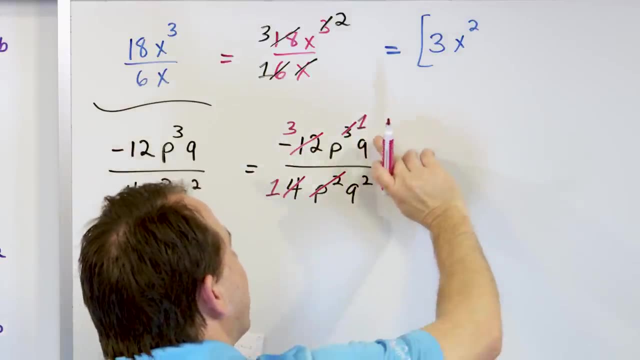 up here, But it's still going to leave a 1 behind. so I put a little 1 there to let me know this p still has a first power. And then the q's. here I have one q on the top and two q's on the bottom. 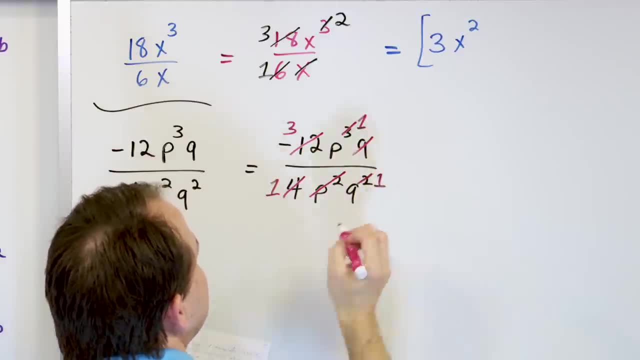 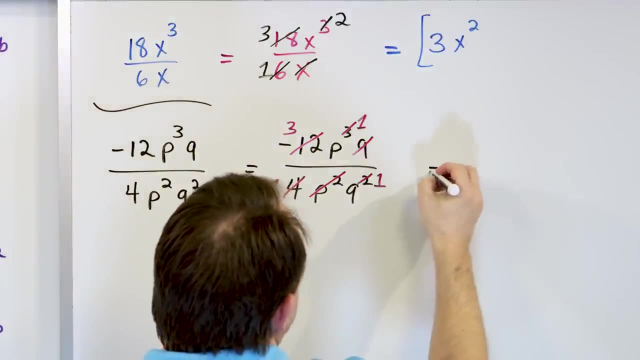 So one q from the top can cancel with one from the bottom, leaving one behind. So you see, you get lots of markups here which can be hard to read, But that's the way it goes. So you still have a negative. 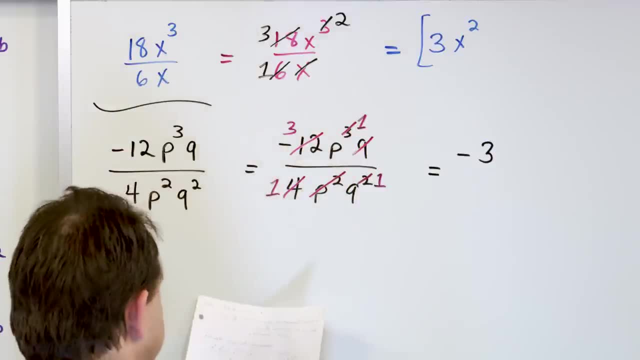 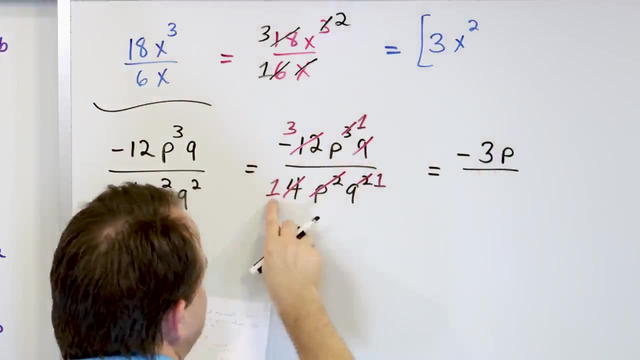 You have a 3 here And then what you have is on the top. you have a p to the first power, So I don't need to write the first power, right? This is gone. So on the bottom, I have a 1.. 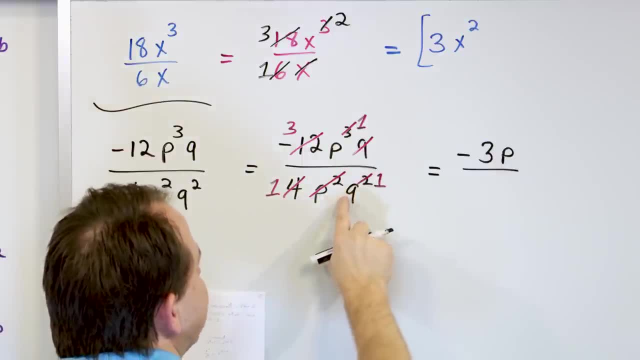 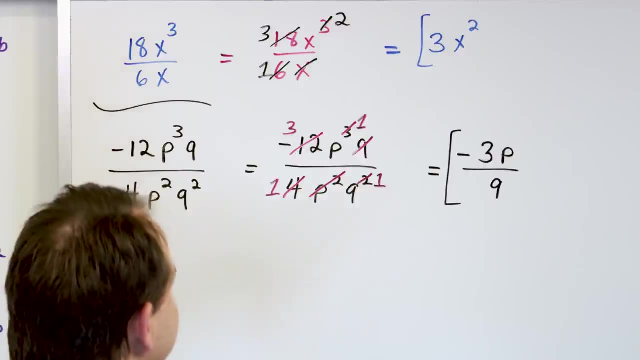 I don't need to write that. The p squared is completely marked out And the q is to the first power. So that's all I have left. negative 3p over q And that's the final answer. Now again, there's lots of ways to think about it. 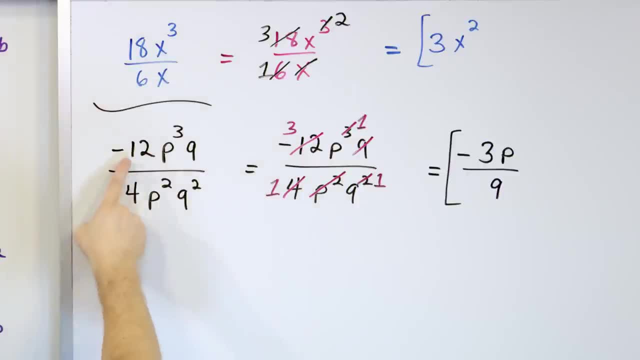 You can think about it like this: Instead of doing the simplification here, you can think of: 12 divided by 4 gives me 3. And of course the negative is still there. And then for the p's you could just subtract the exponents. 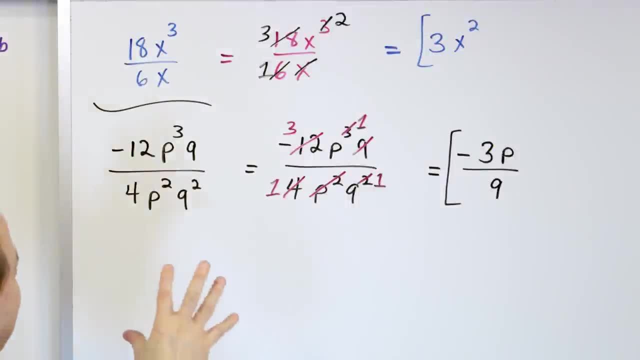 3 minus 2 is p to the first power. So again, there's lots of different ways to think about it. We can do it the way we've done it here, Or you can take a step back and say 12 divided by or negative. 12 divided by 4 is negative 3.. 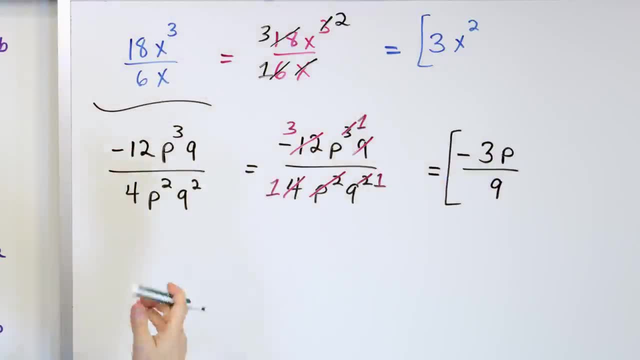 That's where that comes from, And then you can also think. I want you to think about just the p's for a second. What we had the p's here was p cubed over p squared, which is according to the rule over there. 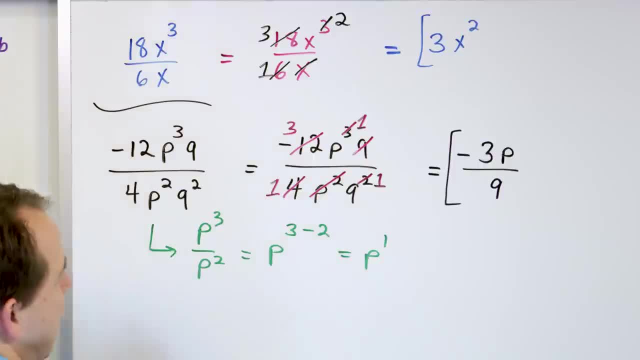 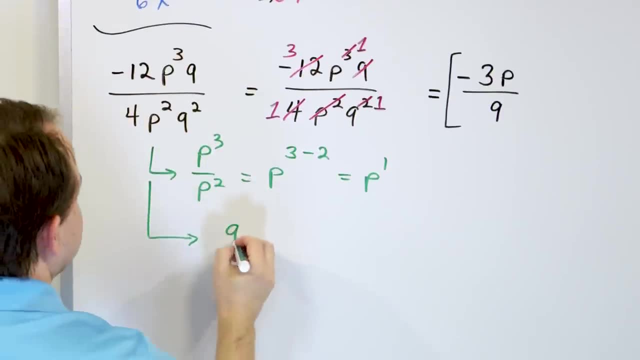 top exponent minus the bottom exponent, which is p to the first power. So that's why this is p to the first power. And then we can also look. Look at the q's right. We had a q on the top and a q squared on the bottom. 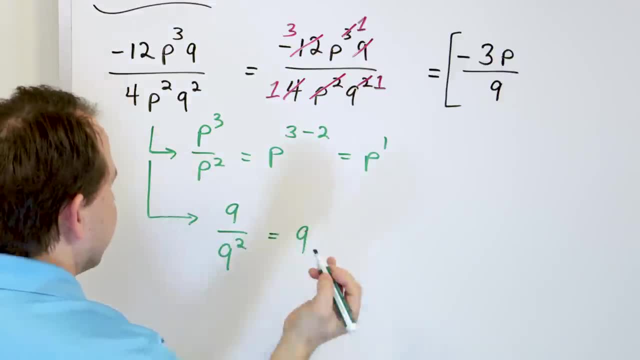 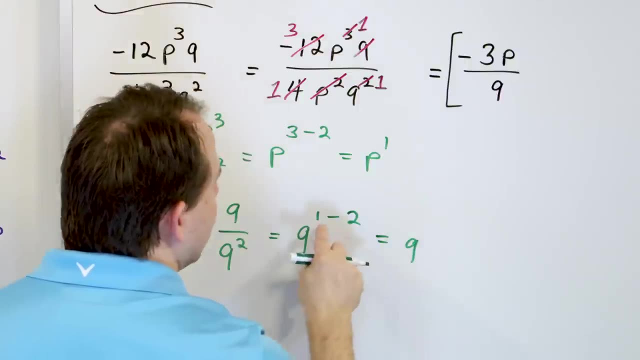 So this is a q on the top, which is q to the first power. So if you're going to do it by subtraction, you'd say 1 minus the bottom here, 1 minus 2.. But notice, what you get here is what is 1 minus 2?. 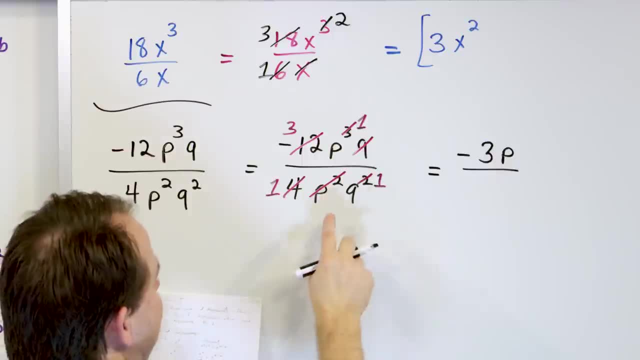 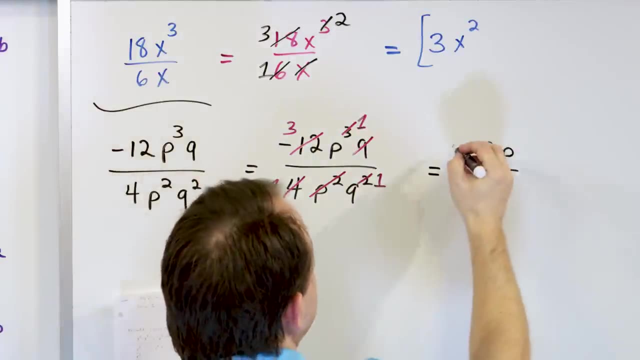 This is gone. So on the bottom I have a one. I don't need to write that. The p squared is completely marked out and the q is to the first power. So that's all I have left. Negative three p over q And that's the final answer. 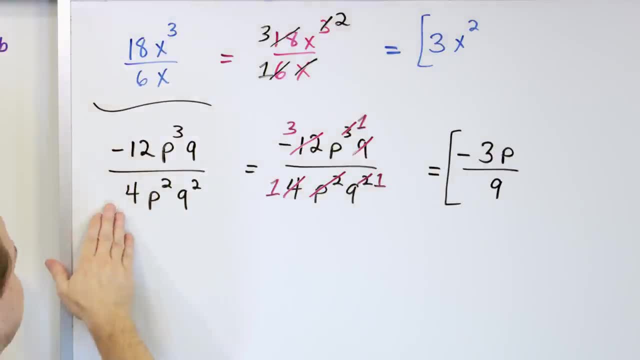 Now again, there's lots of ways to think about it. You can think about it like this: Instead of doing the simplification here, you can think of: 12 divided by four gives me three, And of course the negative is still there. And then for the p's, you could just subtract. 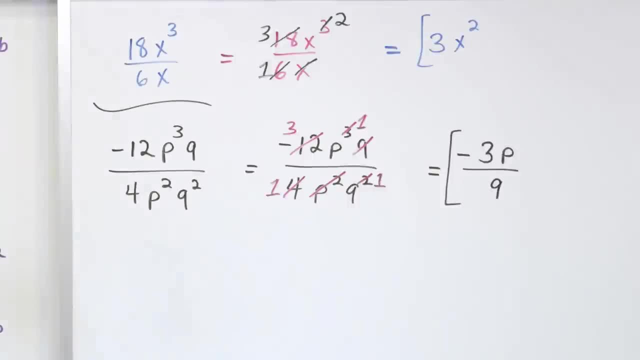 the exponents Three minus two is p to the first power. So again, there's lots of different ways to think about it. You can do it the way we've done it here, or you can take a step back and say 12 divided. 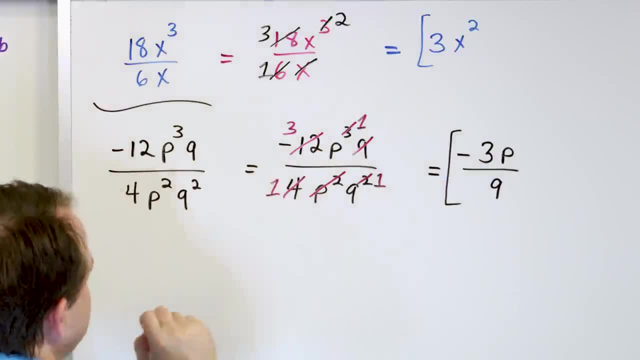 by or negative. 12 divided by four is negative three. That's where that comes from, And then you can also think. I want you to think about just the p's for a second. What we had, the p's here, was p cubed over p squared, which is, as, according to the rule over there, top. 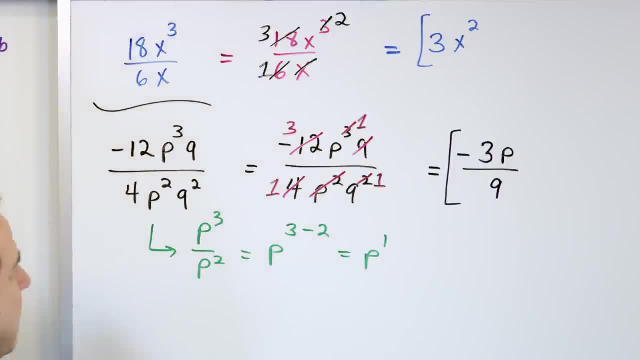 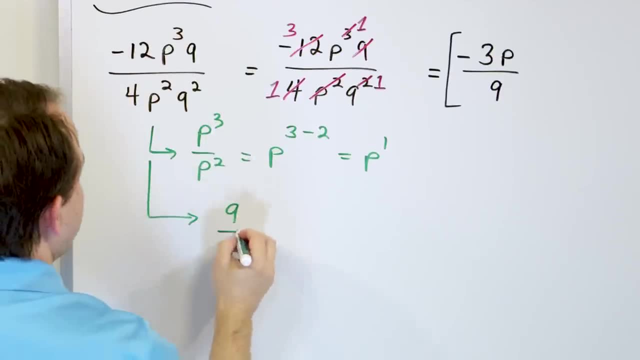 exponent minus the bottom exponent, which is p to the first power. So that's why this is p to the first power. And then we can also look at the q's right. We had a q on the top And a q squared on the bottom, So this is a q on the top, which is q to the first power. 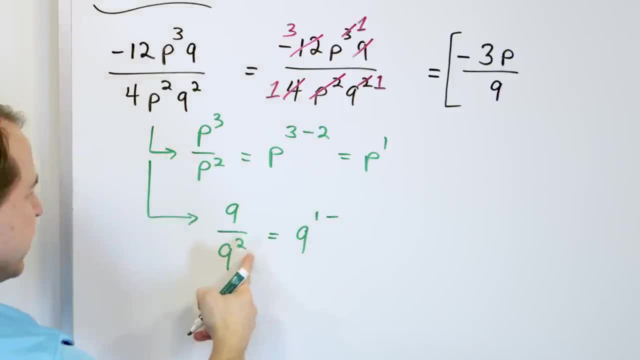 So if you're going to do it by subtraction, you'd say one minus the top, the bottom here one minus two. But notice what you get here is what is one minus two Negative one. Now we have not covered negative exponents in this class yet, We're going to cover negative. 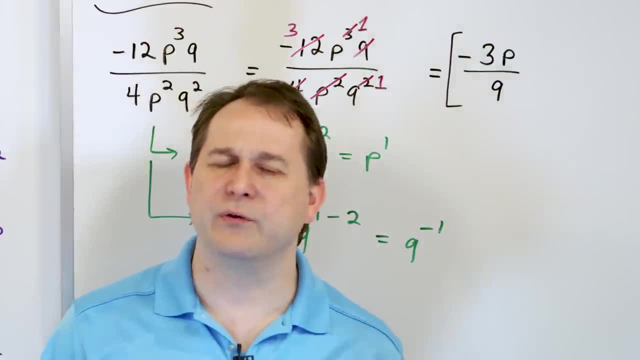 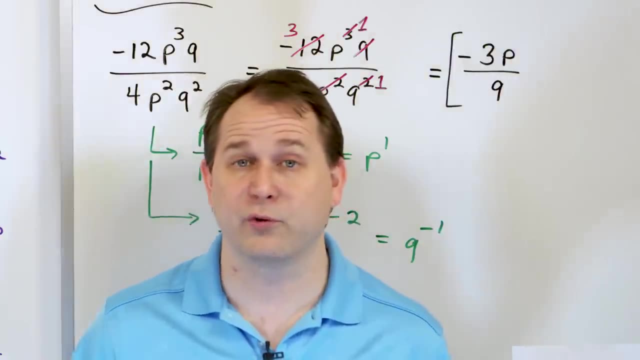 exponents- a few lessons from now, but it's kind of a preview to let you know that there are. there is such a thing as a negative exponent and you need to get comfortable, A comfortable some sort of way, with seeing negative exponents. For now we're not going. 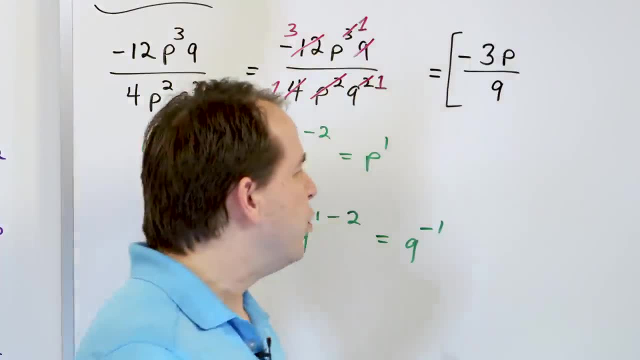 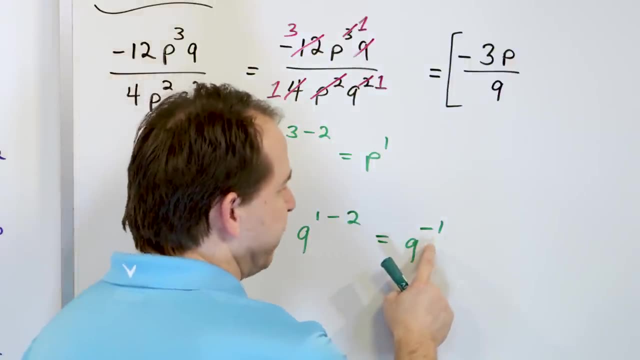 to go into it too much because I want to do a complete lesson on that, But if you do this thing by subtraction and you happen to see a negative exponent, all it means is that the q to the first power doesn't live upstairs. The negative exponent means that the q to 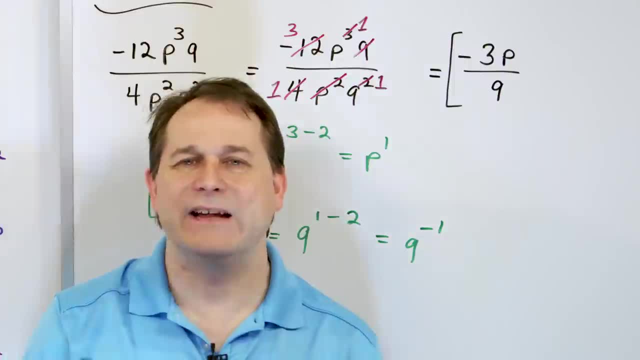 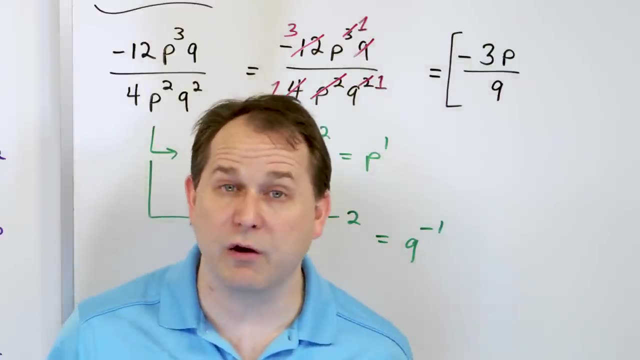 Negative 1.. Now we have not covered negative exponents in this class yet. We're going to cover negative exponents a few lessons from now, But it's kind of a preview to let you know that there is such a thing as a negative exponent. 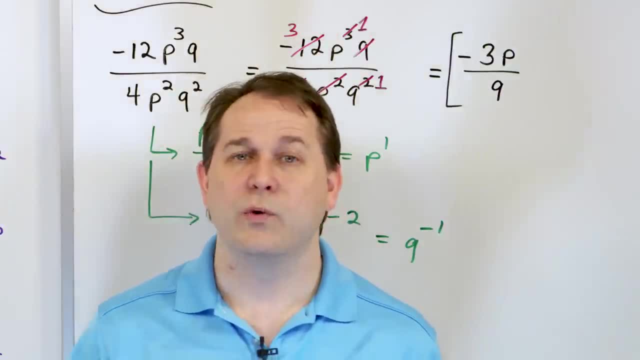 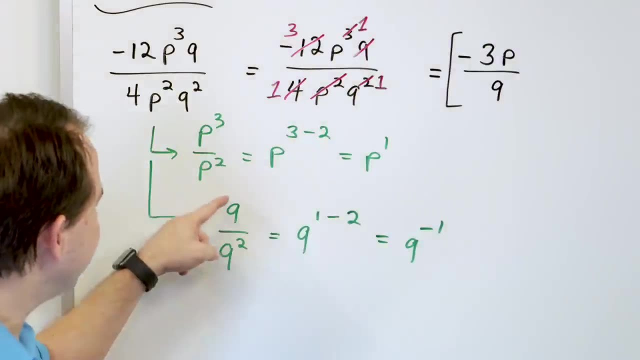 And you need to get comfortable some sort of way with seeing negative exponents. For now we're not going to go into it too much because I want to do a complete lesson on that. But if you do this thing by subtraction, 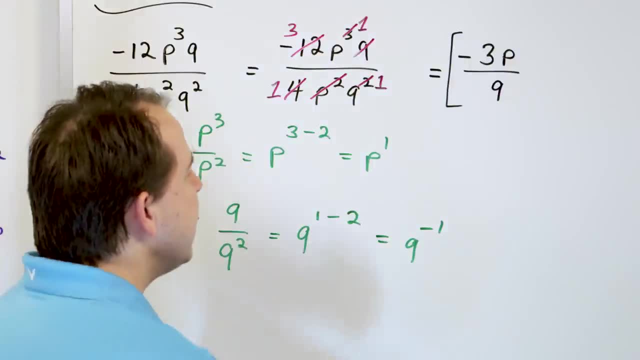 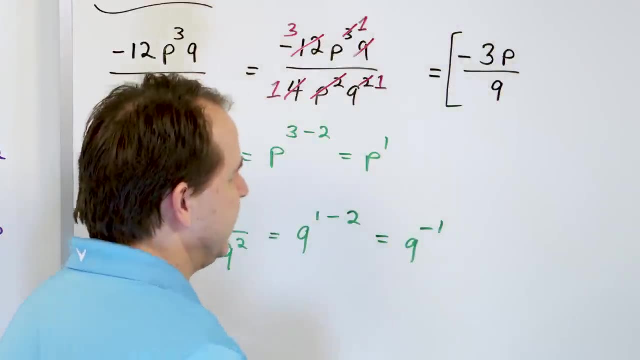 and you happen to see a negative exponent, all it means is that the q to the first power doesn't live upstairs. The negative exponent means that the q to the first power lives downstairs. So any time you see a negative exponent in algebra, it means that you can write it as a negative exponent. 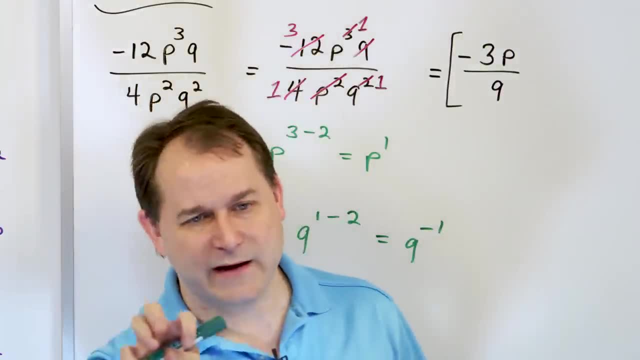 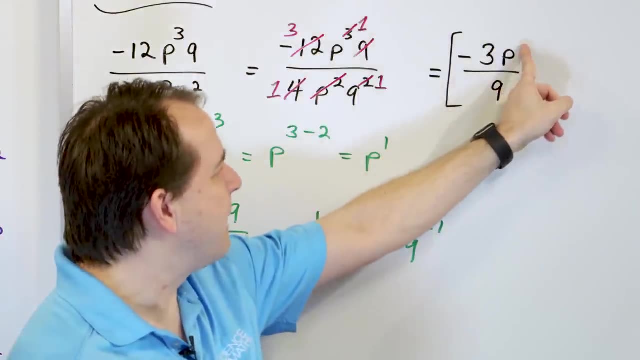 and it's going to be a positive exponent. Sure, you can leave it there, Or you can move it downstairs underneath the fraction and make it a positive exponent. That is what a negative exponent means. Positive exponents live on top of the numerator. 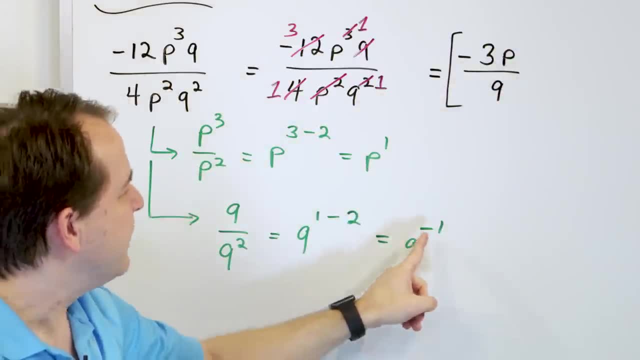 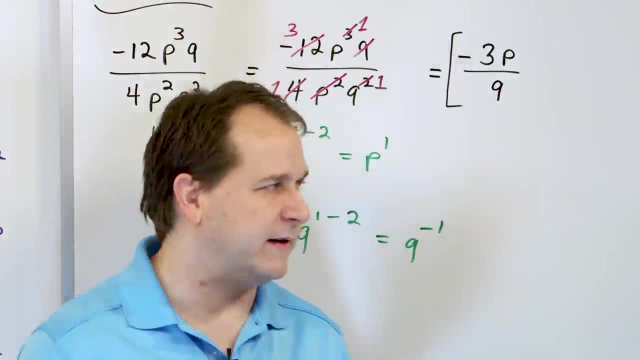 Negative exponents get moved downstairs. Notice he's a q to the first power. The negative implies or means that that exponent actually lives in the bottom of the denominator. So we're going to get into a whole lesson like that. So, because of the fact that you sometimes 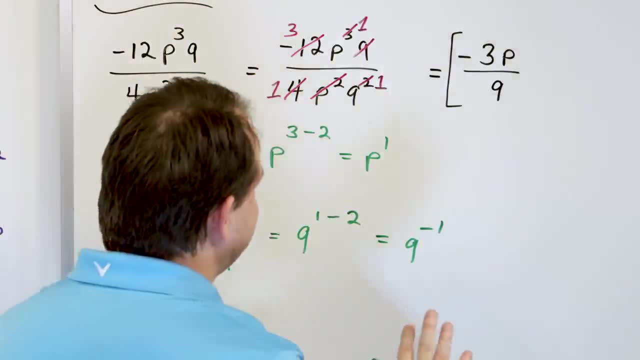 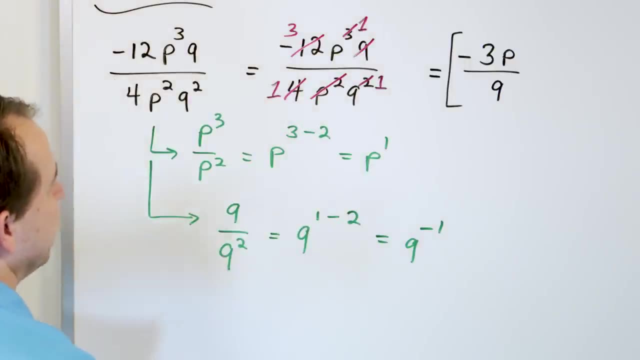 get these negative exponents and because of the fact that we haven't really talked too much about negative exponents yet, typically the way I like to solve these problems is just by canceling things, And that's how I'm going to solve the rest of these problems. 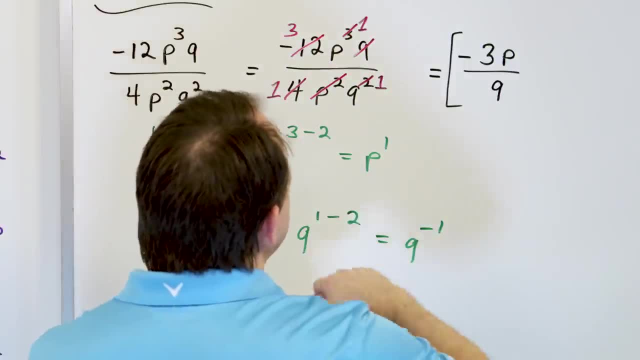 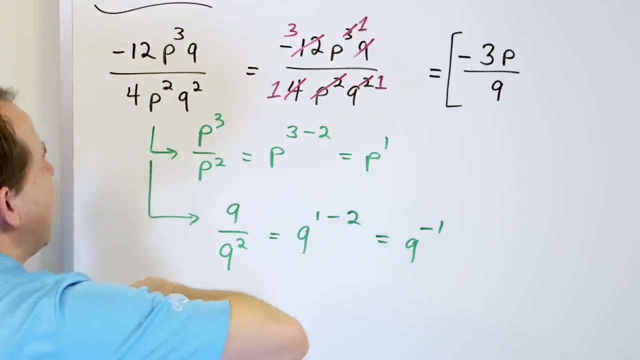 The only other thing I'll say before we continue solving these problems is notice that we had p cubed. Let me gesture here. We had p cubed and we had p squared, So we have two p's and three p's. So when I said we can sacrifice or cancel both of the p's, 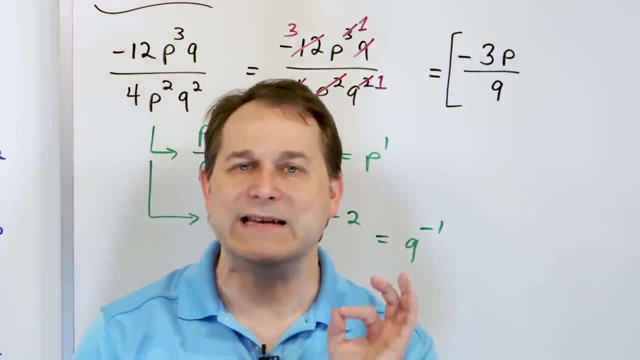 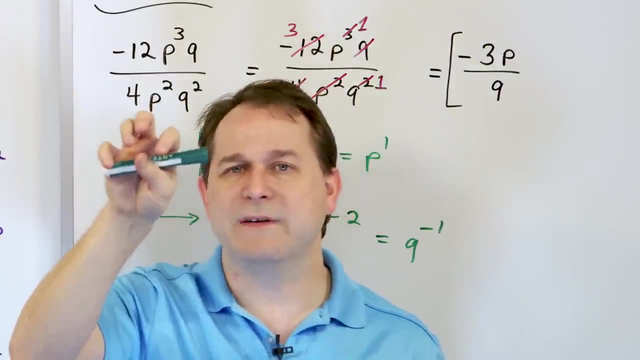 the first power lives downstairs, So anytime you see a negative exponent in algebra, it means that you can write it as a negative exponent. Sure, You can leave it there, or you can move it down Downstairs underneath the fraction and make it a positive exponent. That is what a negative 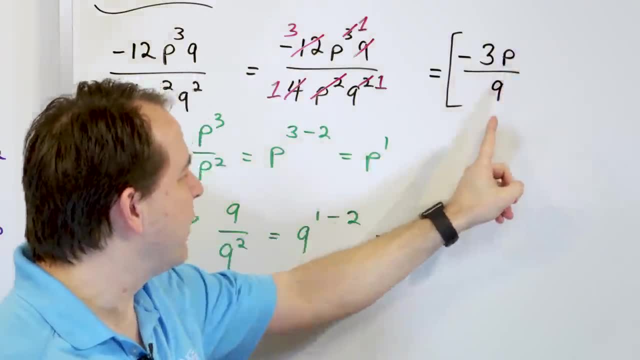 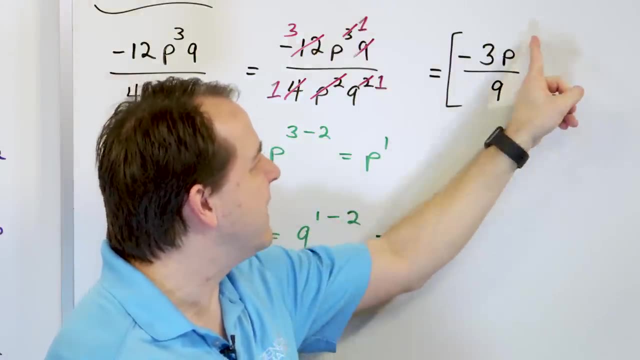 exponent means Positive exponents live on top of the numerator. Negative exponents get moved downstairs. Notice he's a q to the first power. The negative implies or means that that exponent actually lives in the bottom of the denominator. So we're going to get. 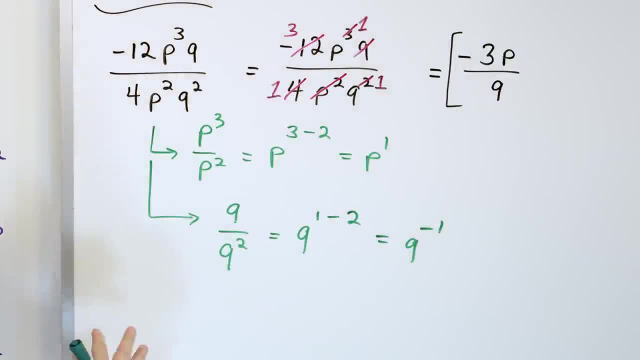 into a whole lesson like that. So, because of the fact that you sometimes get these negative exponents and because of the fact that we haven't really talked too much about negative exponents yet, What I like to solve these problems is just by canceling things, And that's how I'm going. 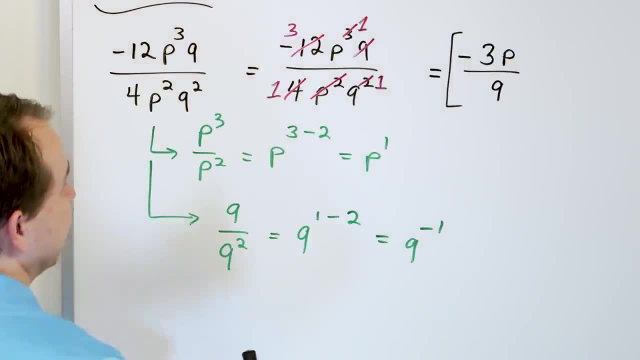 to solve the rest of these problems. The only other thing I'll say before we continue solving these problems is: notice that we had p cubed. Let me gesture here. We had p cubed and we had p squared. So we have two p's and three p's. So when I said we can sacrifice or cancel, 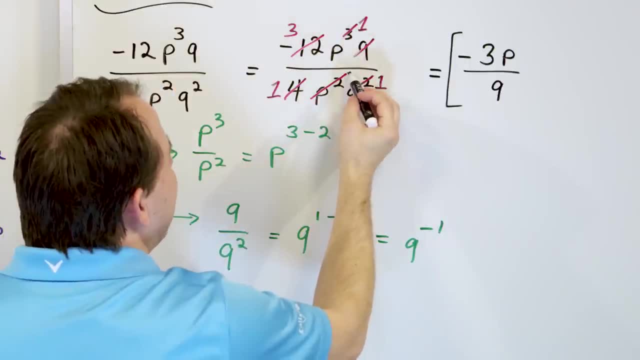 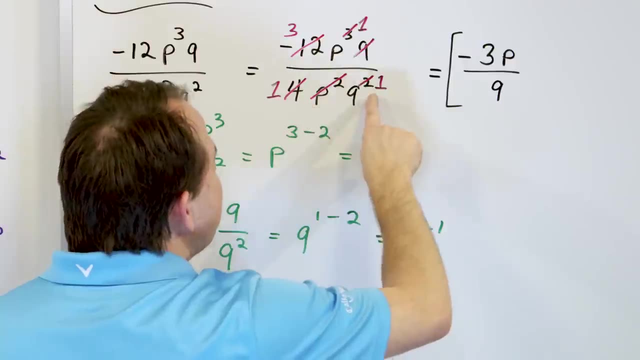 both of the p's on the bottom notice that I drew the strikethrough through the two and also through the p. That tells me when I go to my next step that I've killed all of it down here. So if I go to the exponent just through the two and write a number next to it, that means 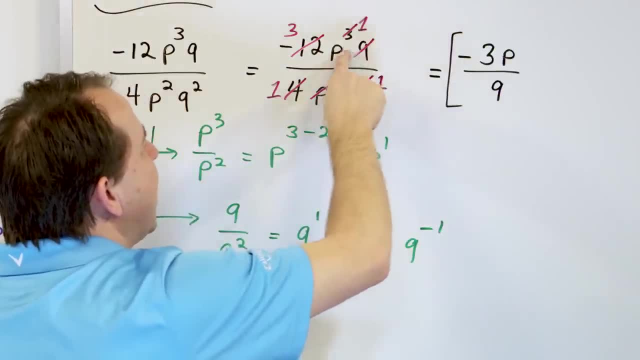 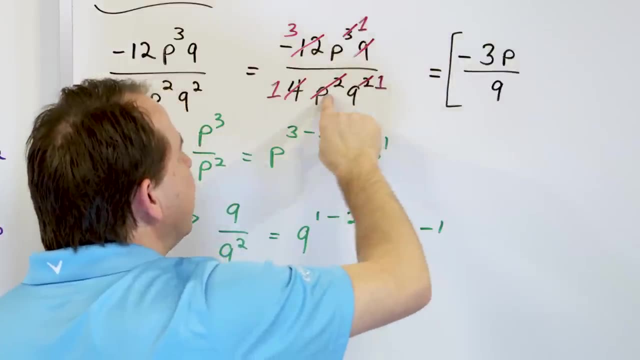 the variable is still there with a new exponent. Here I struck through the three and I wrote down a one. That means it's p to the one. Here I struck through the variable. That means it's gone. Here I struck through the p squared. That means it's gone, And so you need to kind. 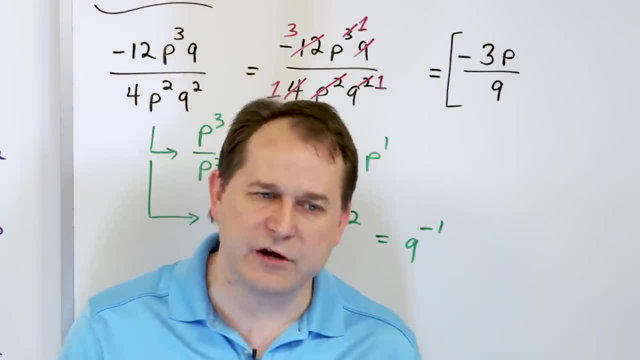 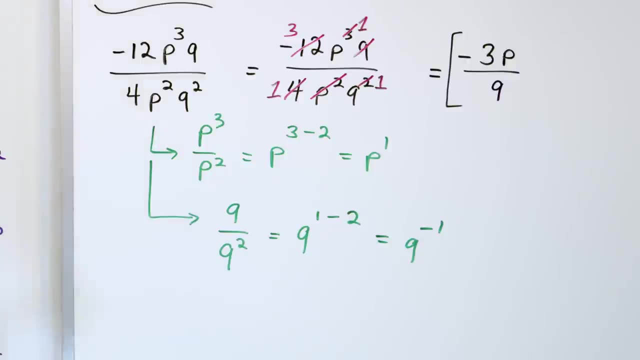 of practice. it, It all takes practice, But it's just a methodology that we use to help us remember what we're doing in the next step. All right, So let's go and solve a few more of these. We have a few more problems. They're going to get more complicated, but they're 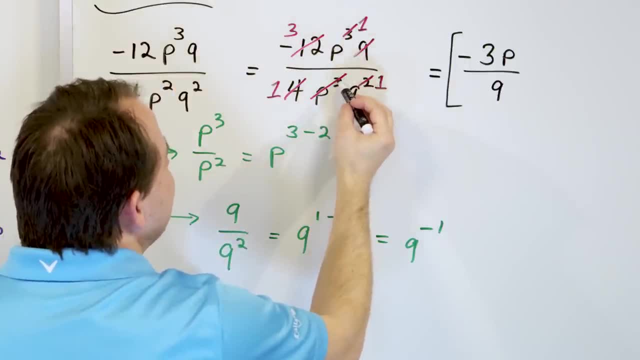 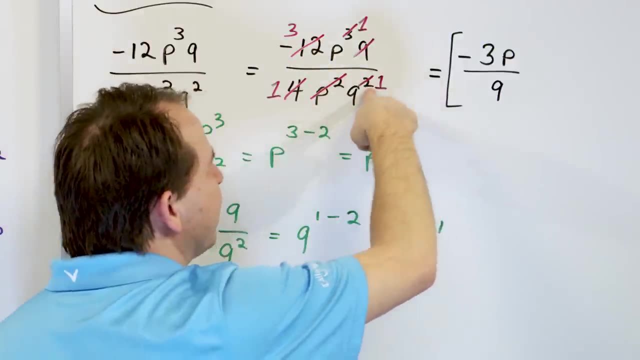 on the bottom notice that I drew the strikethrough through the two and also through the p. That tells me when I go to my next step that I've killed all of it down here If I only strike through the exponent just through the two. 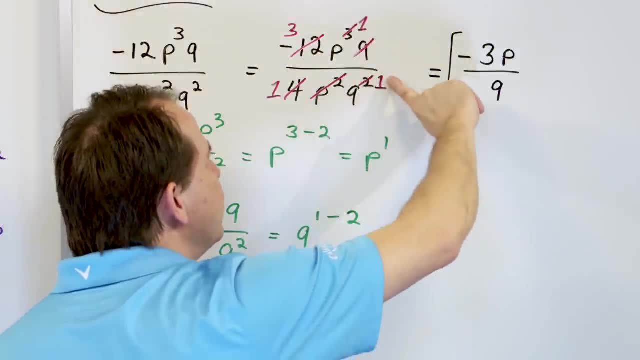 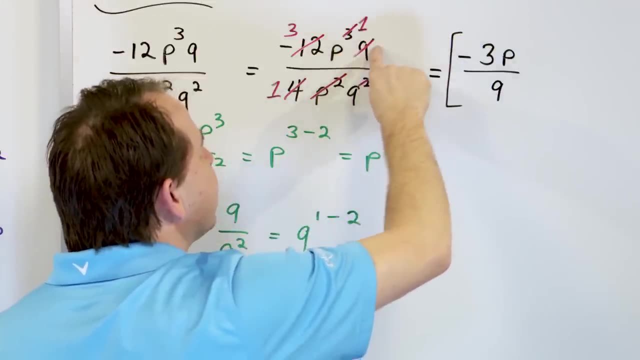 and write a number next to it. that means the variable is still there. with a new exponent: Here I struck through the three and I wrote down a one. That means it's p to the one. Here I struck through the variable. That means it's gone. 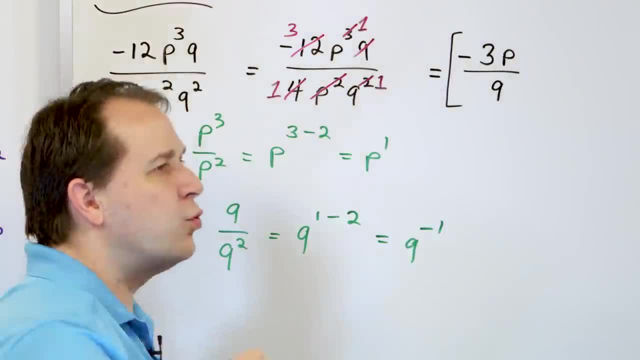 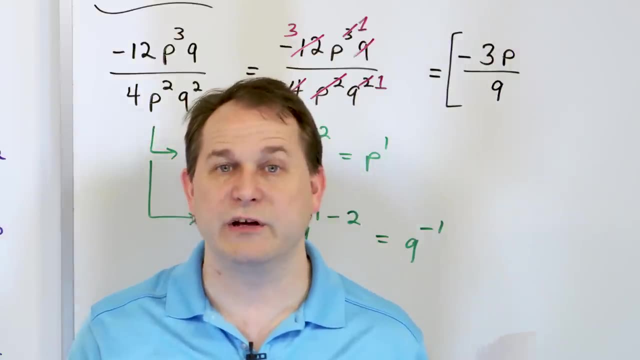 Here I struck through the p squared. That means it's gone, And so you need to kind of practice it. It all takes practice, But it's a methodology that we use to help us remember what we're doing in the next step. All right, so let's go and solve a few more of these. 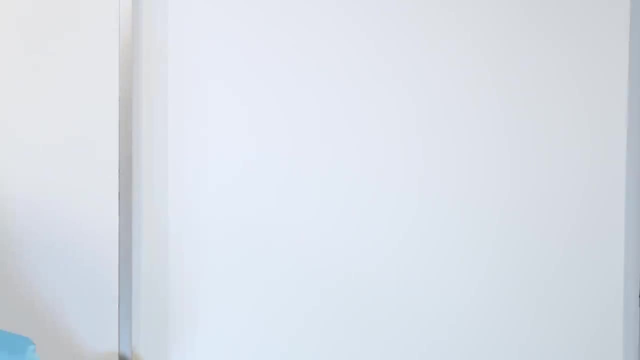 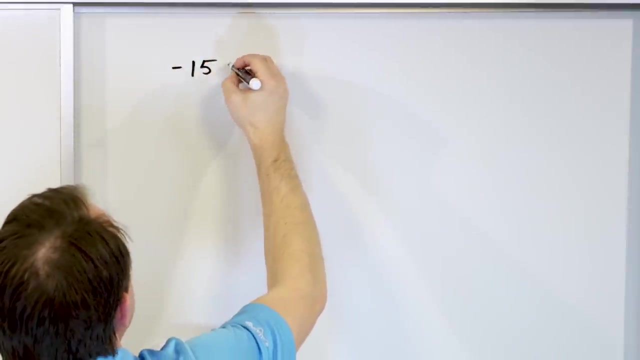 We have a few more problems. They're going to get more complicated, but they're all going to follow exactly the same pattern as what we have done here. What if we have negative 15? u to the fifth power, v to the third power? 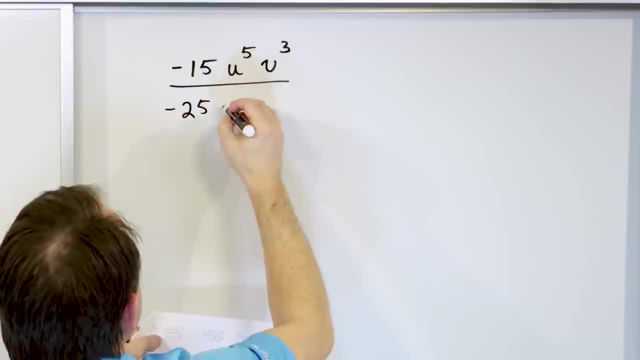 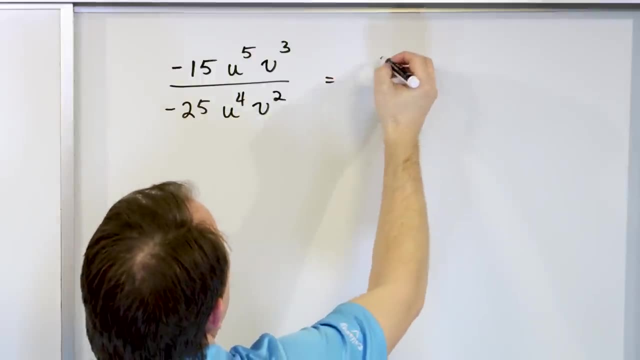 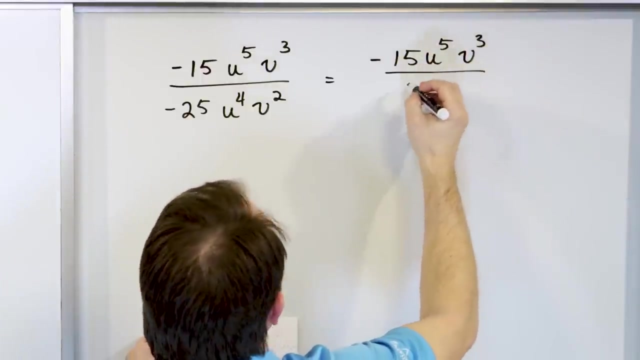 And on the bottom we will have negative 25? u to the fourth power, v to the second power. Now again, same sort of thing. I'm going to mark it up over here. So 15? u to the fifth power, v to the third power, over negative 25? u to the fourth power. 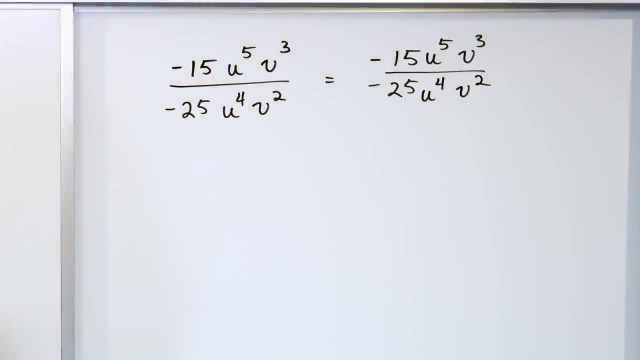 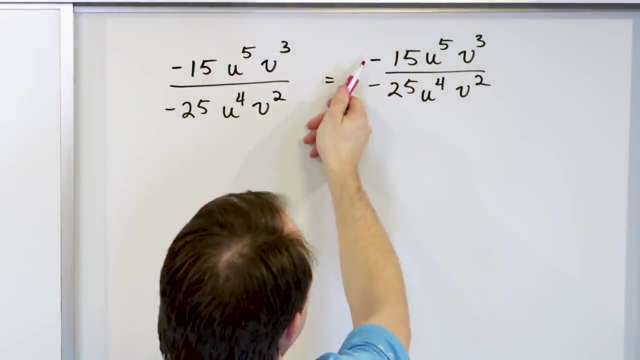 v squared. So we have to decide what to do. First we would tackle the numbers. We have 25 and 15.. So immediately you should think you can divide both of those by five. But we also have negative divided by negative. So you can kind of strike through both of those making them positive, because you all 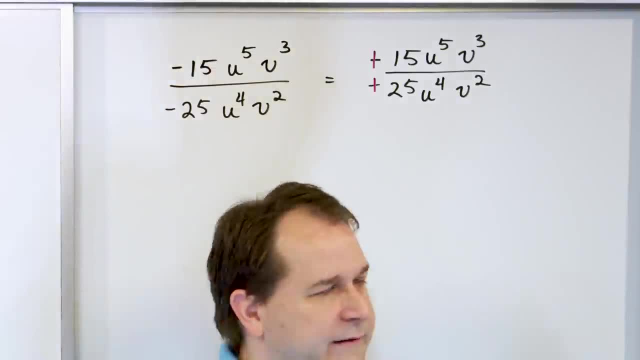 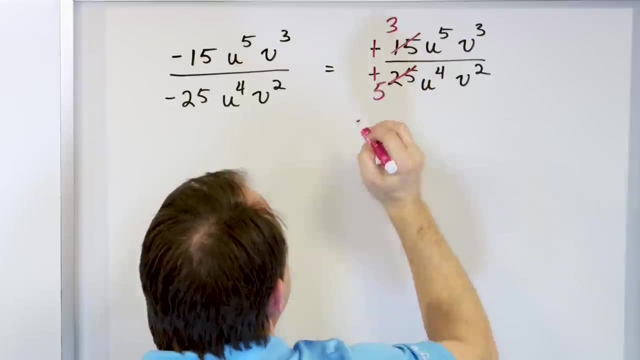 know that negative- anything divided by negative- always gives you a positive. And then for the 15, we'll divide by five, giving us three. The 25 divided by five will give us a five. So we have new numbers in there. We've simplified that fraction. 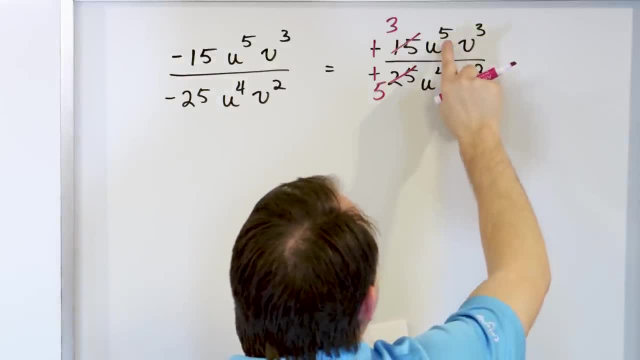 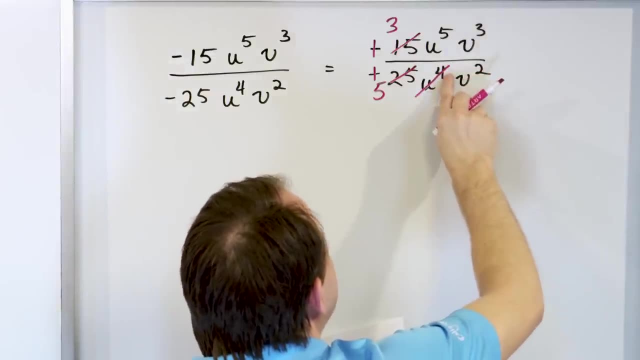 And then we look at the u's: There's four on the bottom and five on the top. Everything's multiplied. So I cancel all four of these u's, meaning I strike through the whole thing, including the u and the exponent On the top. I only have one left. 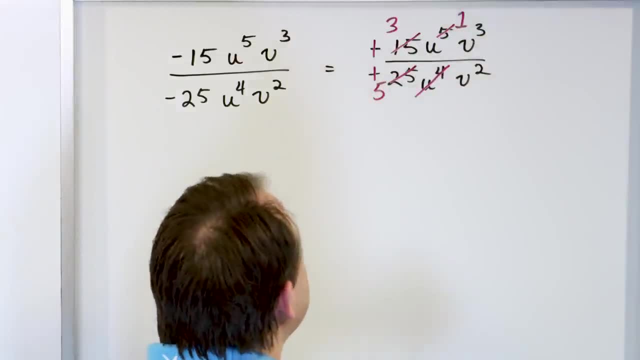 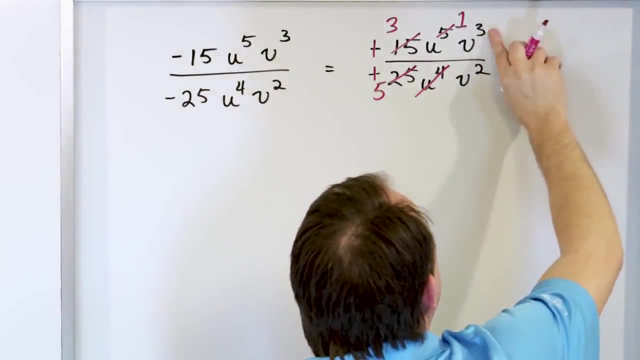 So I only strike through the five and I write the number one next to it, letting me know that I still have a u to the fifth power v to the fourth power v squared. Now on this one I have two v's and three v's on the top, so I can cancel both of the. 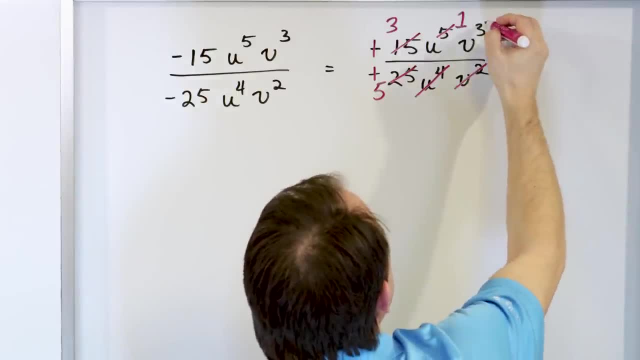 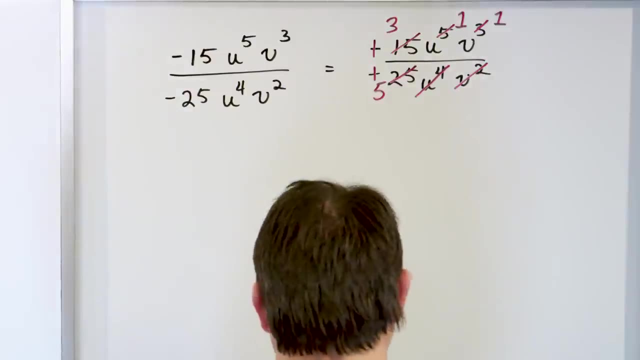 v's. I strike through the complete thing, including the base and the exponent. Here I strike through only the three, leaving me a one left, because if I have two on the bottom I cancel two up here. I have one left. 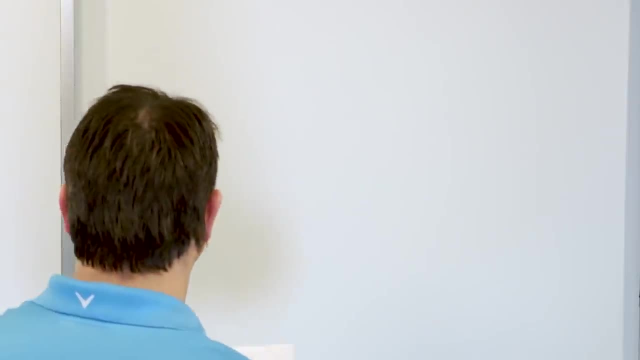 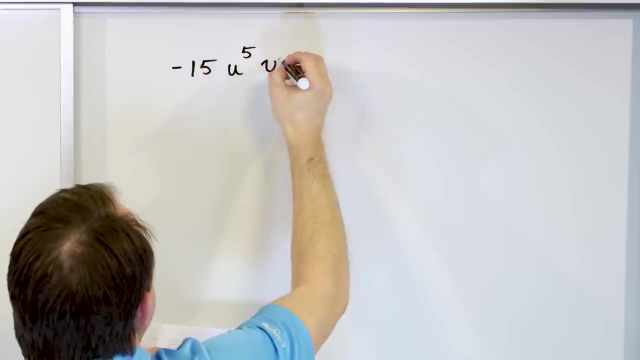 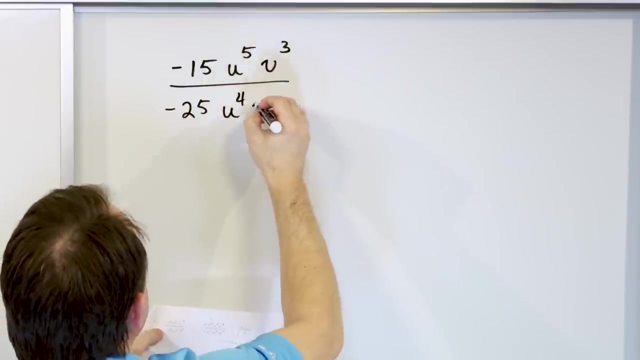 all going to follow exactly the same pattern as what we have done here. What if we have negative 15? u to the fifth power, v to the third power? And on the bottom we will have negative 25? u to the fourth power, v to the second power. Now again, same sort of thing. 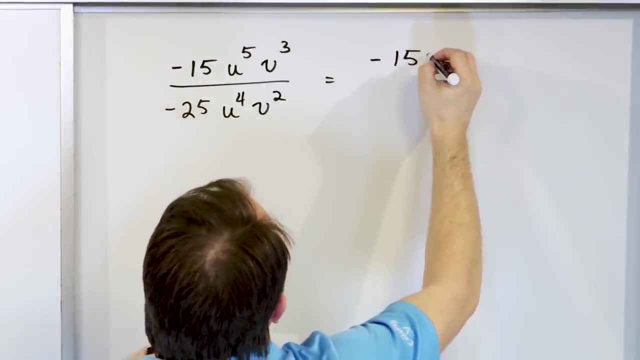 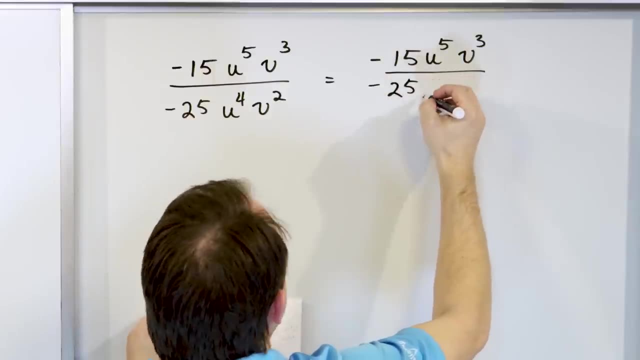 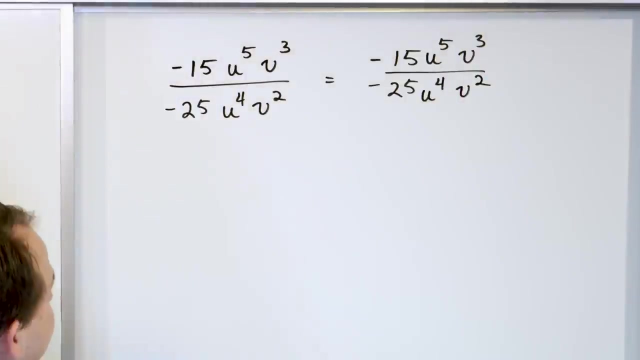 I'm going to mark it up over here. So 15? u to the fifth power, v to the third power, V to the third power over negative 25 u to the fourth power, v squared. So we have to decide what to do. First we would tackle the numbers We have: 25 and 15.. So immediately, 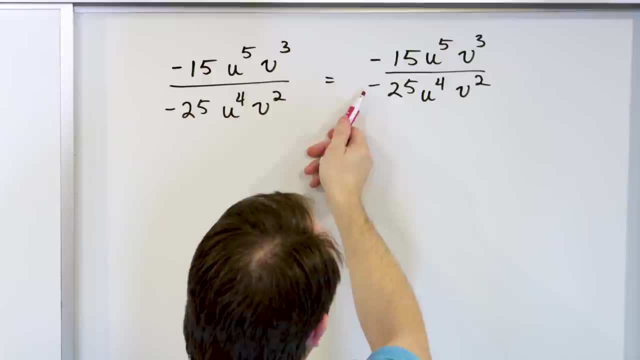 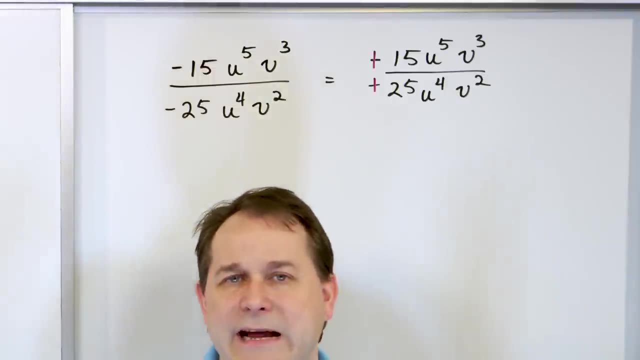 you should think you can divide both of those by five. But we also have negative divided by negative, So you can kind of strike through both of those, making them positive, because you all know that negative, anything divided by negative, always gives you a positive. And 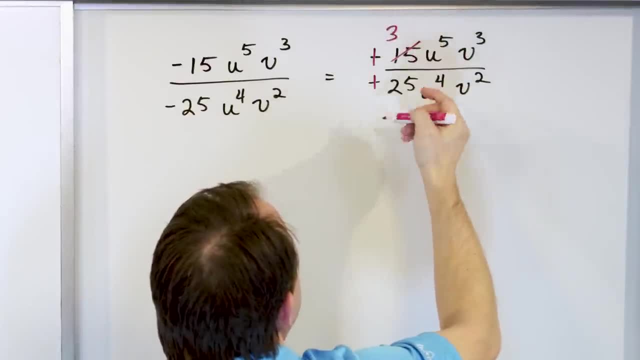 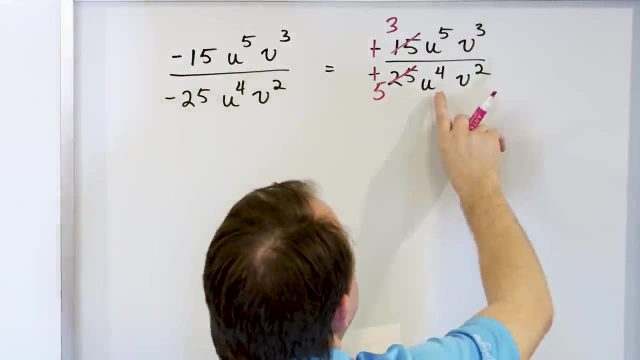 then for the 15 we'll divide by five, That's three. The 25 divided by five will give us a five. So we have new numbers in there. We've simplified that fraction. And then we look at the u's. There's four on the. 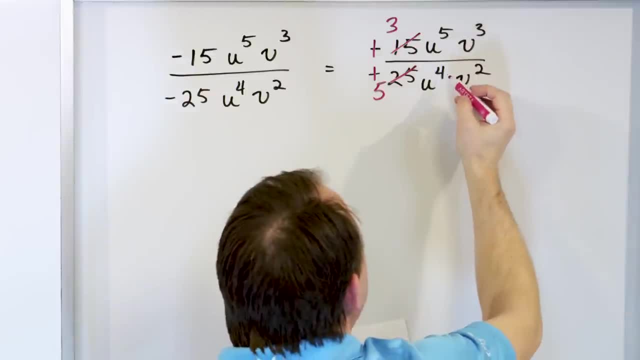 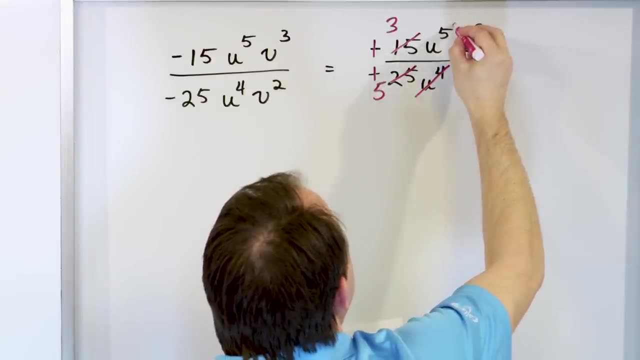 bottom and five on the top. Everything's multiplied. So I cancel all four of these u's meaning I strike through the whole thing, including the u and the exponent On the top. I only have one left, so I only strike through the five And I write the number one next to it. 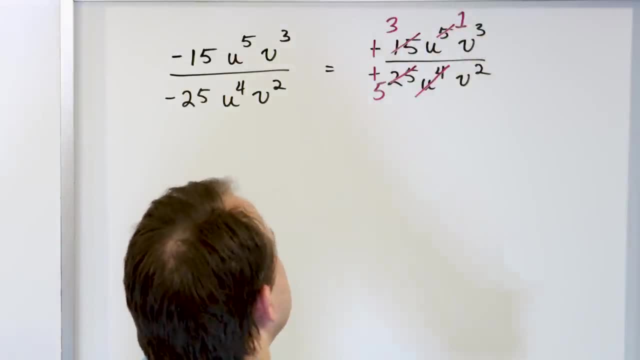 letting me know that I still have a? u to the first power. Now, on this one, I have two v's, V to the third power, v to the fourth power, v squared, So I have two v's. So I have two v's and three v's on the top, So I can cancel both of the v's. I strike through the complete. 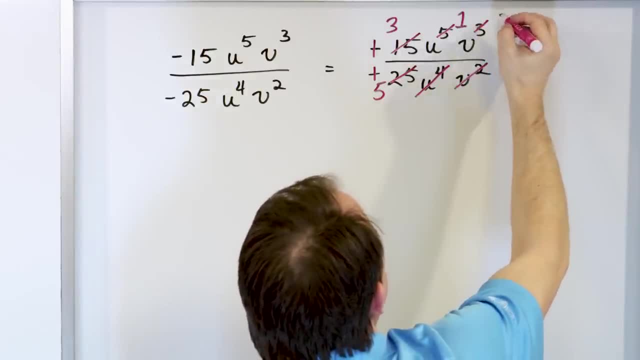 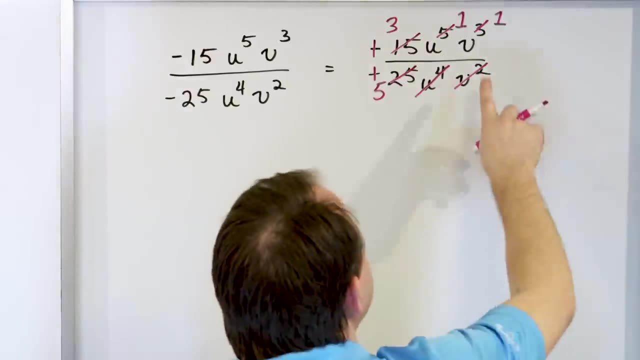 thing, including the base and the exponent. Here I strike through only the three, leaving me a one left, Because if I have two on the bottom, I cancel two up here. I have one left. So you see, what you're doing is you're subtracting exponents when you're writing the new numbers. 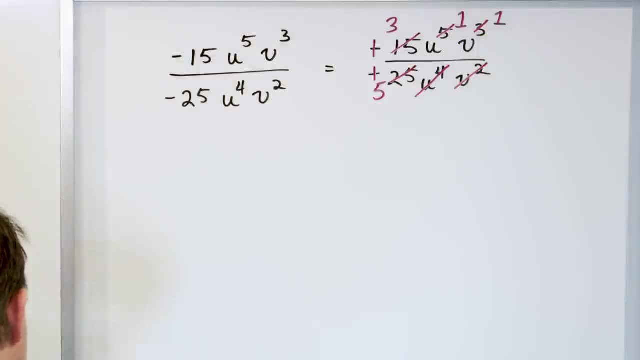 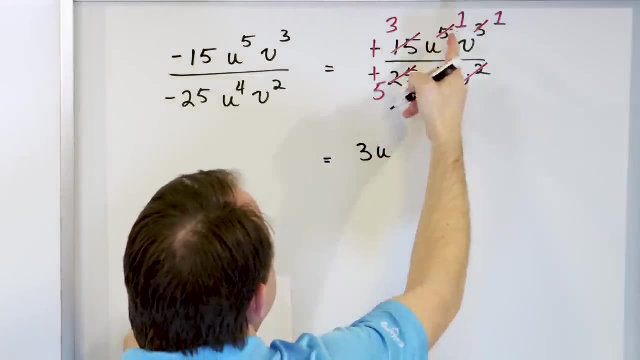 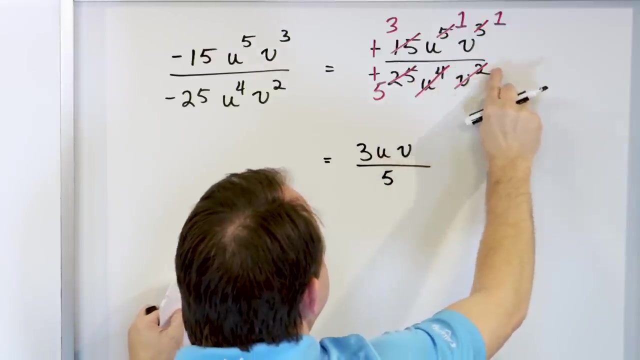 down up here. All right. So then, what we're going to have for our final answer is going to be positive: three? u to the first power, v to the first power. On the bottom, we will have five. But notice, we struck through all of this. It's totally. 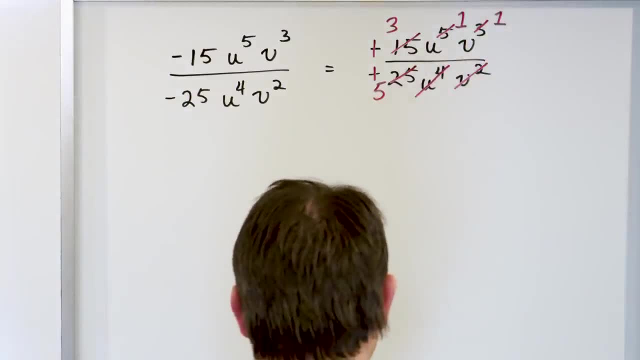 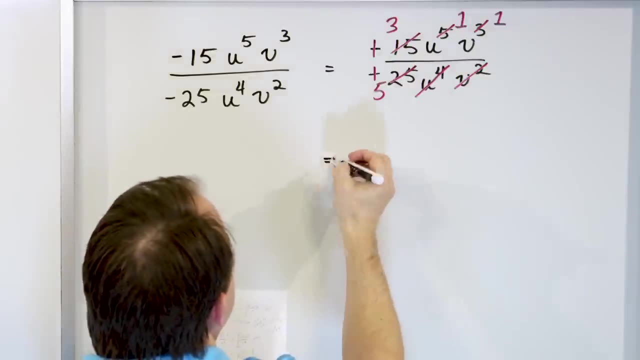 So you see, what you're doing is you're subtracting exponents when you're writing the new numbers down up here. So then, what we're going to have for our final answer is going to be positive. We're going to have three: u to the first power, v to the first power. 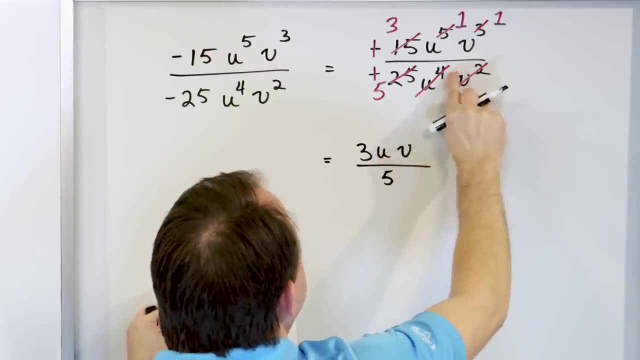 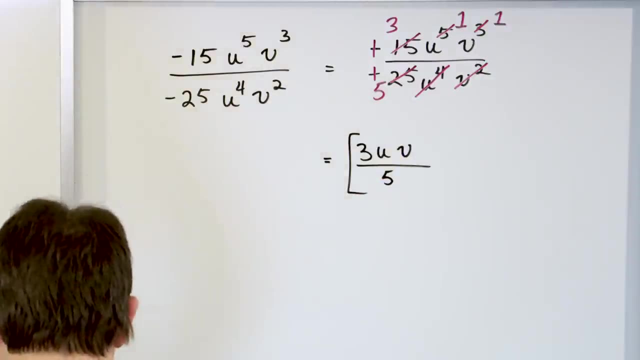 On the bottom we will have five. But notice, we struck through all of this- It's totally gone. so there's nothing else left except for the five on the bottom. So we have that as our final answer. So, again, that's doing it in the method of canceling things, but I want to show you how. 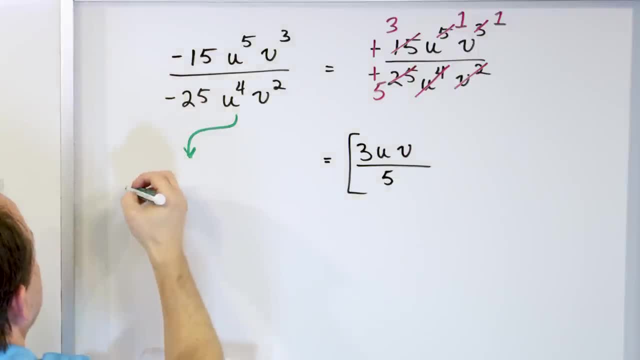 to think about different things. So let's talk about, forget about the numbers. let's talk about the? u to the fifth, v to the third over u to the fourth v squared. Let's do that, Let's talk about that. So, what you're going to have, you have u and u. 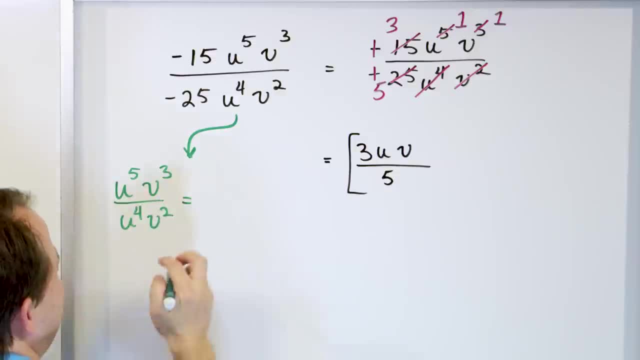 So you have these guys on the top and the bottom, different exponents, same base. So what you can have is you subtract the exponents five minus four and then you'll have that multiplied by the v terms. So you have v and you subtract these exponents three minus two. 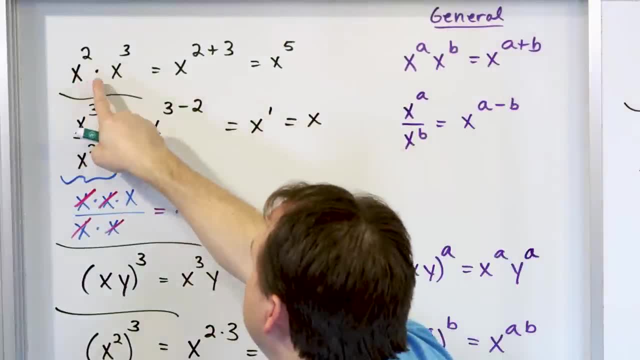 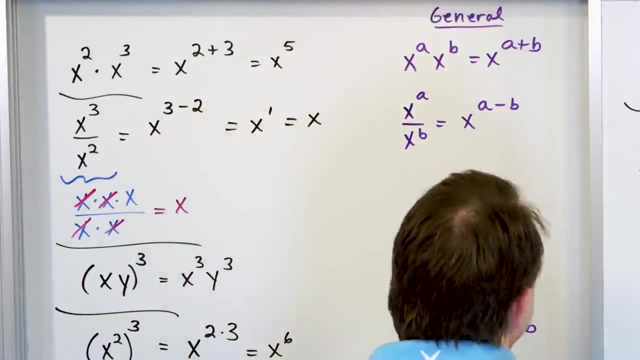 You see, all we're doing is using this rule here. When you multiply exponents or terms with the same base- different exponents- you add, But when you're dividing terms, you subtract the exponents. So all we're doing is we're saying we've got a division here and a division here. 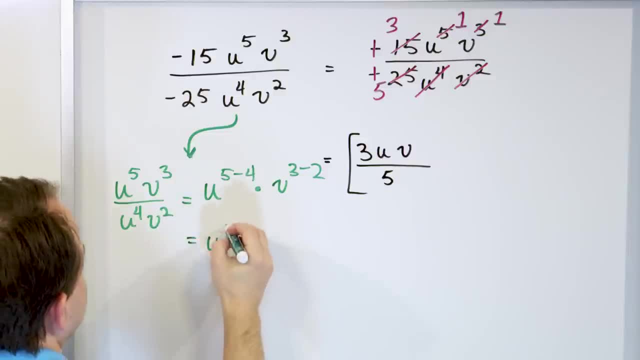 So we subtract the exponent, subtract the exponent, and of course, what you get is u to the first times, v to the first, which is exactly what we got for our final answer. Different ways to think about it. It's okay to think about either way to do it. 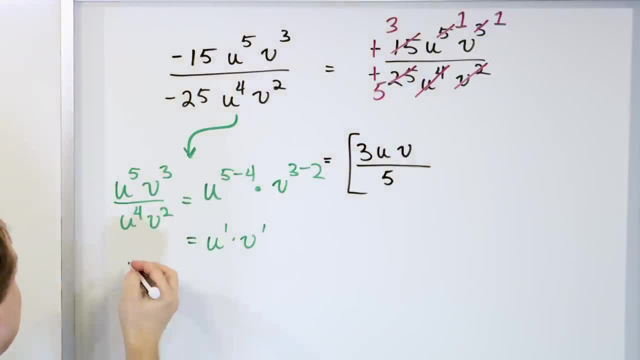 You can totally use this or you can do the cancellation method. I typically do the cancellation method. It becomes a little easier when the problems get harder. I think in order to do that, And also later on, I am going to introduce negative exponents, which it just depends. 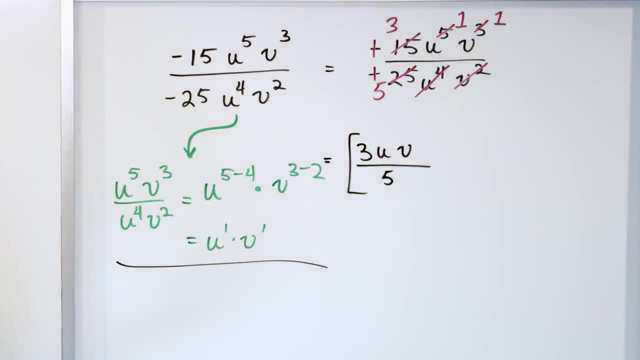 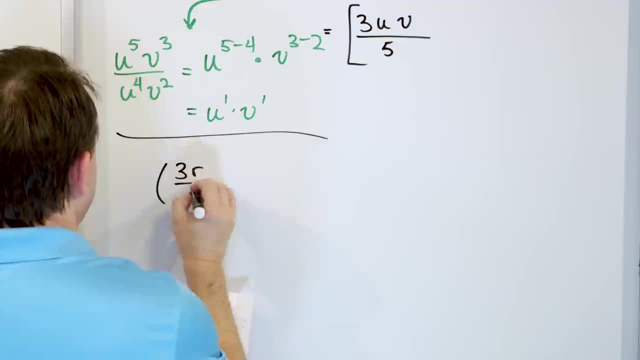 on the problem. There's no right answer, but typically I use this cancellation technique more than anything else. All right, Now let's move on to something a little different. What if we have three times r over s squared and that's a fraction, all raised to the third? 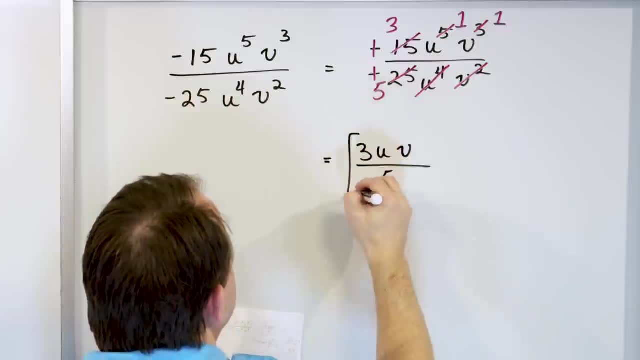 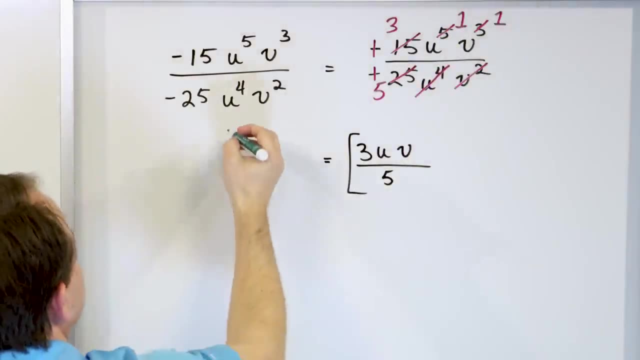 gone, so there's nothing else left except for the five on the bottom. So we have that as our final answer. So, again, that's doing it in the method of canceling things, But I want to show you how to think about different things. So let's talk about, forget about the numbers. let's 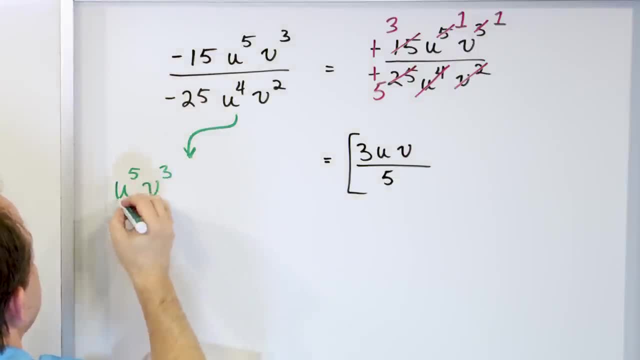 talk about the u to the fifth, v to the third over. u to the fourth v squared. Let's talk about that. So what you're going to have, you have u to the fourth v squared. So you're going to have u and u, So you have these guys on the top and the bottom different. 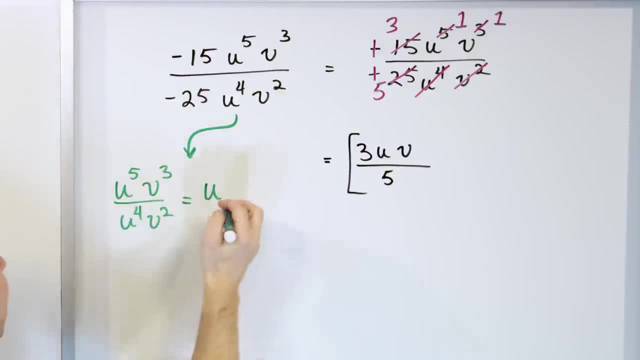 exponents same base. So what you can have is you subtract the exponents five minus four, And then you'll have that multiplied by the v terms. So you have v and you subtract these exponents three minus two. You see, all we're doing is using this rule here When 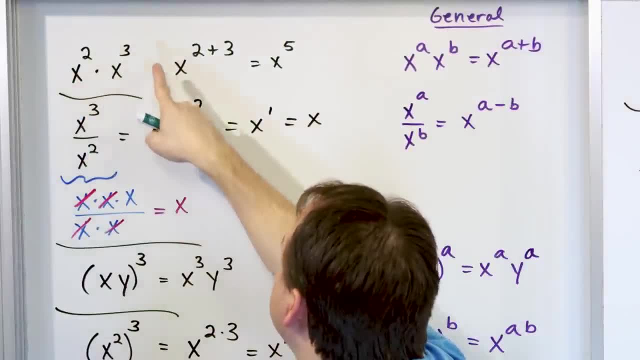 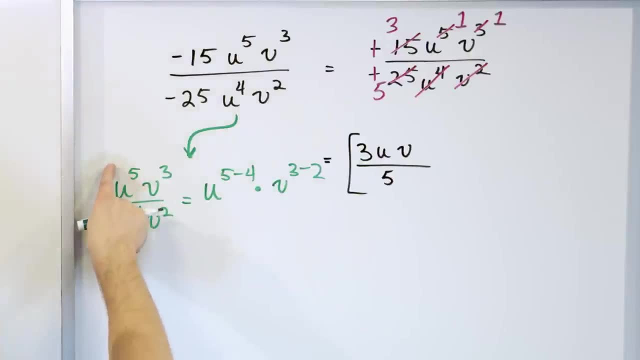 you multiply exponents or terms with the same base. different exponents you add, But when you're dividing terms you subtract the exponents. So all we're doing is we're saying we've got a division here and a division here, So we subtract the exponent. subtract the exponent. 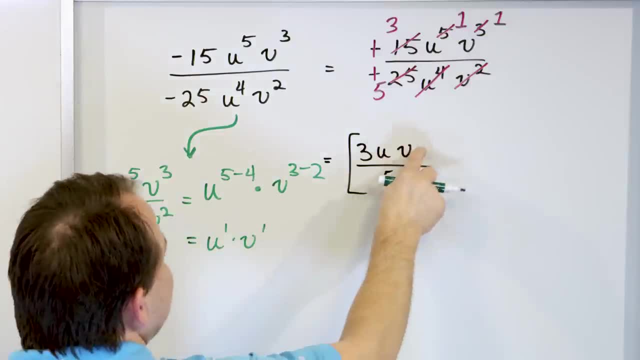 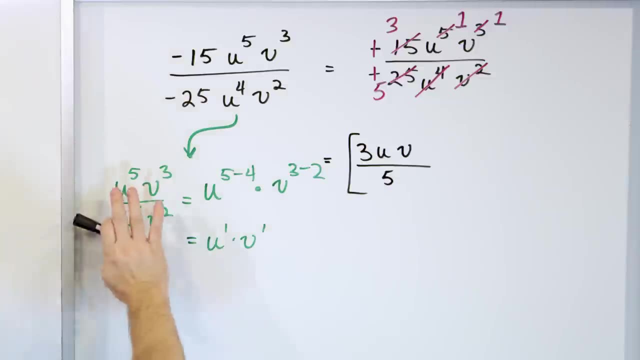 And, of course, what you get is u to the first times, v to the first, which is exactly what we got for our final answer: Different ways to think about it. It's okay to think about either way to do it. You can totally use this or you can do the cancellation method. I typically 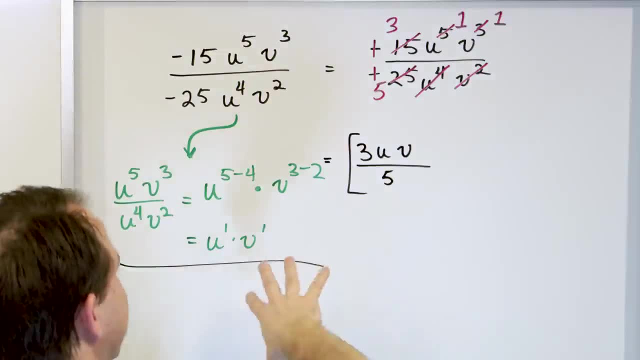 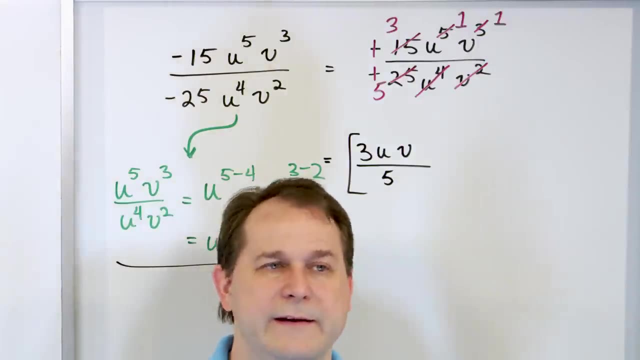 do the cancellation method. It becomes a little easier when the problems get harder, I think. in order to do that Also later on, I am going to introduce negative exponents, which it just depends on the problem. I don't know if that's the right answer, but typically I use this cancellation technique. 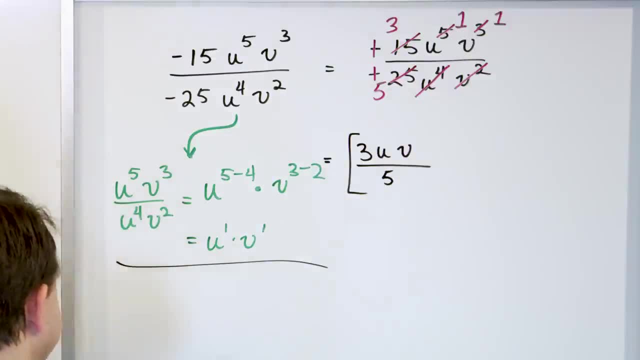 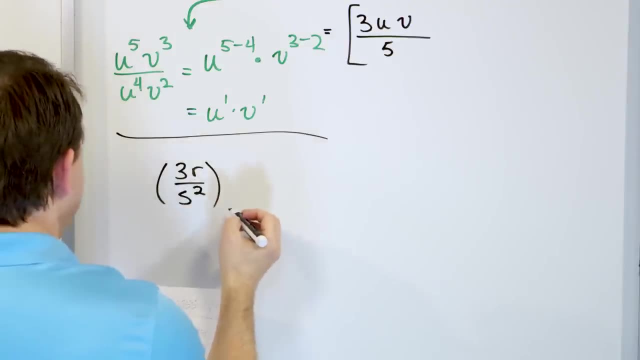 more than anything else. All right, Now let's move on to something a little different. What if we have three times r over s squared and that's a fraction all raised to the third power? All right Now. you look inside of here first and you try to simplify this, but you 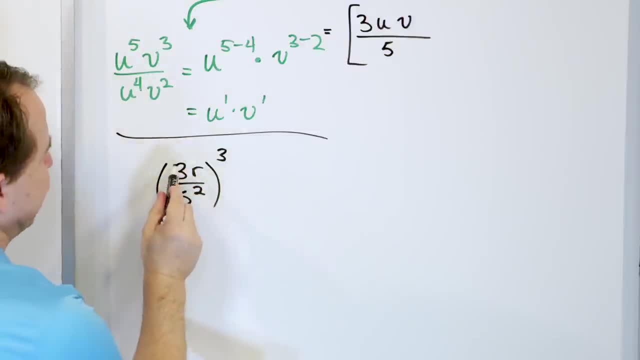 power. All right now you look inside of here first and you try to simplify this, but you can't, because three and one you can't do anything with, R and s squared you can't do anything with. So you go back to your exponent laws, right? 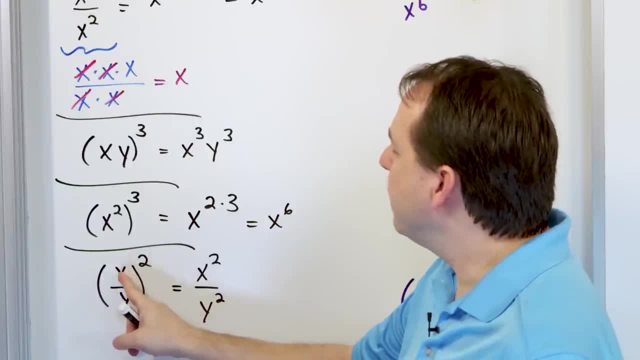 When you have a fraction of any kind with an exponent on the outside, you apply the exponent to the top and then the exponent to the bottom. So the way we're going to write that and make it clean is we're going to apply this to the. 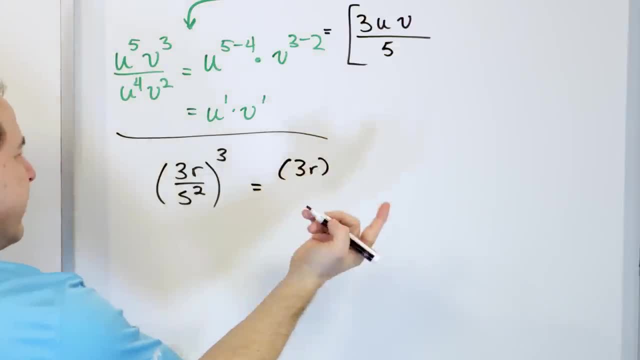 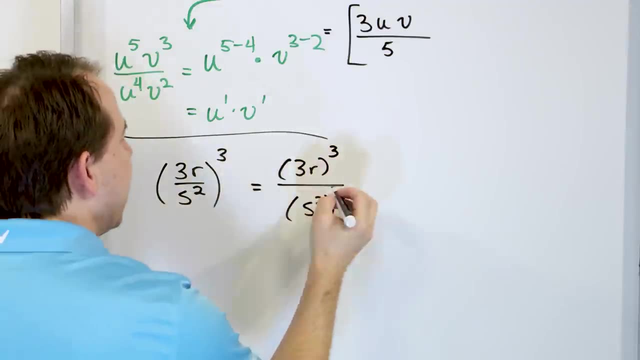 numerator. But the numerator is a complex thing with three r. We're going to raise that to the third power and then we're going to apply that to what we have here. S squared is the denominator, which has to be raised to the third power. 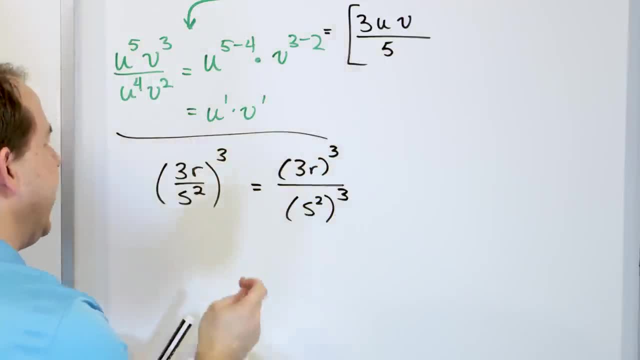 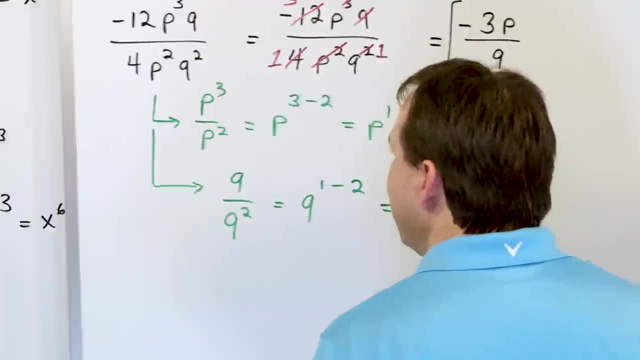 So you see, you're taking and applying it to the numerator, Which is a complex thing, and then you apply it to the denominator, which is kind of a complex thing too. But notice, the numerator is two things multiplied together, and we have a rule for that. 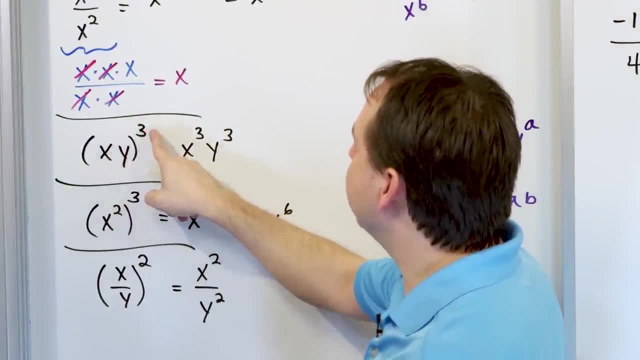 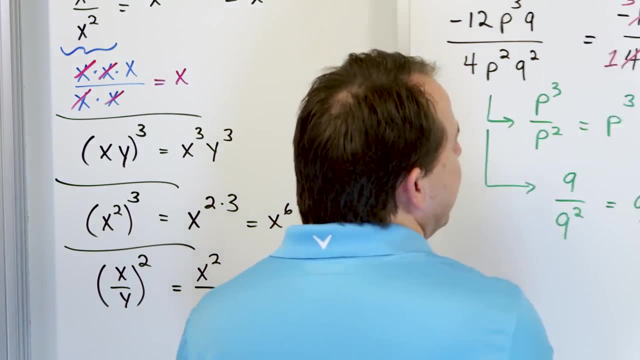 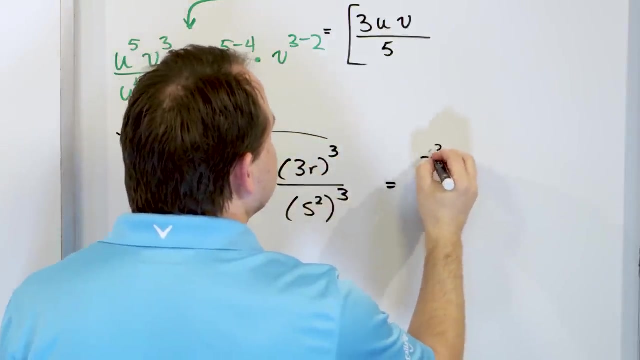 When we have two things multiplied together to an exponent, you apply the exponent to each one, And also an exponent raised to an exponent means you multiply the exponents. So now we have to apply both of those rules here. So right now the three would get applied to the three, making it three cubed. 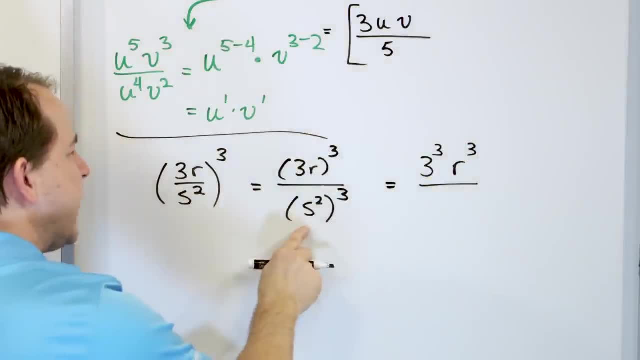 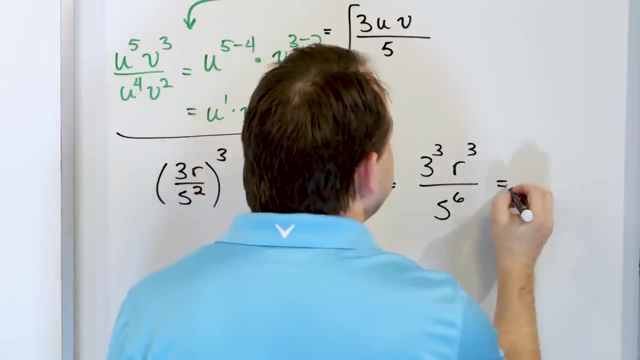 The r would get that exponent applied to the third power. The exponent applied as well, But on the bottom it's an exponent raised to an exponent. So it's two times three is six, And then finally, what is three, to the third power. 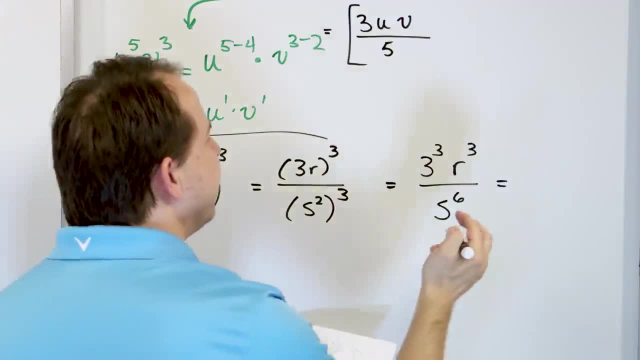 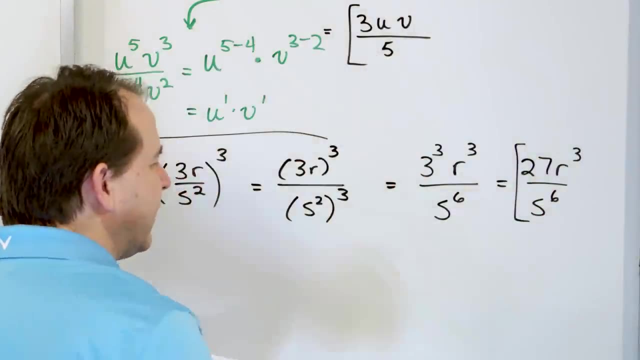 Three times three times three. So three times three is nine. Nine times three is twenty-seven. R cubed over s to the sixth, And I know you might want to do more with this because you don't like all those exponents. 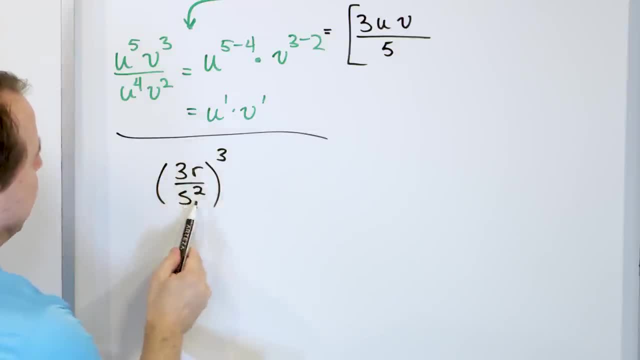 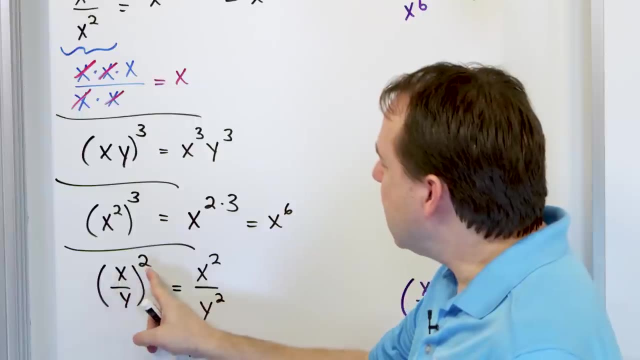 can't, because three and one you can't do anything with. r and s squared you can't do anything with. So you go back to your exponent laws. right, When you have a fraction of any exponent on the outside, you apply the exponent to the top and then the exponent to the bottom. 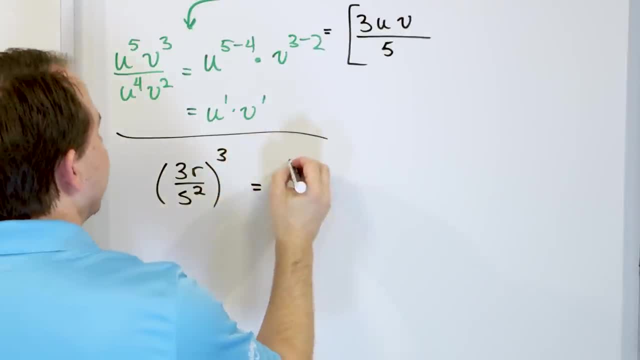 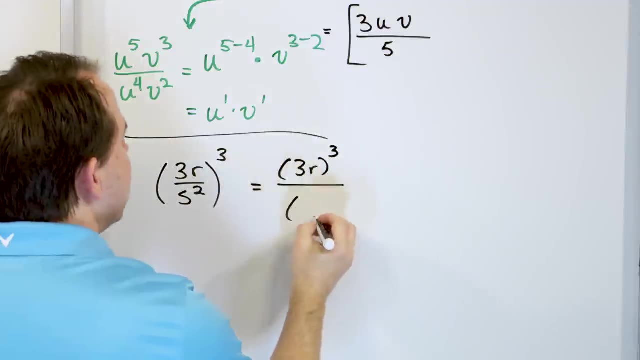 So the way we're going to write that and make it clean is: we're going to apply this to the numerator, but the numerator is a complex thing with three r. We're going to raise that to the third power and then we're going to apply that to what we have here: S squared. 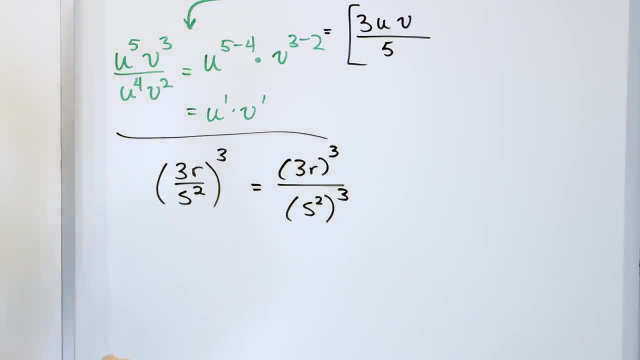 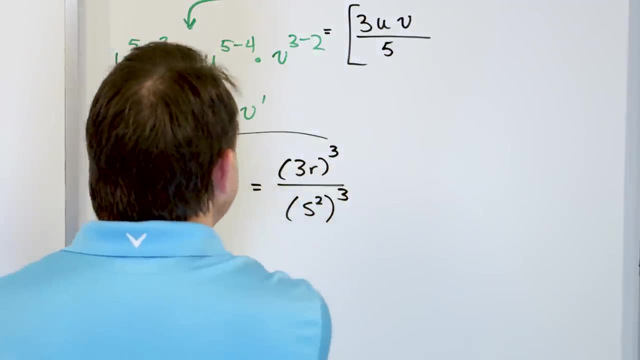 is the denominator which has to be raised to the third power. So you see, you're taking and applying it to the numerator, which is a complex thing, and then you apply it to the denominator, which is kind of a complex thing too. But notice, the numerator is going. 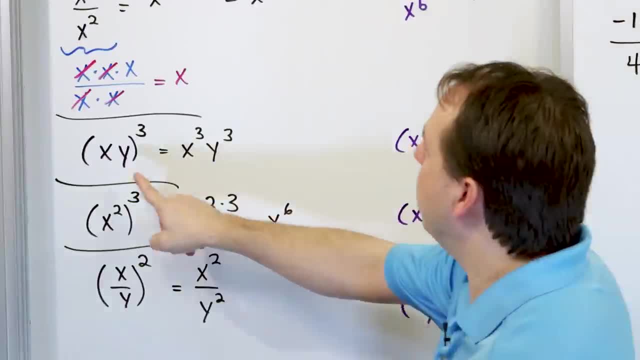 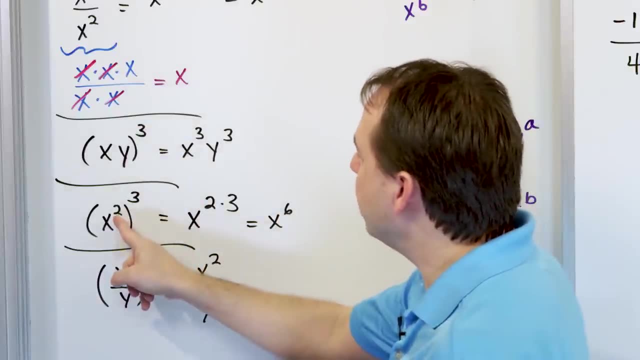 to be just two things multiplied together, And we have a rule for that: When we have two things multiplied together to an exponent, you apply the exponent to each one, And also an exponent raised to an exponent means you multiply the exponents. So now we have to. 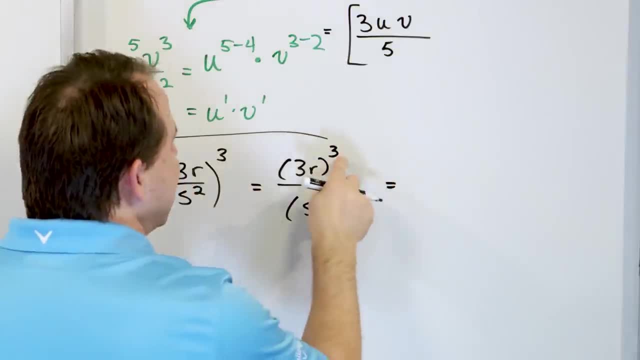 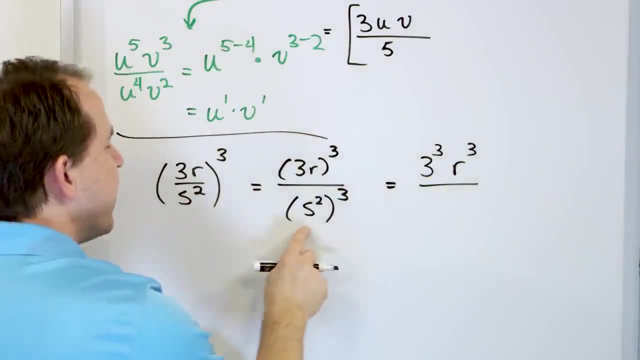 apply both of those rules here. So right now the three will get applied to the three, making it 3 cubed The r will get that exponent applied as well, but on the bottom it's an exponent raised to an exponent. So it's two times three is six. 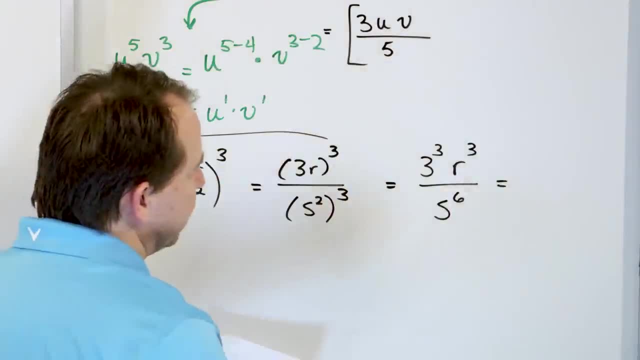 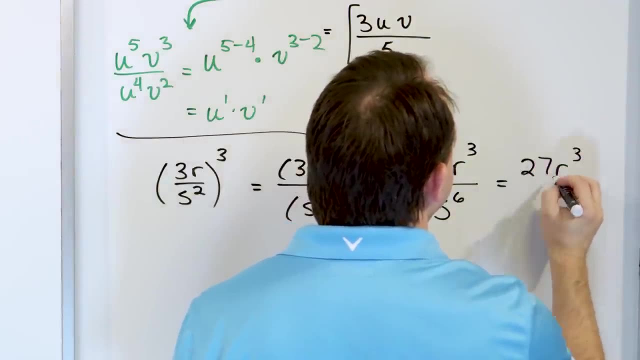 All right. And then finally, what is 3 to the third power? 3 times 3 times 3.. So 3 times 3 is 9.. 9 times 3 is 27.. r cubed over s to the 6th And I know you might want to do more with this. 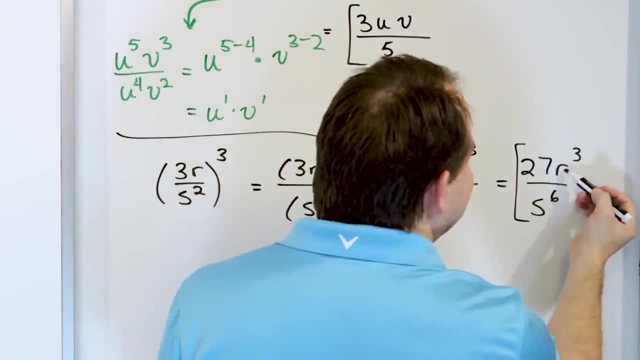 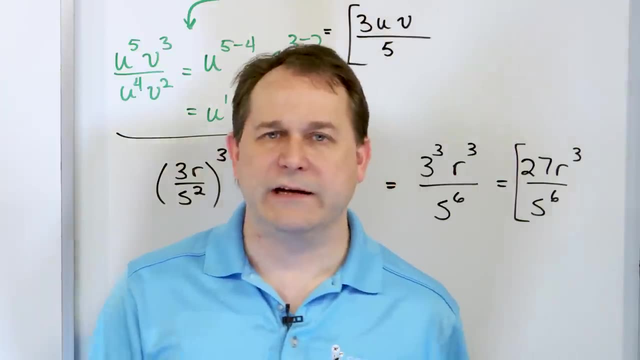 because you don't like all those exponents. but you can't because this is a different base than this one. You see, all of these exponent laws, they only apply if the base is the same. It's like peanut butter and jelly. You know, I know peanut butter and jelly, they go in a sandwich. 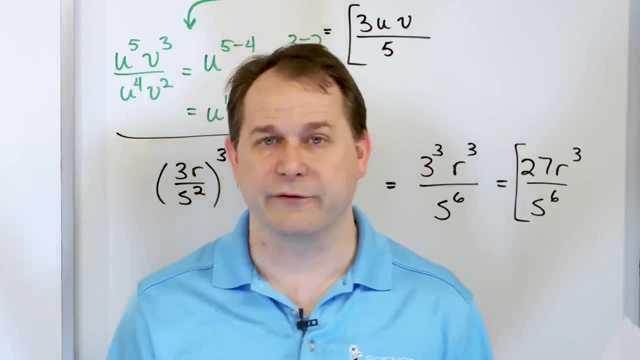 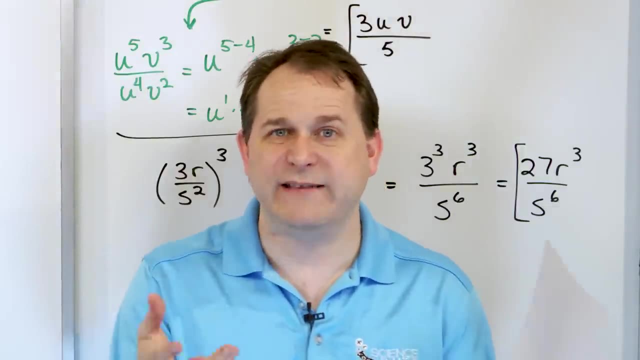 together and we love to eat peanut butter and jelly or ham and cheese or something right, They go together. But in algebra things can really only be worked on together or combined if they really are identical in some sense. So the bases have to be the same in order to add. 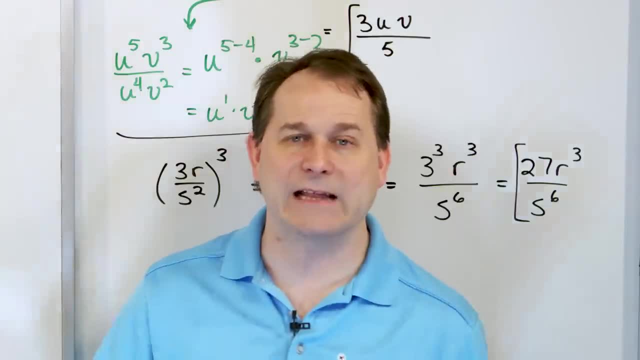 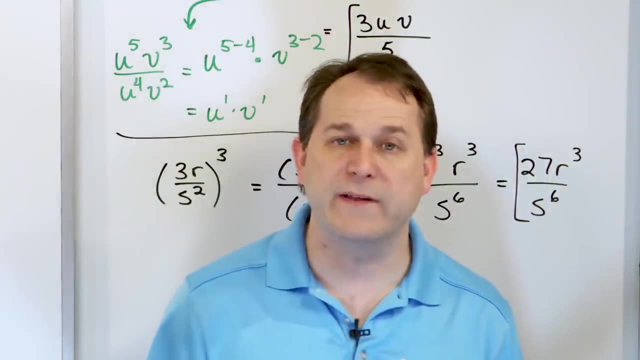 these exponents, or subtract the exponents, or even when we do other things like adding like terms, everything has to be the same right. So here we have an r cubed and an s to the 6th. Sorry, we just can't do anything with it, because these are completely different items. You can't just 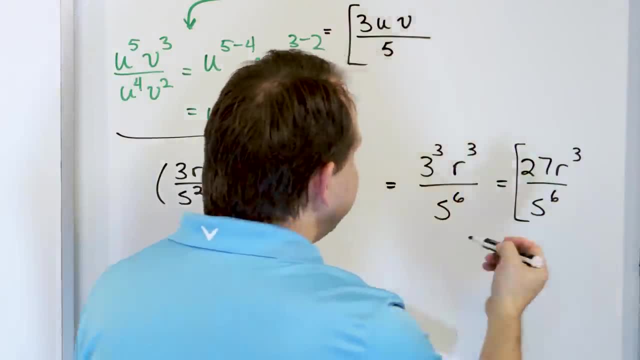 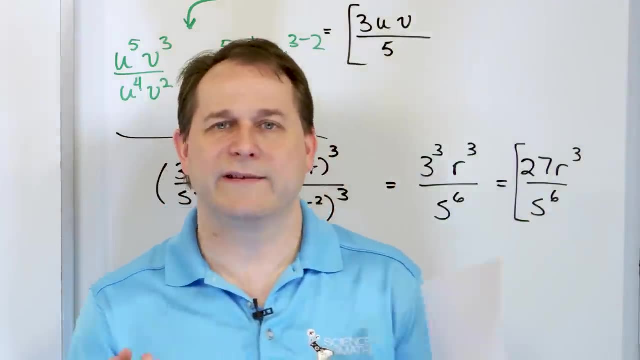 but you can't, Because this is a different base than this one. You see, all of these exponent laws, they only apply if the base is the same. It's like peanut butter and jelly. You know, I know, peanut butter and jelly, they go in a sandwich together. 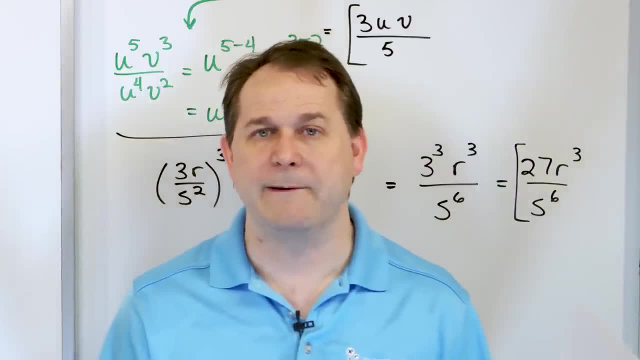 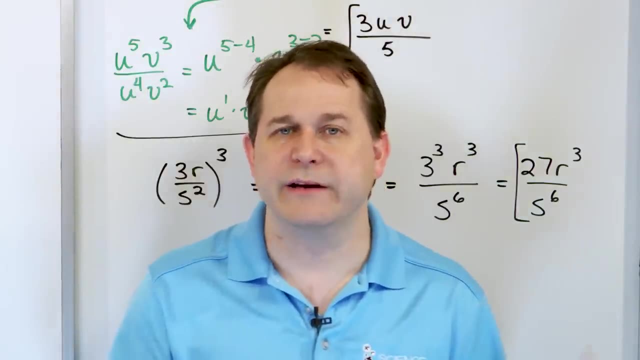 We love to eat peanut butter and jelly or ham and cheese or something right. They go together. But in algebra things can really only be worked on together or combined if they really are identical in some sense, So the bases have to be the same in order to add these exponents or subtract the exponents. 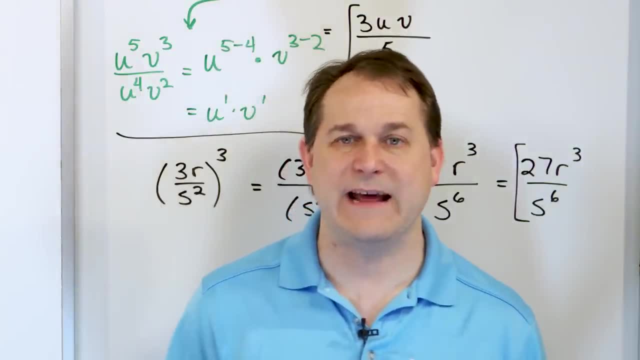 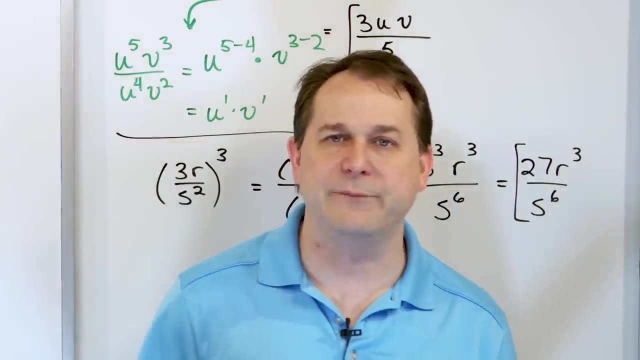 or even when we do other things like adding like terms, Everything has to be the same right. So here we have an r cubed and an s to the sixth. Sorry, we just can't do anything with it Because these are completely different items. 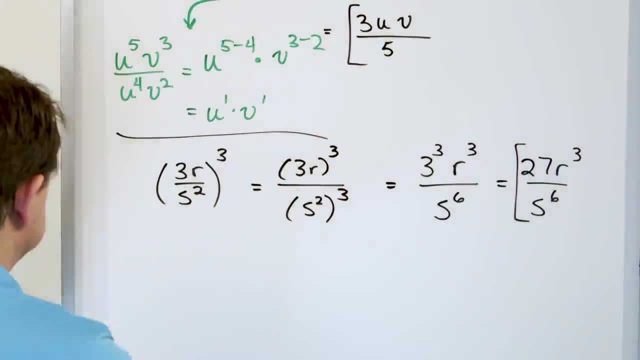 You can't just combine them together, So we leave it like this. all right, The next one we'll do is similar to this one. It's actually a little bit easier, But let's say we have 3s over t squared. 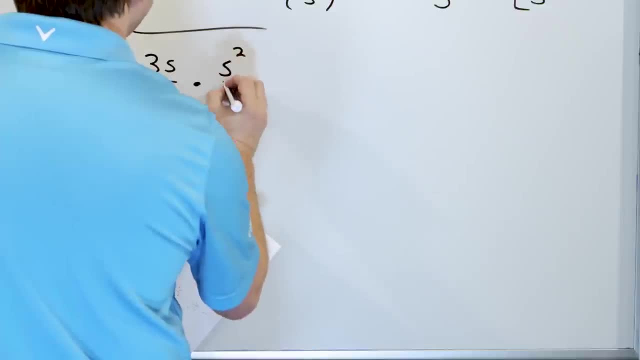 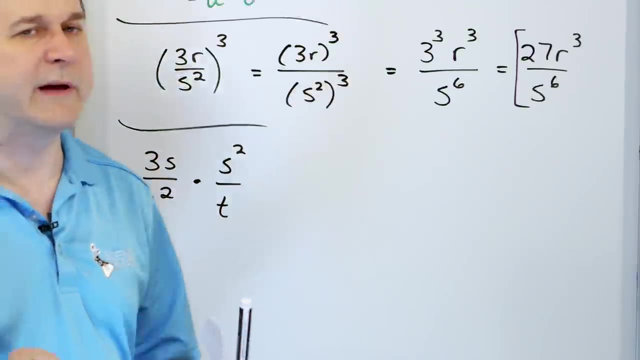 That's a fraction And we're going to multiply it by another fraction, which is going to be s squared over t. So when you look at this, when you first look at this, it can look a little intimidating, right? None of us, when we first learn fractions, really love fractions, right? 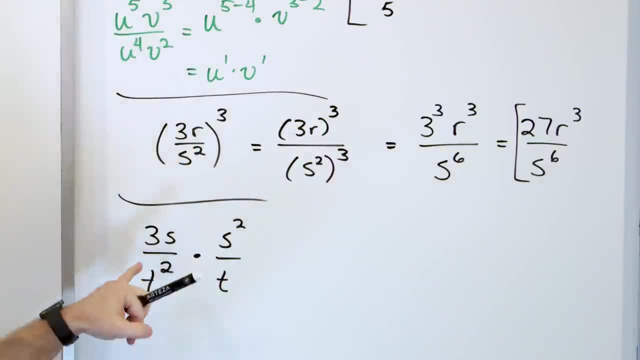 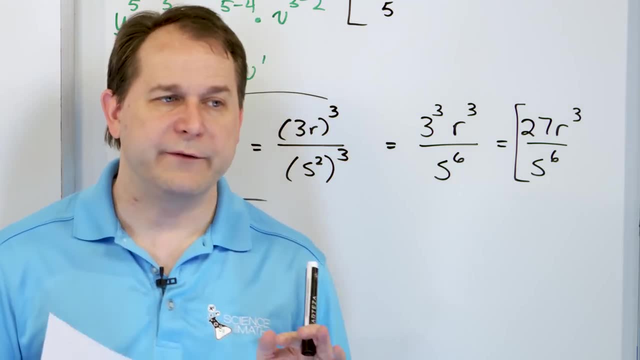 But you kind of get used to it and you can handle it. Then you start dealing with fractions that have terms on top exponents, on bottom exponents. on top It looks very difficult. My advice to you is: forget about the fact that it's a fraction in algebra. 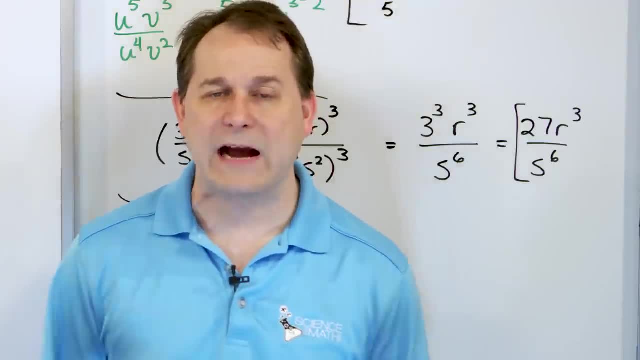 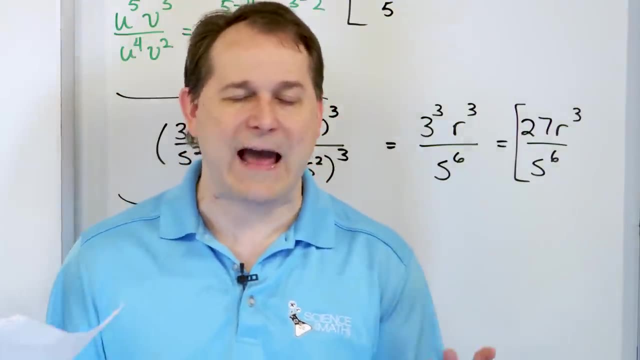 Forget about the fact that it looks complicated. The exact same rules of fractions apply to algebraic fractions as apply to any other fraction. In other words, to add any two fractions, you have to have a common denominator. Same thing is true. You have to have the same thing on the bottom. 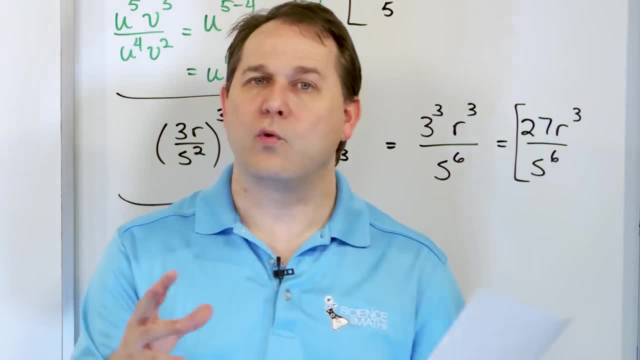 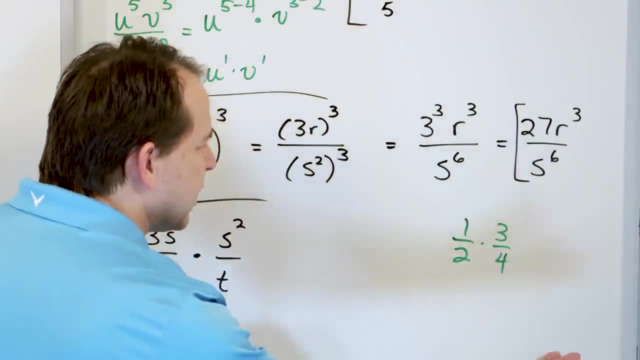 When you multiply fractions, no matter if it's a number fraction or an algebra fraction. remember what happens if we have something like 1 half times 3 fourths. How do we do it? We don't get a common denominator for this. 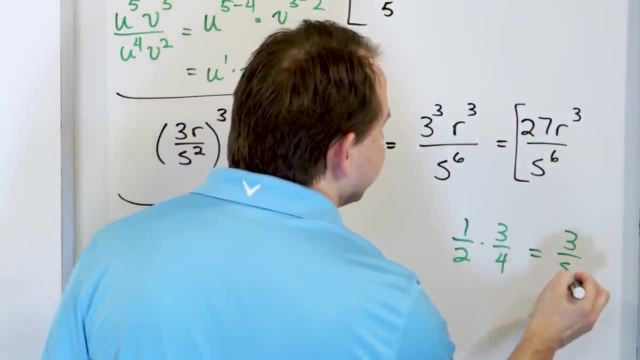 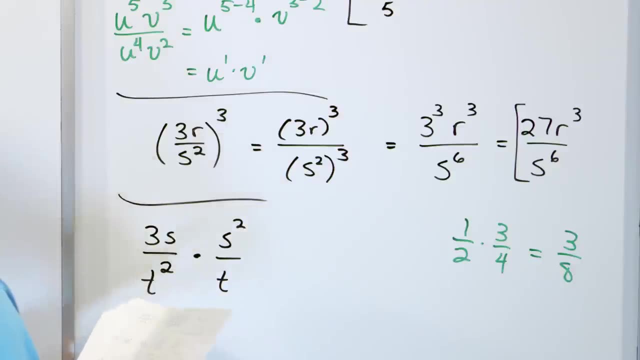 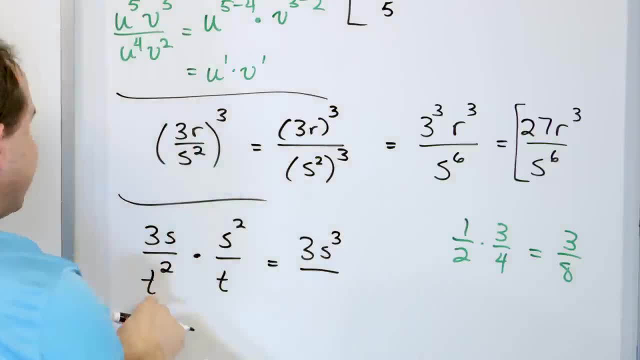 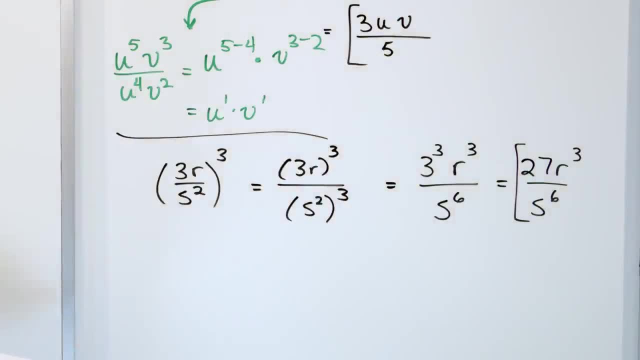 combine them together. So we leave it like this. All right, The next one we'll do is similar to this one. It's actually a little bit easier. but let's say we have 3s over t squared. That's a fraction, and we're. 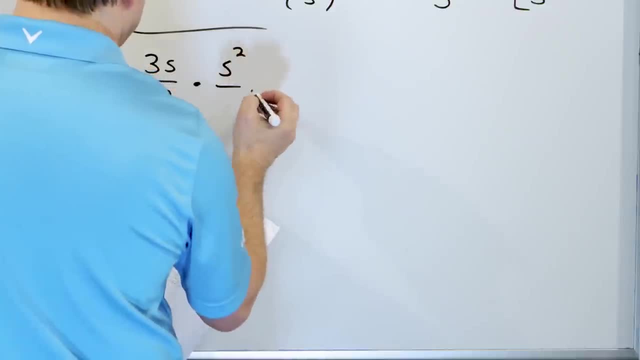 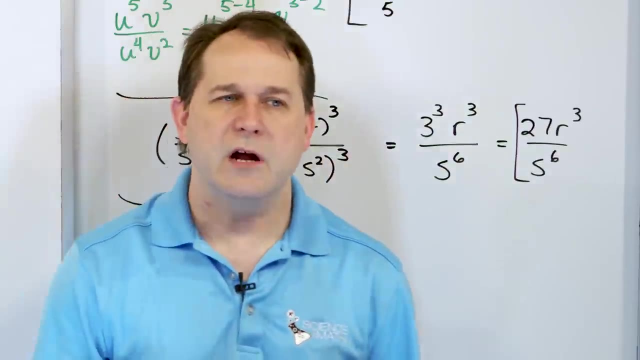 going to multiply it by another fraction, which is going to be s squared over t. So when you look at this, when you first look at this, it can look a little intimidating, right? Because none of us, when we first learn fractions, really love fractions, right? 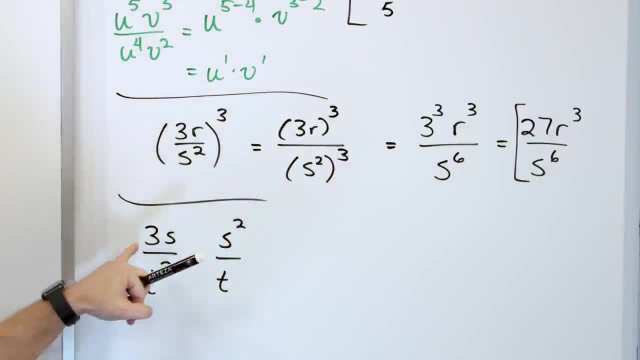 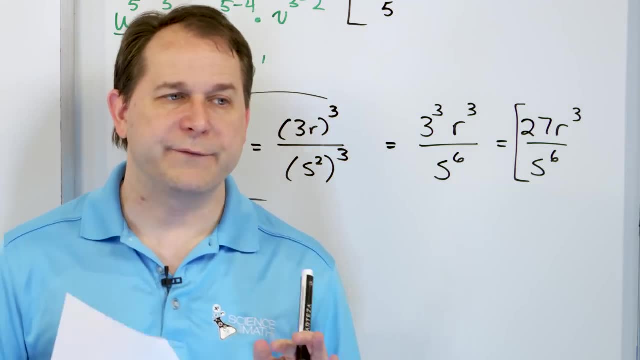 You kind of get used to it and you can handle it. And then you start dealing with fractions that have terms on top exponents, on bottom exponents. on top It looks very difficult. My advice to you is: forget about the fact that it's a fraction in algebra. Forget about the fact that it looks. 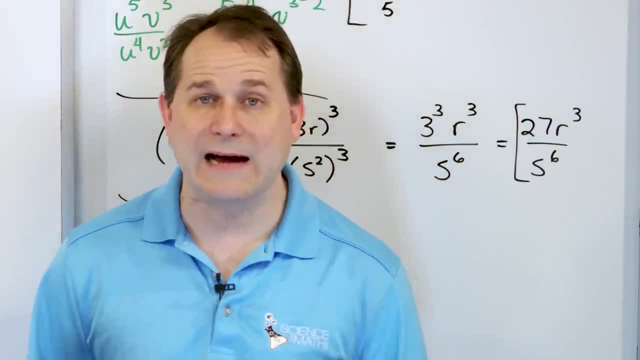 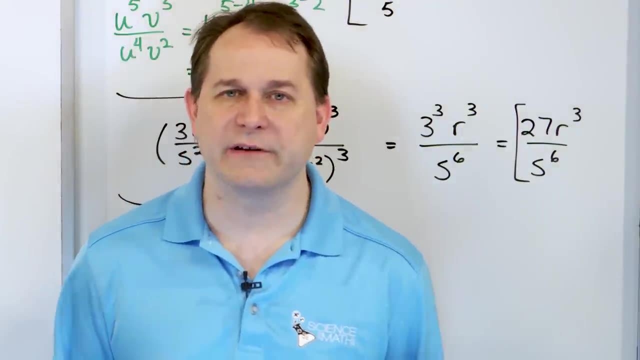 complicated. The exact same rules of fractions apply to algebraic fractions as apply to any other fraction. In other words, to add any two fractions, you have to have a common denominator. Same thing is true if it's an algebra fraction. You have to have the same thing on the bottom. 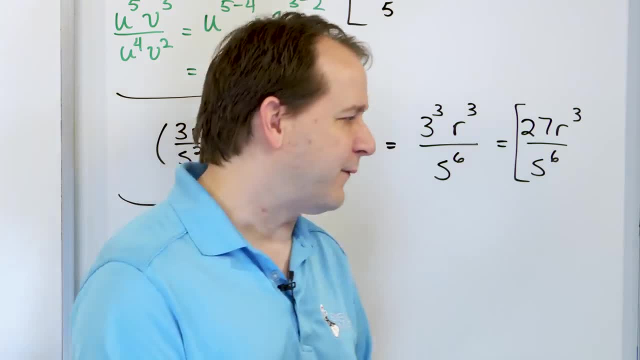 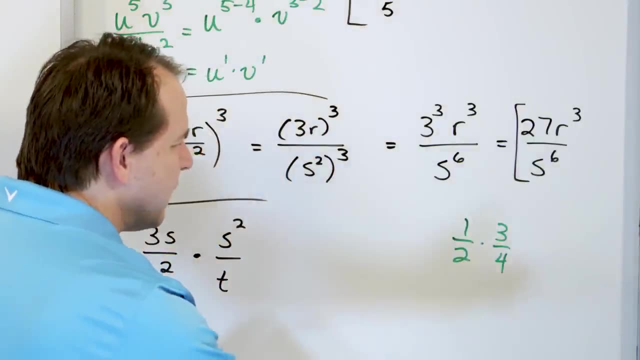 So we multiply fractions, No matter if it's a number fraction or an algebra fraction. remember what happens if we have something like 1 half times 3, fourths. How do we do it? We don't get a common denominator for this. We just multiply the tops, giving us 3, and we multiply the bottoms. 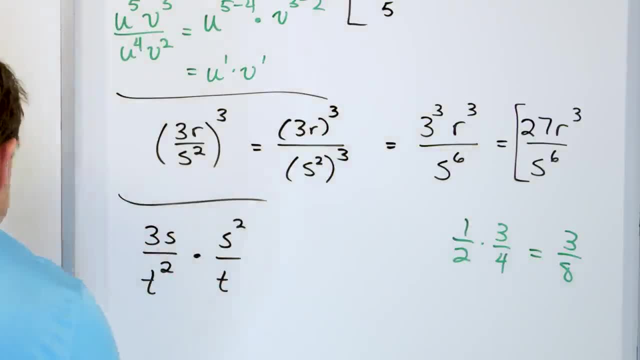 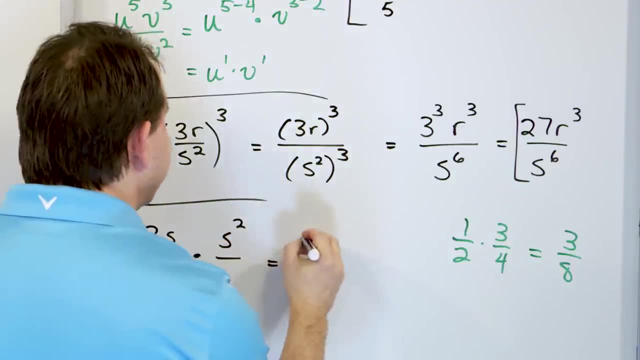 giving us 8. Multiply the tops, multiply the bottoms. So the exact same thing happens here: We multiply the tops and we multiply the bottoms. So when we multiply this together we get 3s. but we have to add these exponents because it'll be 3s. 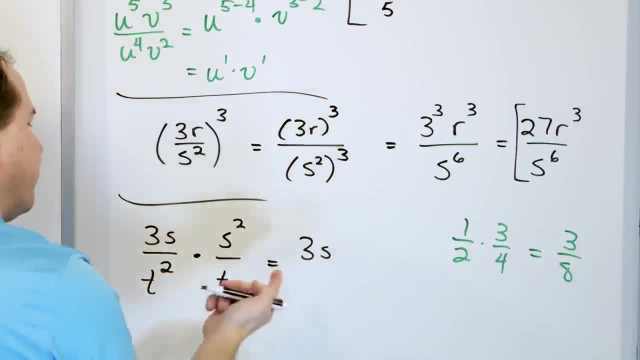 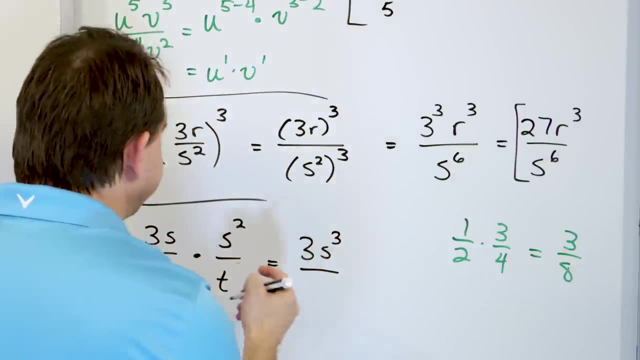 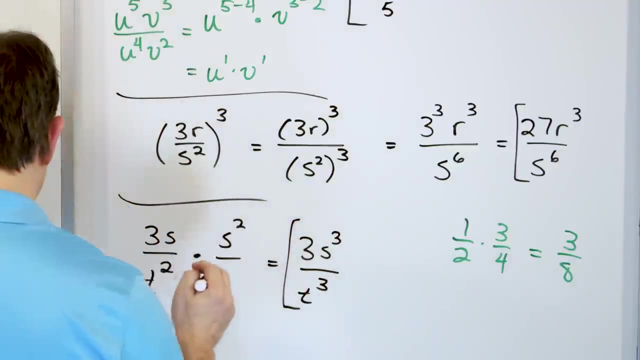 times s, So we can add those exponents, because we're multiplying the s terms together. So it'll be 3s cubed And then t squared times t is going to be adding those exponents. 2 plus 1 is 3. So we get t cubed right here. So we get 3s cubed over t cubed. So again, 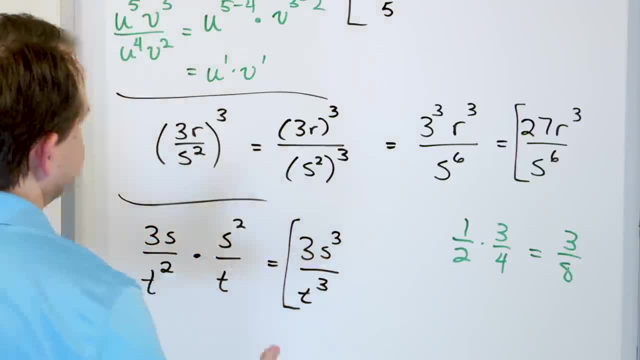 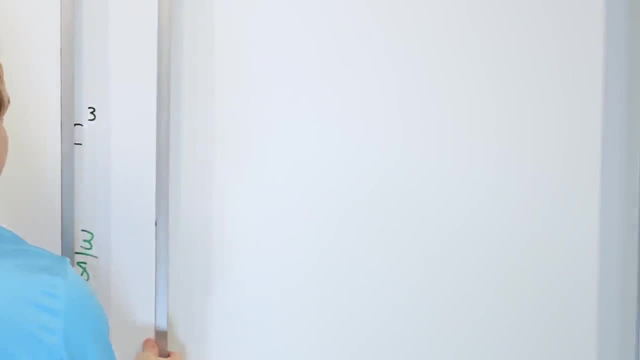 the final answer is: 3s cubed over t cubed. And as much as you want to combine these, you can't. You can't subtract exponents or anything, because these have different bases. So you can't, You can't combine them, They're different. All right, We have two more. They're not difficult. 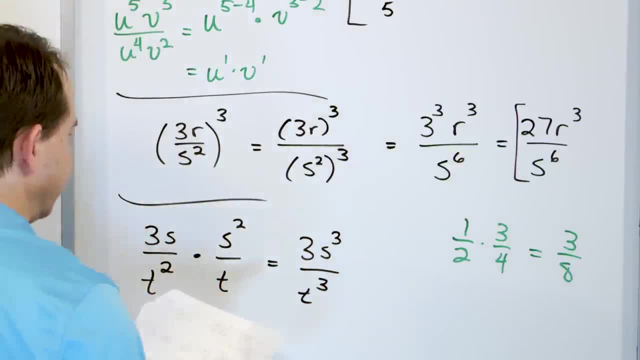 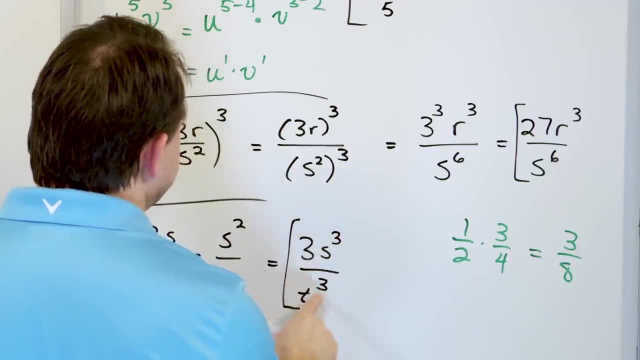 we get t cubed right here. So we get 3s cubed over t cubed. So again, the final answer is 3s cubed over t cubed. And as much as you want to combine these, you can't. You can't subtract exponents. 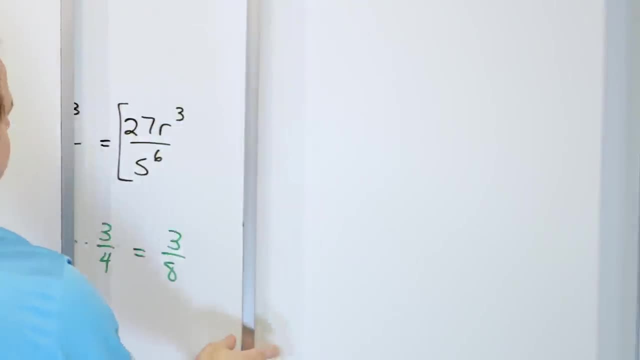 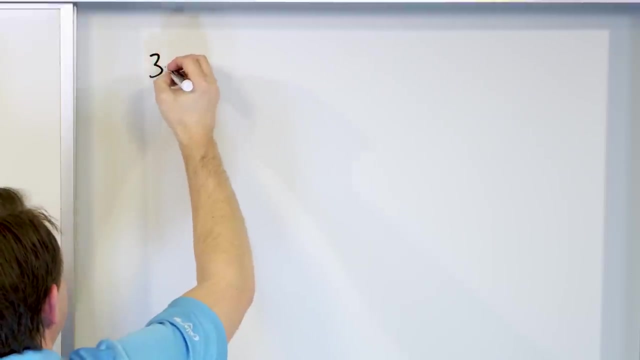 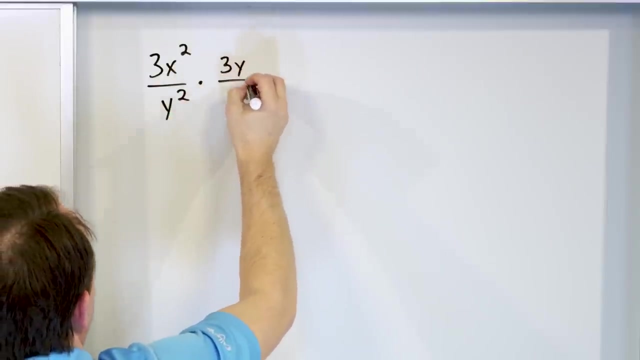 or anything, because these have different bases So you can't combine them. They're different. All right, We have two more. They're not difficult, but we want to get through these. What about 3x squared divided by y squared times 3y over 6x? All right, So it's the same kind of. 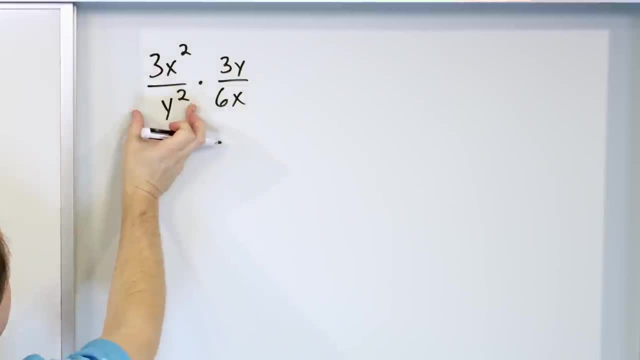 thing, We have to treat them as fractions. This is a fraction. Yes, it's ugly. I understand that This is a fraction. Yes, I understand that it's ugly, But it's a fraction nonetheless. So we multiply them. We treat them the same way as everything else. 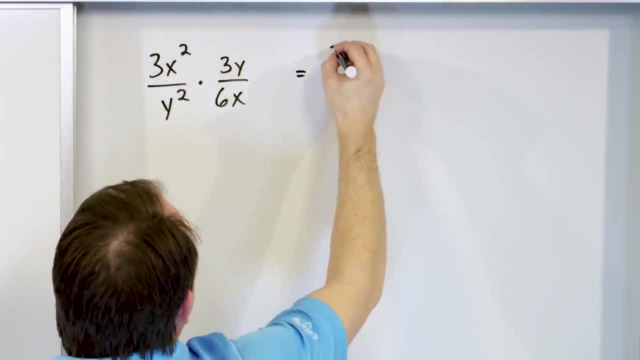 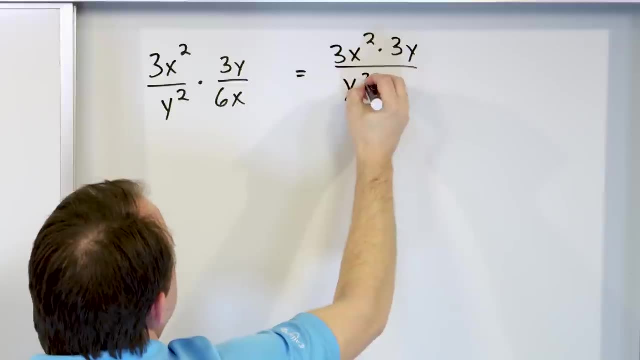 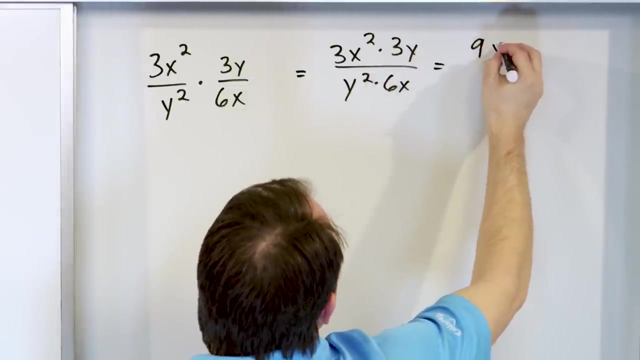 So what we have is multiplying the tops together: 3x squared times 3y. right, And on the bottom we have this y squared times 6x. So we just handle the multiplication. Now we can always multiply the numbers together. That gives us 9.. We'll have x squared y And on the bottom, 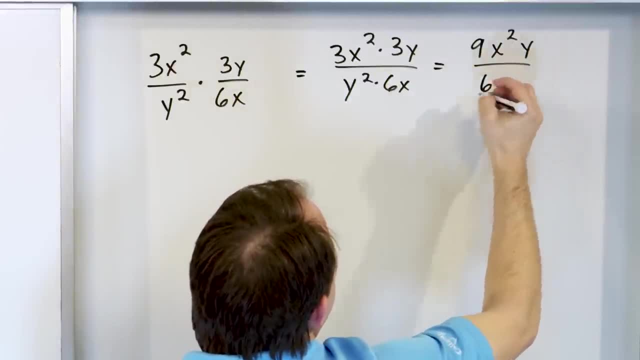 we'll have a y squared with a 6 in the front, So we'll have a 6.. Let's write it as x first and then y squared. Now you see, this kind of problem looks exactly like some of the other problems. 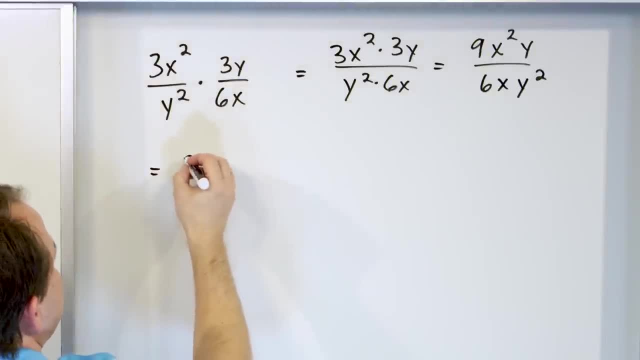 The earlier problems we have. So we need to simplify that. Let me go ahead and write it again: 9x squared y, And then we'll have 6xy squared. So again we try to simplify. We'll divide top and bottom by 3.. So 6 divided by 3 is 3.. 9 divided by 3 is: I'm sorry, 6 divided by 3 is: 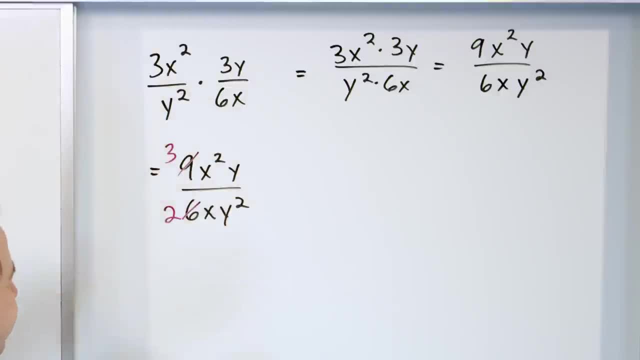 2. And 9 divided by 3 is 3.. And then for the exponents we have 1x and 2x. So this entire x cancels with one of these. So we're leaving one left. 1y on the top cancels. So we scratch that out And we have only one left. 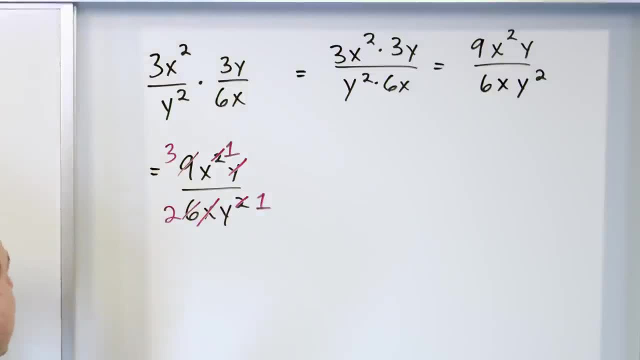 because we had 2. And now we have only 1.. So then we can write the final answer as on the top we have a 3x And on the bottom we have a 2 times y. Everything else is gone. The y is gone. 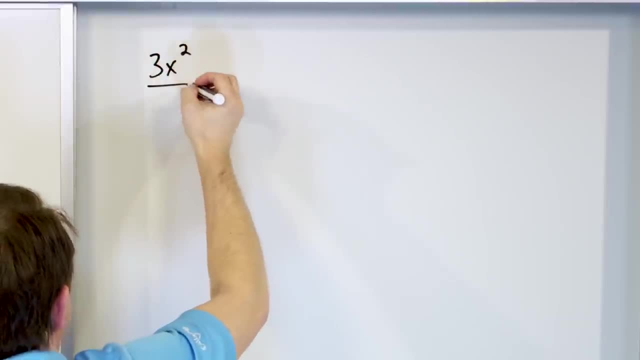 but we want to get through these. What about 3x squared divided by y? squared times 3y over 6x? All right, So it's the same kind of thing. We have to treat them as fractions. This is a fraction. Yes, it's ugly. I understand that This is a fraction. Yes, I understand. 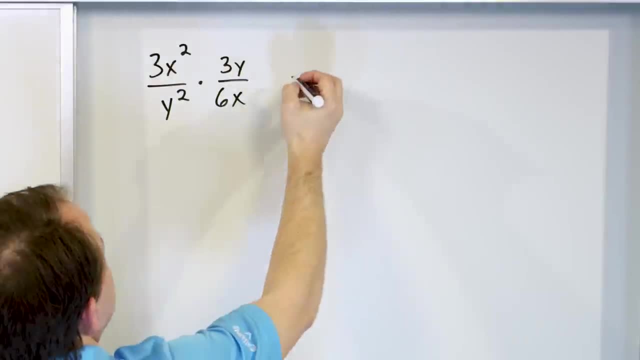 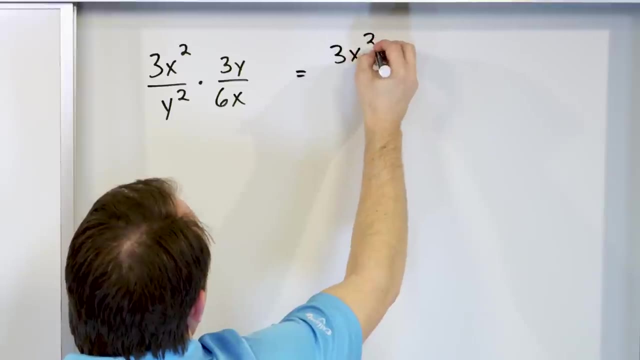 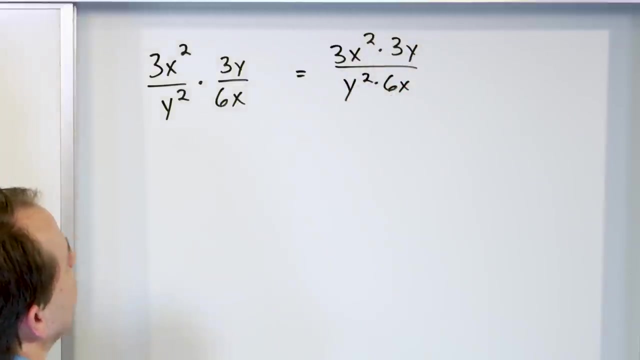 that it's ugly, But it's a fraction nonetheless. So when we multiply them, we treat them the same way as everything else. So what we have is multiplying the tops together, 3x squared times 3y right, And on the bottom we have this y squared times 6x. So we just handle. 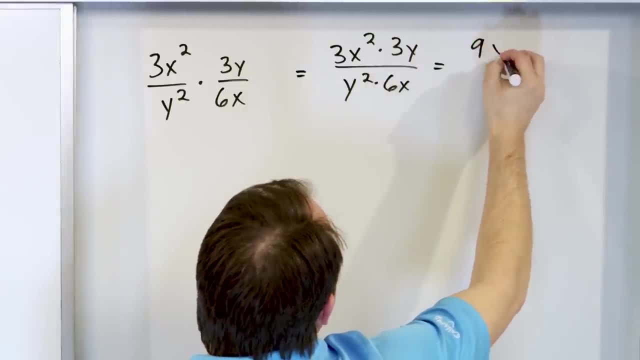 the multiplication. Now we can always multiply the numbers together. that gives us 9.. We'll have x squared y, And on the bottom we'll have a y squared with a six in the front, So we'll have a six. 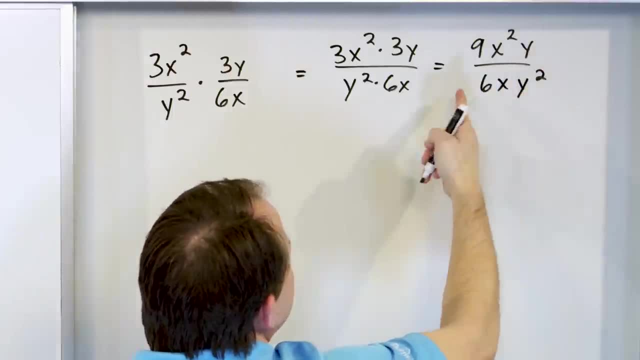 let's write it as x first And then y squared: 00,000,000,000 favor: 00,000,000,000. Noram Hare Looks exactly like some of the earlier problems we have, So we need to simplify that. 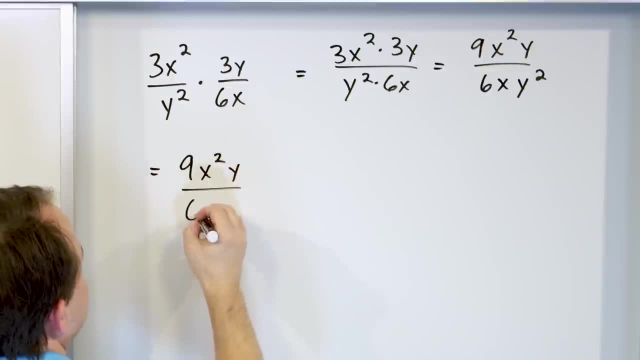 Let me go ahead and write it again: 9x squared y, and then we'll have 6xy squared. So again, we try to simplify. We'll divide top and bottom by 3.. So 6 divided by 3 is 3.. 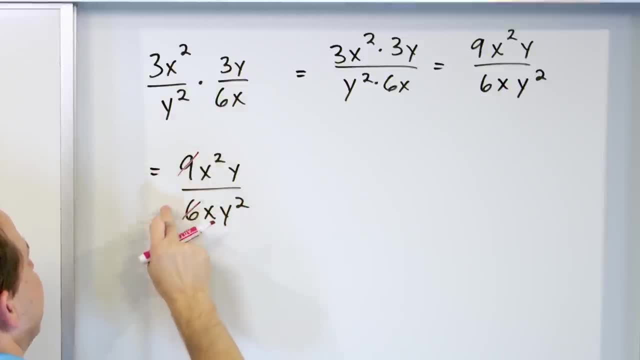 9 divided by 3 is- I'm sorry- 6 divided by 3 is 2.. And 9 divided by 3 is 3.. And then for the exponents we have 1x and 2x. So this entire x cancels with one of these, leaving one left. 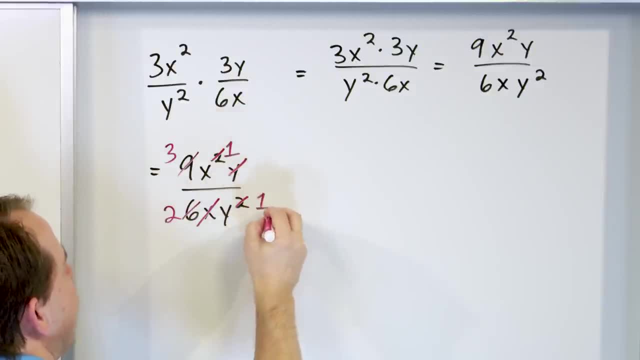 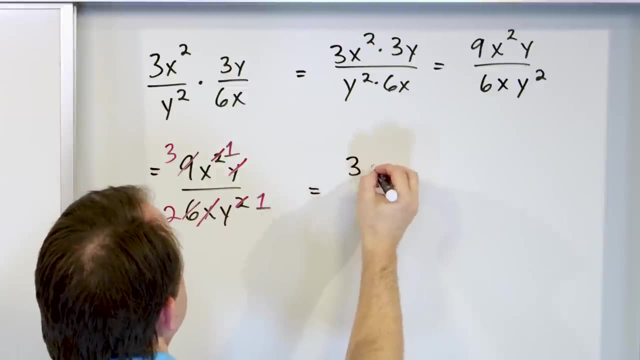 One y on the top cancels, so we scratch that out and we have only one left, because we had 2, and now we have only 1.. So then we can write the final answer as on the top we have a 3x. 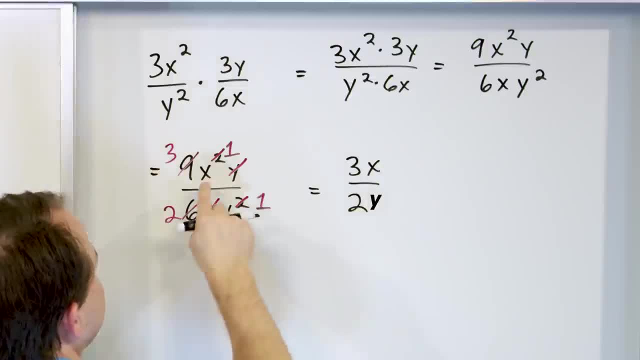 and on the bottom we have a 2 times y. Everything else is gone, The y is gone, and so on, so we have 3x over 2y. That's the final answer. Now, always in my algebra there's always multiple ways to do things. 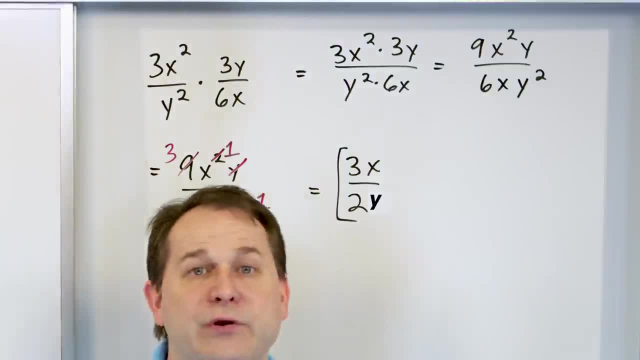 When you're looking at this, probably thinking of a slightly different way to do this. If you see a different way to do it, great, That's totally fine. There is probably three different ways I could do this problem, And none of them are right or more correct. 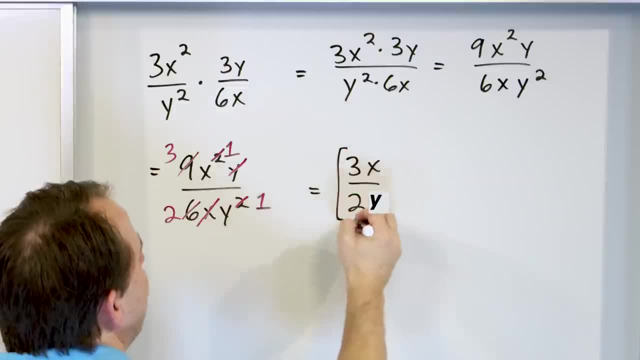 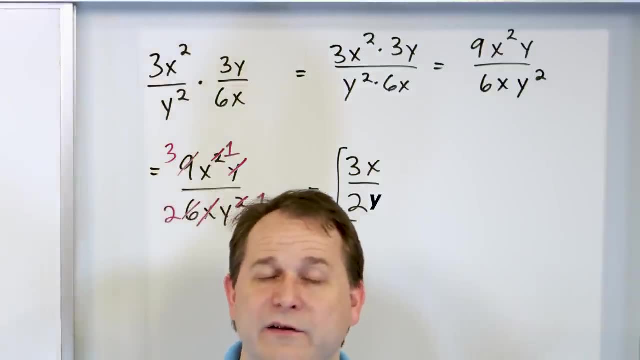 and so on. So we have 3x over 2y. That's the final answer. Now, always in my algebra, there's always multiple ways to do things. When you're looking at this, probably thinking of a slightly different way to do this. If you see a different way to do it, great, That's totally fine. 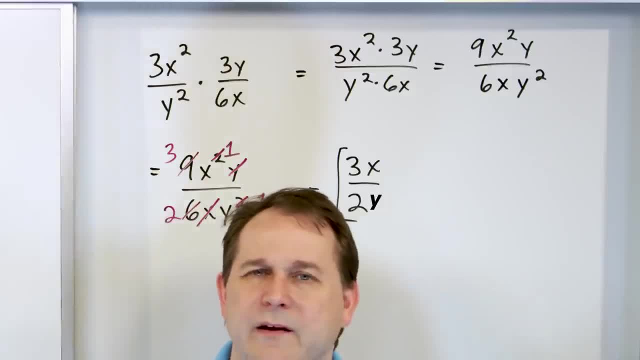 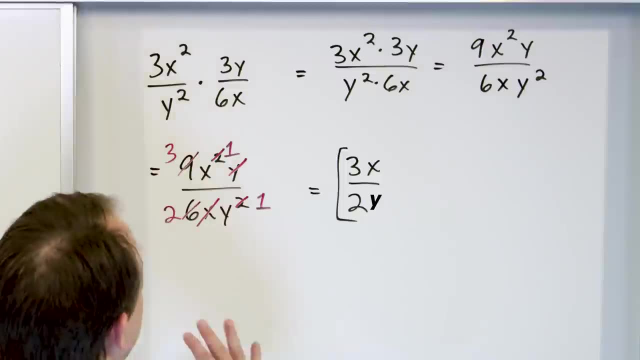 There's probably three different ways I could do this problem, And none of them are right or more correct. It's just different ways of doing it. Let me give you a couple. I'm not going to solve it again, but let me do another example of how it could be different or how you could think of it. 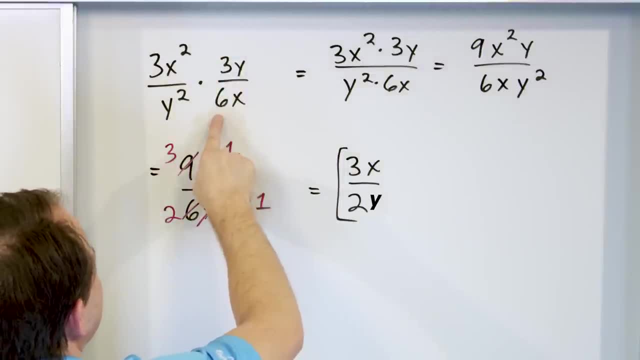 differently Right away. you see, this is 3 divided by 6.. So immediately before doing anything else, I could just simplify this fraction and make this 1 half, So it would be y over 2x. So if I simplified this, the 3 would go away, The 2 would be on the bottom. Notice we have a 3 and a 2.. So 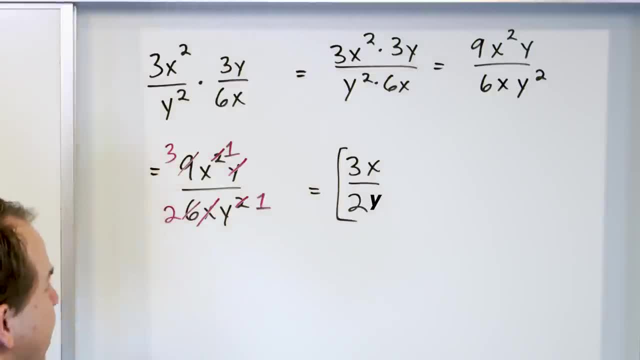 the numbers would triple or would ripple. Remember exactly as we got to this final answer here. Here in this step, we multiplied the tops, multiplied the bottoms, then simplified. But we could simplify the numbers first and we'll get exactly the same answer. Also, many of you know, because we've done in previous 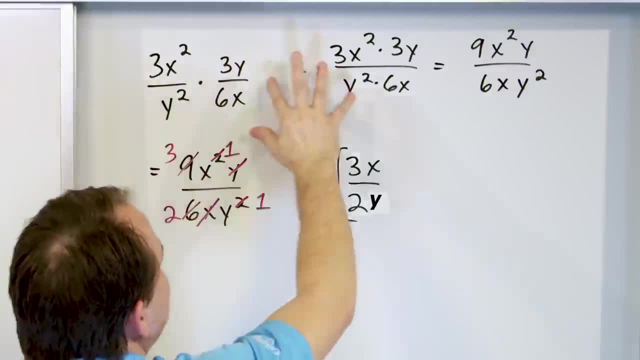 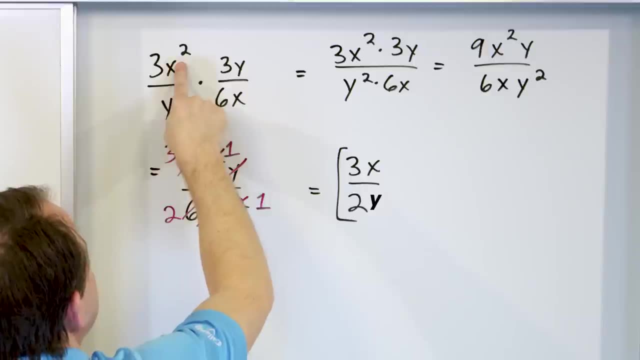 problems that we can simplify all of this if we want to. even before doing the multiplication, For instance, you know it's multiplied. So when you have a fraction times a fraction, if you have something in the top here, you can cancel with the bottom And you have something. 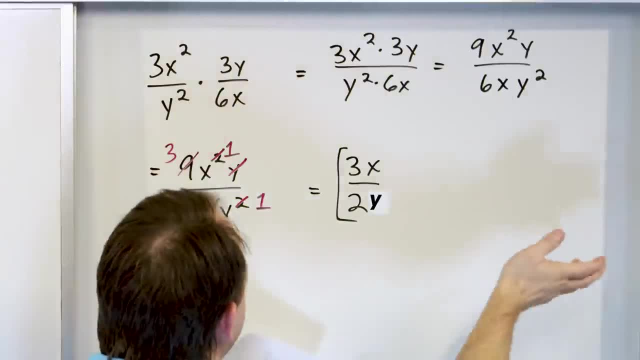 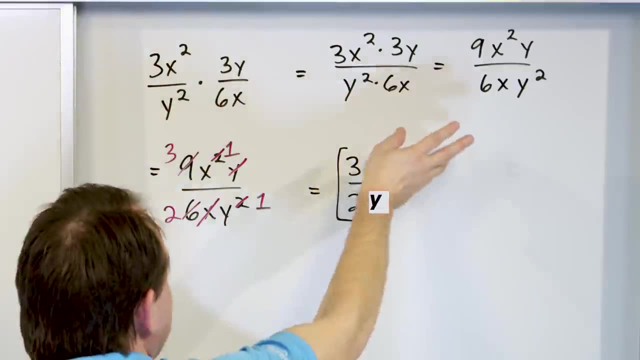 here you can cancel with the bottom And you have something here you can cancel with the bottom Because in the end you're going to multiply them all through anyway, on the tops and on the bottoms. So you can simplify before you multiply the fractions, or you can multiply first, like 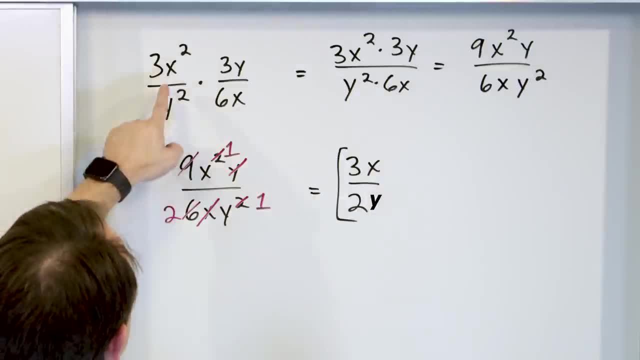 we've done here and then simplify at the end. So in other words, I could look at the x squared and the x and I could cancel the x here and cancel one of these x's straight away. I could cancel one of the y's straight away. I could simplify the numbers before I do any fraction. 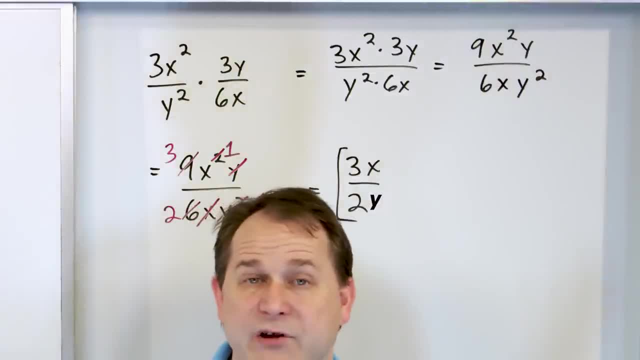 multiplication and then multiply the fractions, and I would get exactly what I've done here, which is doing all the multiplication first and then simplifying. Is there a right way? No, There's no right way, But there's different ways, and that's OK. As long as you know what the different ways are and what's legal, I'm happy. 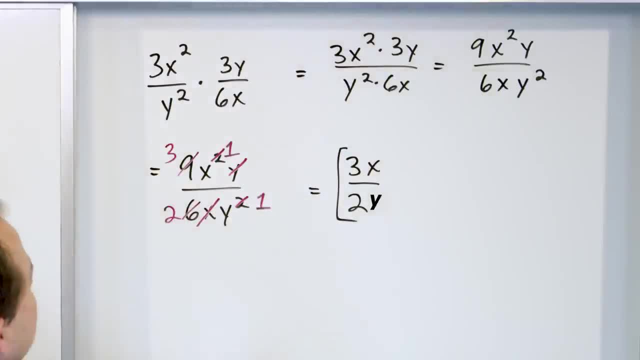 It's just different ways of doing it. Let me give you a couple. I'm not going to solve it again, but let me do another example of how it could be different or how you could think of it differently Right away. you see, this is 3 divided by 6.. 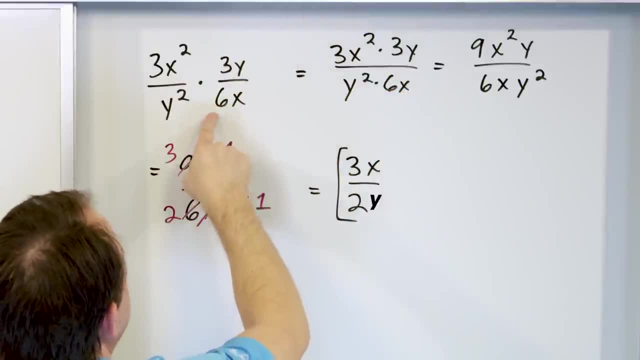 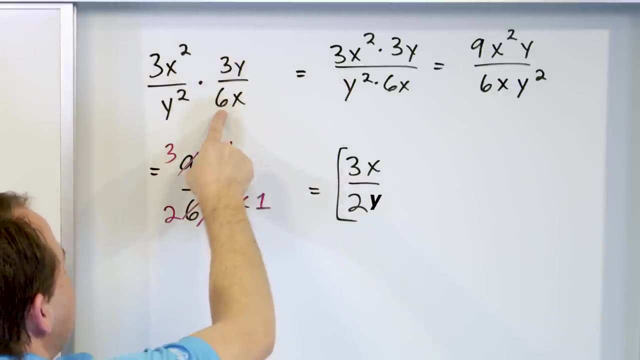 So, immediately before doing anything else, I could just simplify this fraction and make this 1 half, So it would be y over 2x, right? So if I simplified this, the 3 would go away, The 2 would be on the bottom. 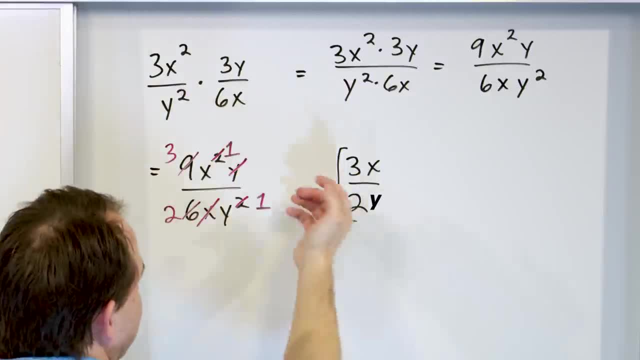 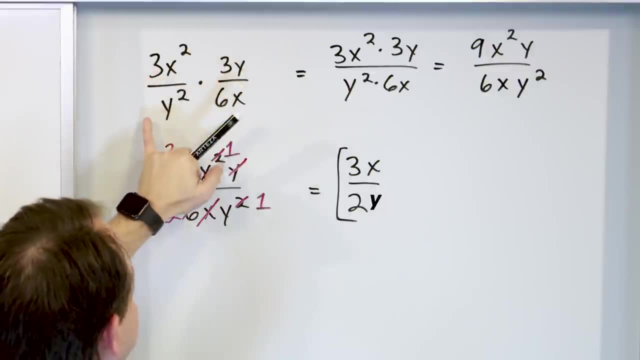 Notice, we have a 3 and a 2. So the numbers would triple or ripple through, exactly as we got to this final answer here. Here, in this step, we multiplied the tops, multiplied the bottoms, then simplified. But we could simplify the numbers first and we'll get exactly the same answer. 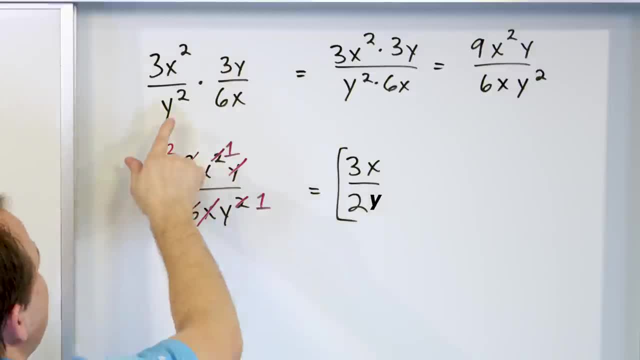 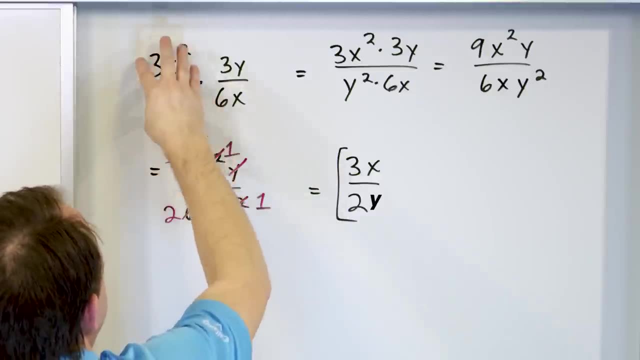 Also, many of you know, because we've done in previous problems, that we can simplify all of this if we want to. even before doing the multiplication, For instance, you know it's multiplied. So when you have a fraction times a fraction. 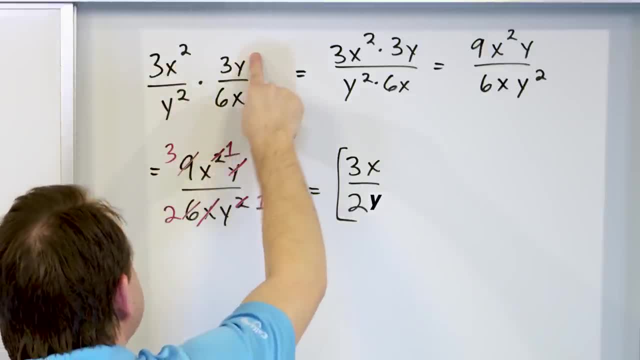 if you have something in the middle, on the top, here you can cancel with the bottom. And you have something here, you can cancel with the bottom here, Because in the end you're going to multiply them all through anyway, on the tops and on the bottom. 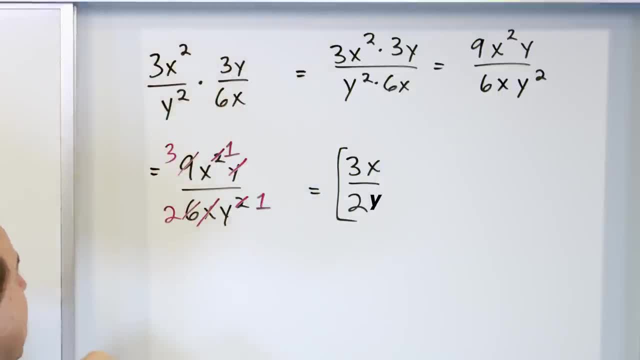 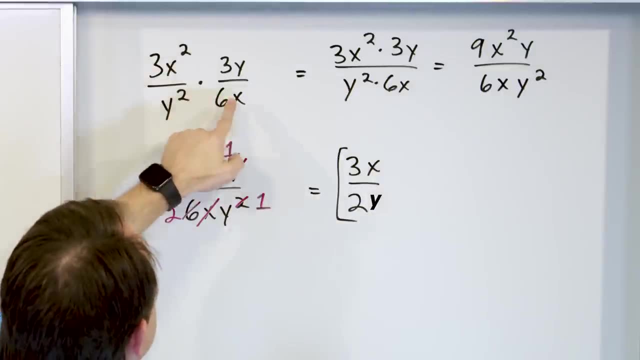 So you can simplify before you multiply the fractions, Or you can multiply first, like we've done here, and then simplify at the end. So in other words, I could look at the x squared and the x and I could cancel the x here and cancel one of these x's straight away. 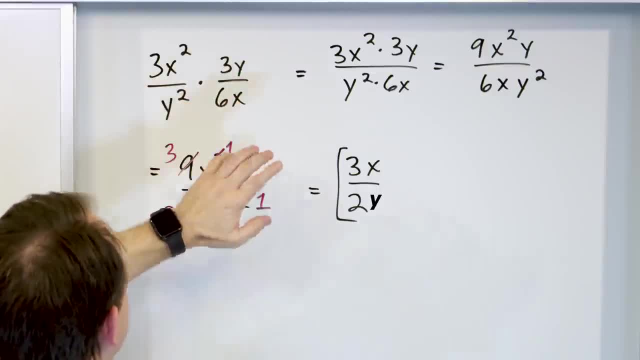 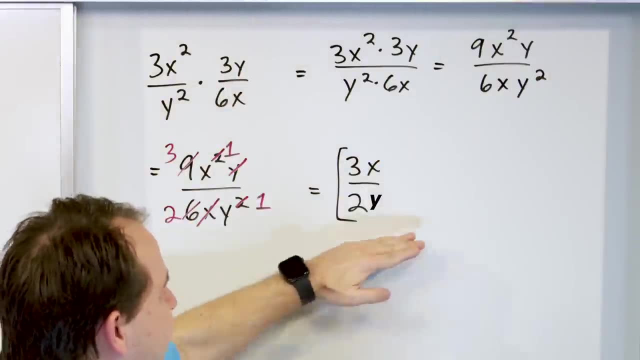 I could cancel one of the y's straight away. I could simplify the numbers before I do any fraction multiplication and then multiply the fractions, and I would get exactly what I've done here, which is doing all the multiplication first and then simplifying. Is there a right way? 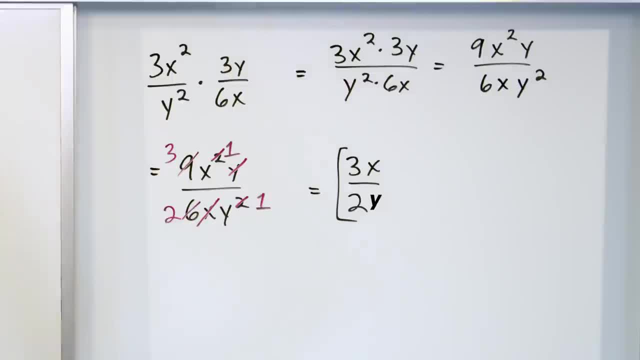 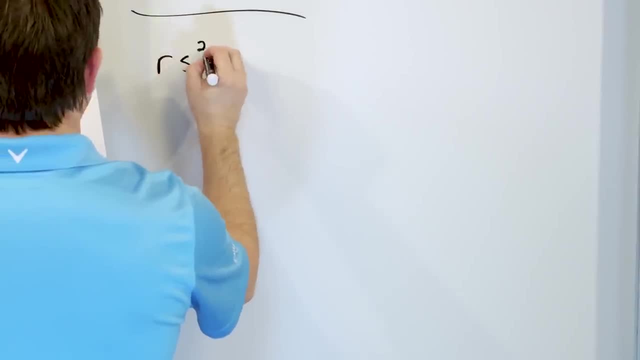 No, there's no right way, But there's different ways and that's okay. As long as you know what the different ways are and what's legal, I'm happy. Final problem: r times s squared times. t cubed over r cubed s squared t. 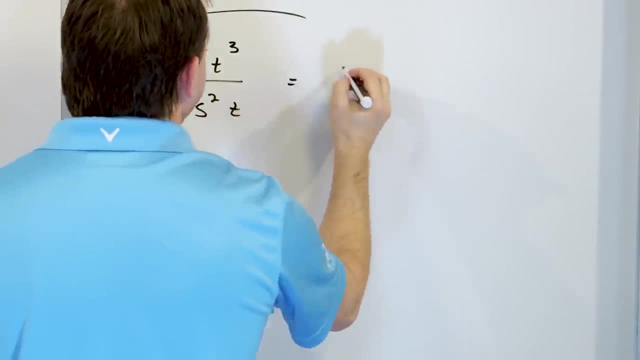 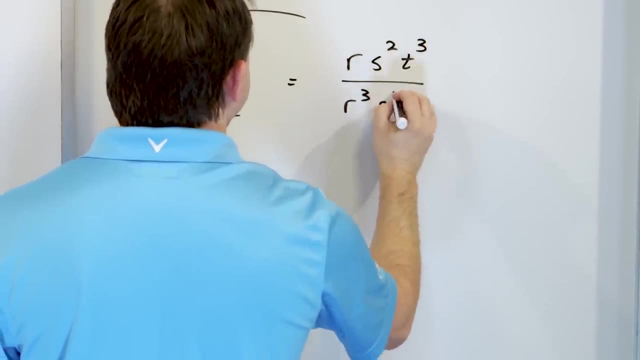 So now we have three variables instead of just two. I'm going to rewrite everything so I don't mess anything up. r s t cubed over r cubed s squared t. All right, so we look at the r's. We have one r and three r's. 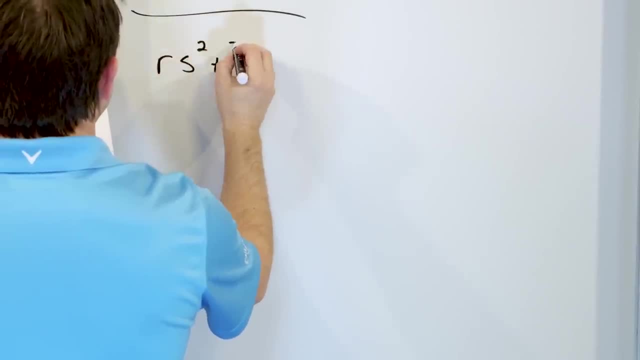 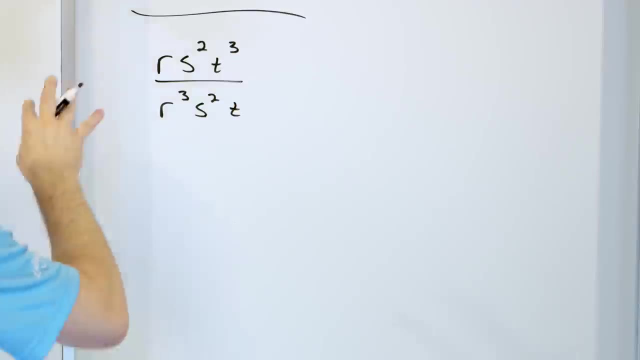 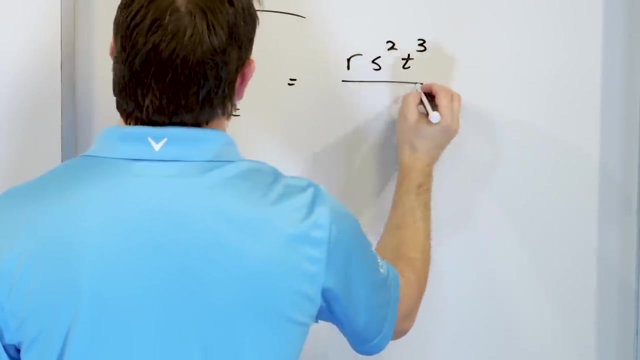 Final problem: r times s squared times t cubed over r cubed s squared t. So now we have three variables instead of just two. I'm going to rewrite everything so I don't mess anything up. r s t cubed over r cubed s? 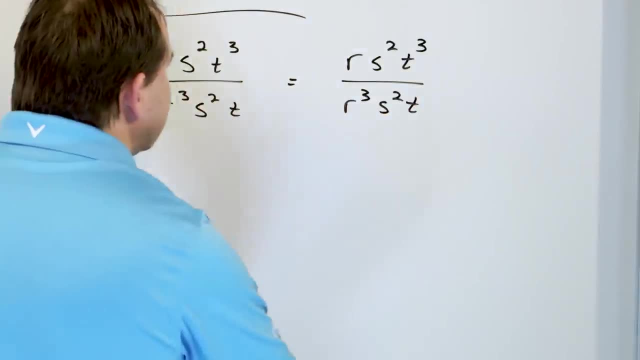 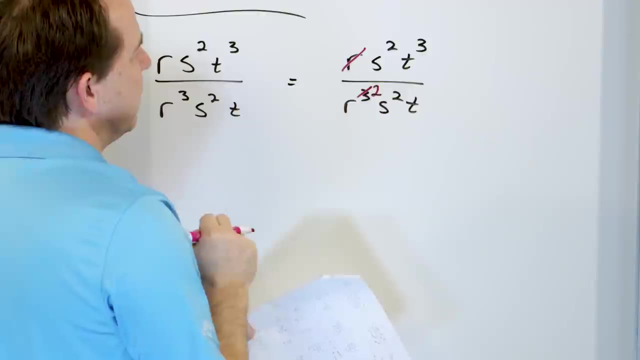 s squared. t All right. so we look at the r's. We have one r and three r's, So the single r can strike out with this, giving me two r's left over. I have an s squared and an s squared. 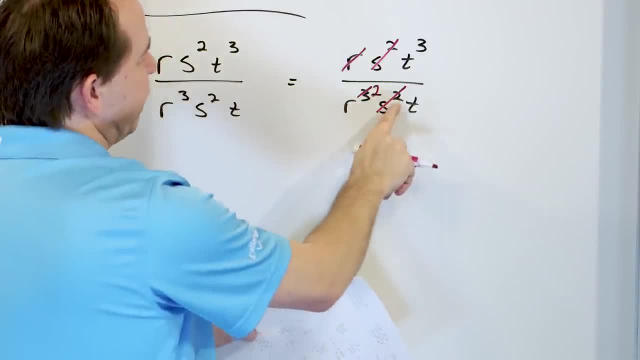 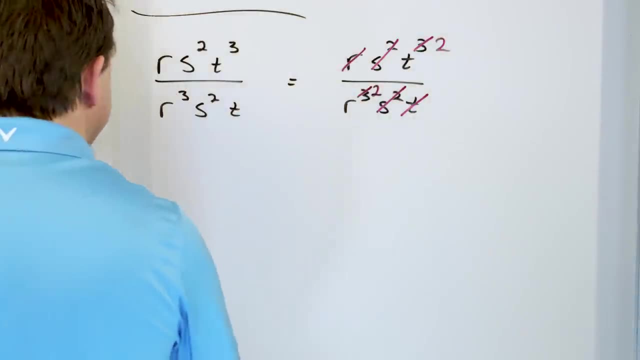 so the entire s squared can cancel with the entire s squared. Notice, I struck through the whole thing, so it's gone. One of these t's can cancel with one of these t's, leaving me two left over in the final answer. So the final answer that I'm going to get. I have no r's left. 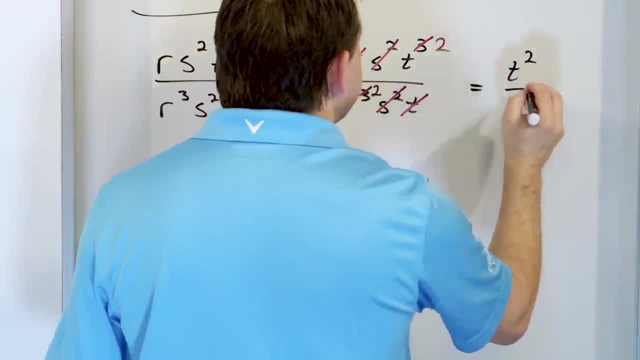 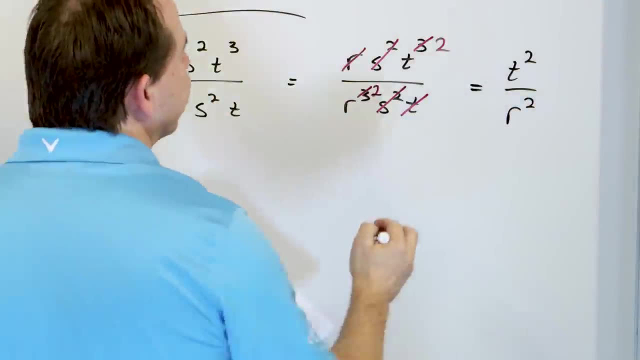 no s's left, but I do have a t squared on the top And on the bottom I have an r squared, but I don't have any s's or t's, so it's going to be r squared. Let me double check: t squared over r squared. that's the final answer. 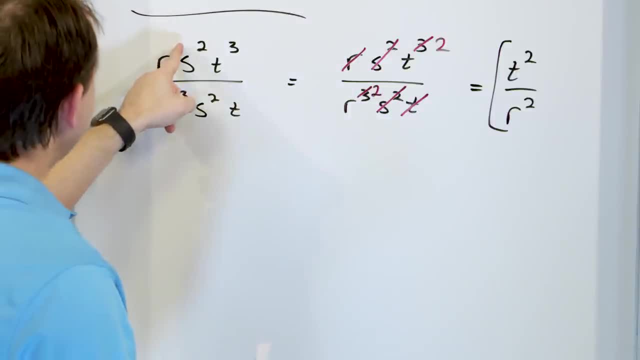 Now let's look at it by subtraction. What we have here for r's, let's just do it down here: r over r? cubed. If this was the problem, I told you you can subtract exponents, So you have r. 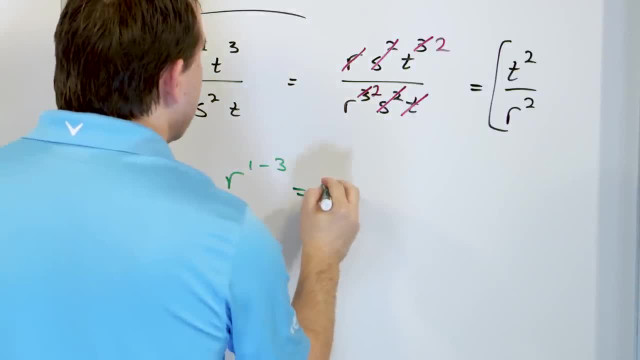 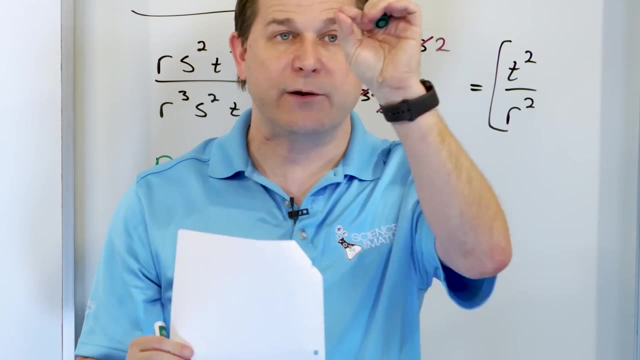 one minus three, one on the top minus three on the bottom, r to the negative two. I told you we haven't done negative exponents, but when you see a negative exponent it just means that it really lives downstairs as a positive version. So negative exponents. 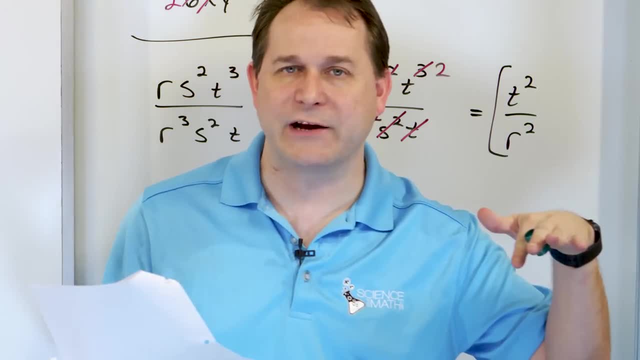 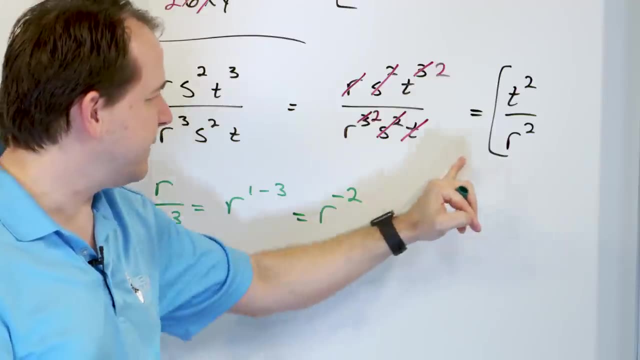 are a way of writing fractions without really putting a fraction bar right. You can write it as a negative exponent or you can just move it downstairs and make it positive. That's why it lives down here. So when you see this, it means it really lives downstairs For the s terms. 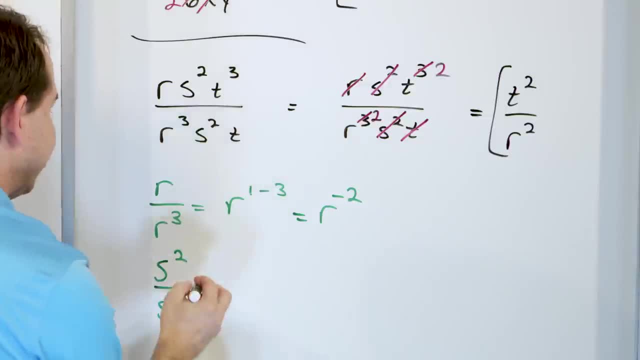 it would be s squared over s squared. That's just the s terms, right, Which is s two minus two, which is s to the zero. And we're going to do a lesson on this, but I'll give you a preview. Anything raised to the zero power is one, So that's why there's no s's. 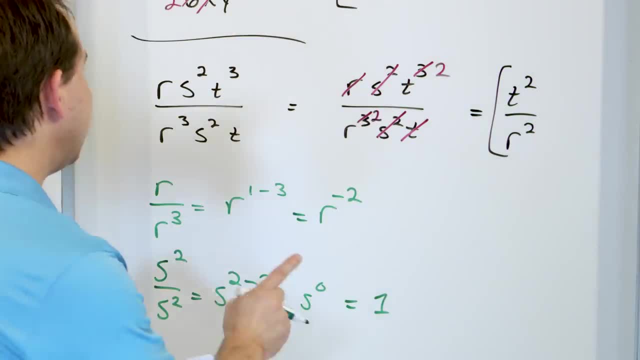 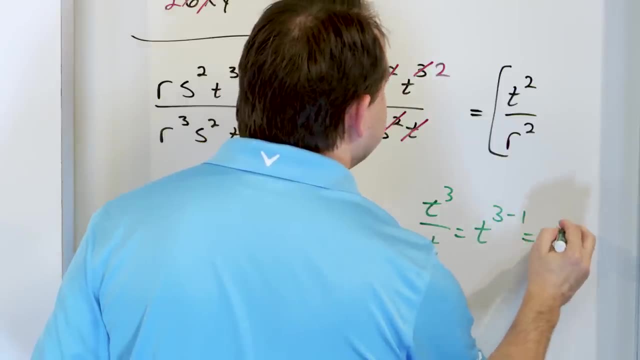 in our final answer, because it all went away to one And then finally we have t. So we have t cubed over t, which is t to the three minus one, which is t squared, And we have t squared in our. 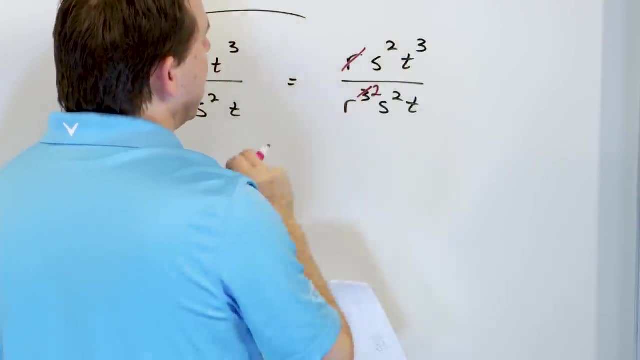 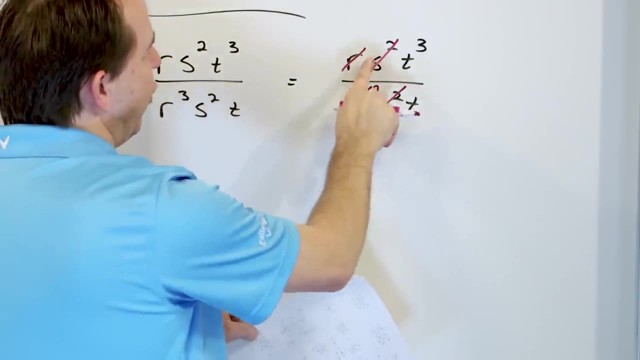 So the single r can strike out with this, giving me two r's left over. I have an s squared and an s squared, So the entire s squared can cancel with the entire s squared. Notice, I struck through the whole thing, so it's gone. 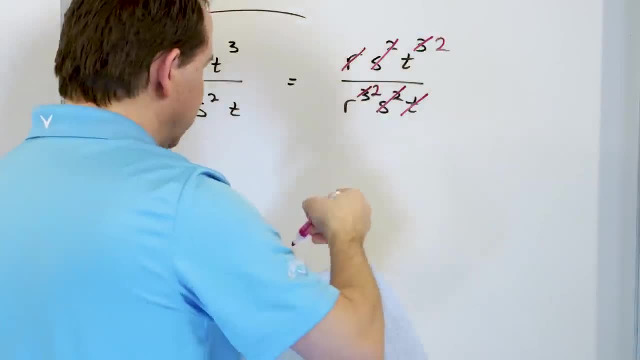 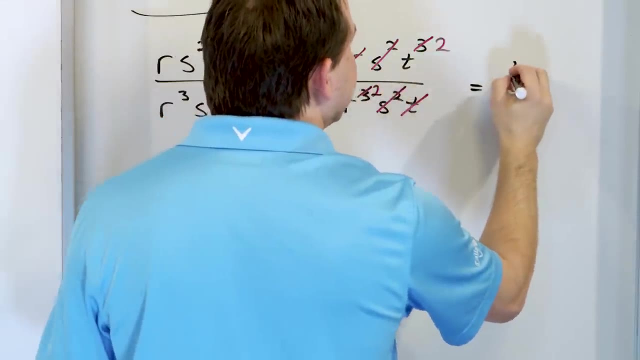 One of these t's can cancel with one of these t's, leaving me two left over in the final answer. So the final answer that I'm going to get: I have no r's left, no s's left, but I do have a t squared on the top. 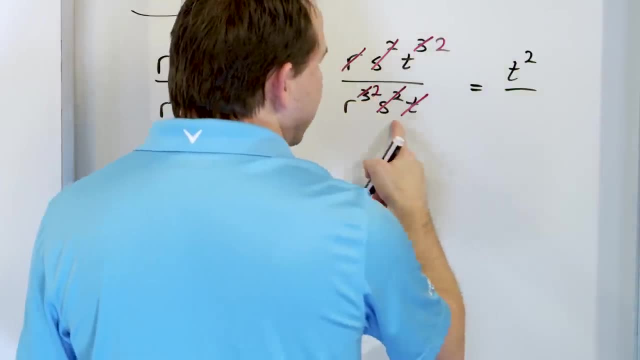 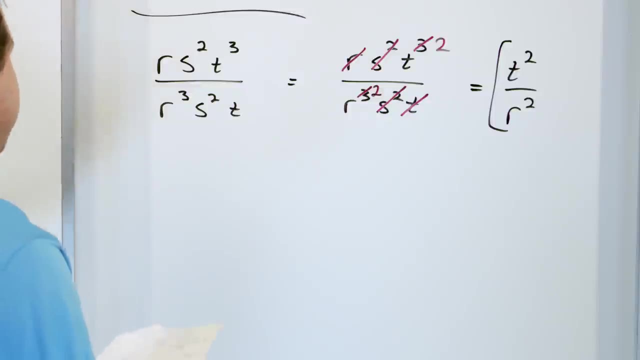 And on the bottom I have an r squared, but I don't have any s's or t's, So it's going to be r? squared. Let me double check: t squared over r squared. That's the final answer. Now let's look at it by subtraction. 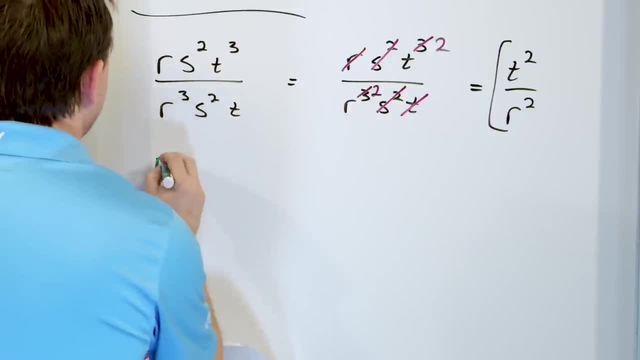 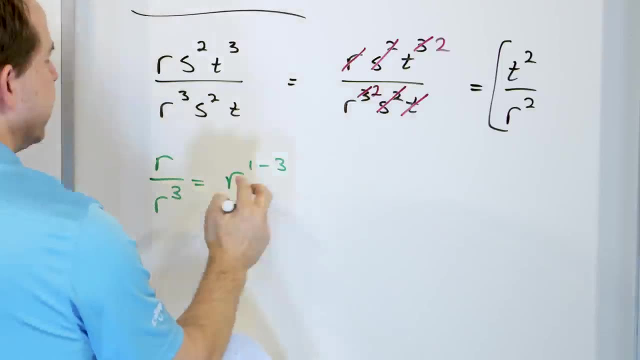 What we have here for r's. let's just do it down here. r over r cubed. If this was the problem, I told you you can subtract exponents, So you have r one minus three, one on the top minus three on the bottom. 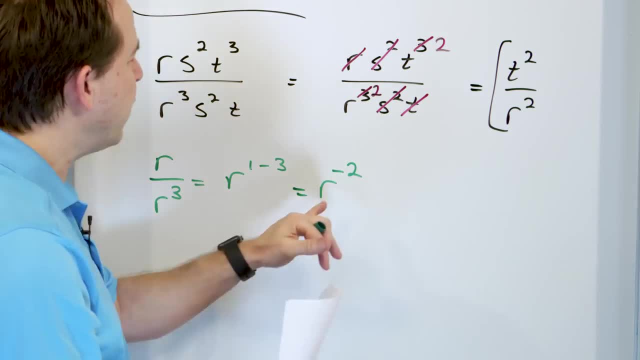 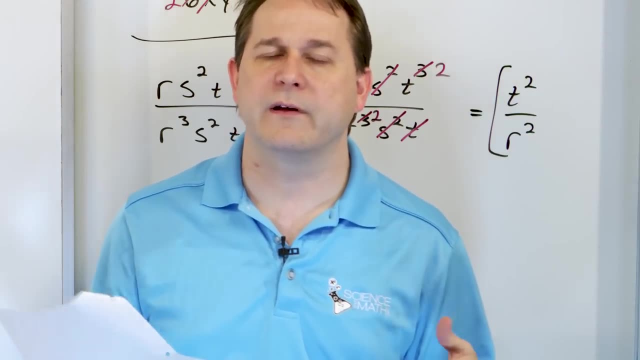 So you have r to the negative two. I told you we haven't done negative exponents, But when you see a negative exponent it just means that it really lives downstairs as a positive version. So negative exponents are a way of writing fractions without really putting a fraction bar right. 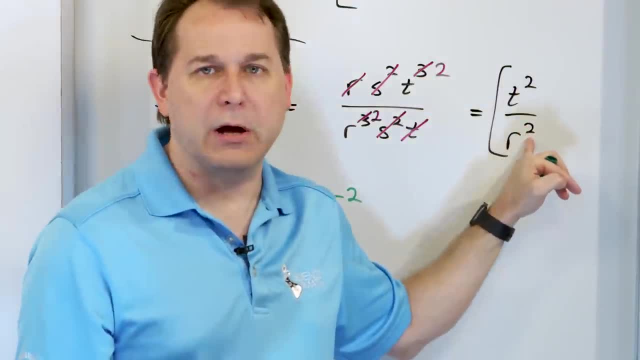 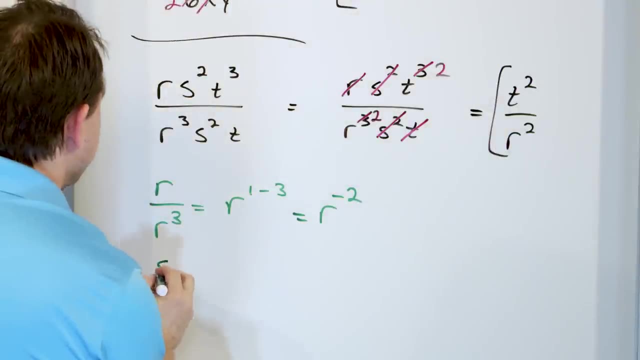 You can write it as a negative exponent, or you can just move it downstairs and make it positive. That's why it lives down here. So when you see this, it means it really lives downstairs. For the s terms, it would be s squared over s squared. 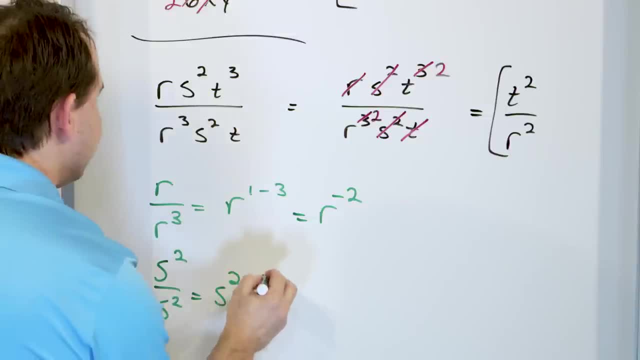 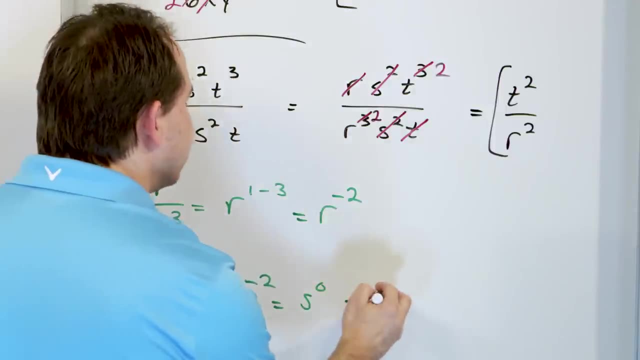 That's just the s terms, right, Which is s two minus two, which is s to the zero, And we're going to do a lesson on this later on, but I'll give you a preview. Anything raised to the zero power is one. 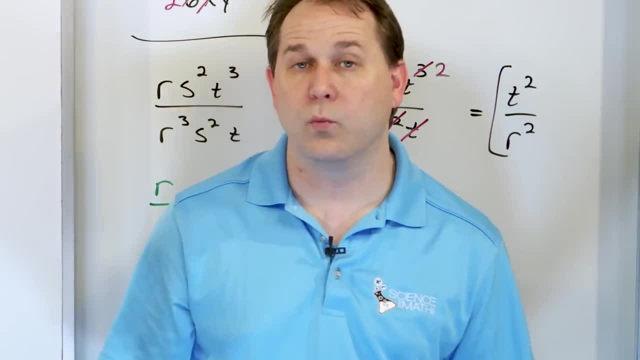 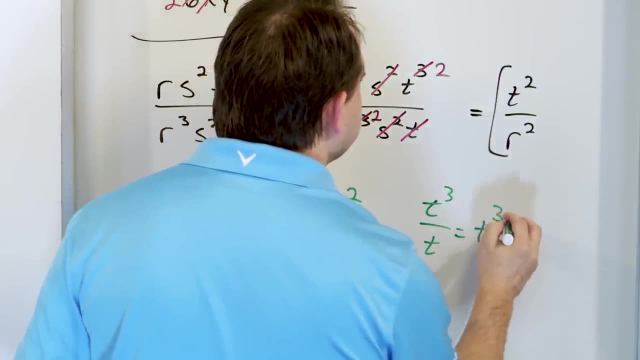 So that's why there's no s's in our final answer, because it all went away to one. And then finally we have t. So we have t cubed over t, which is t to the three minus one, which is t squared. 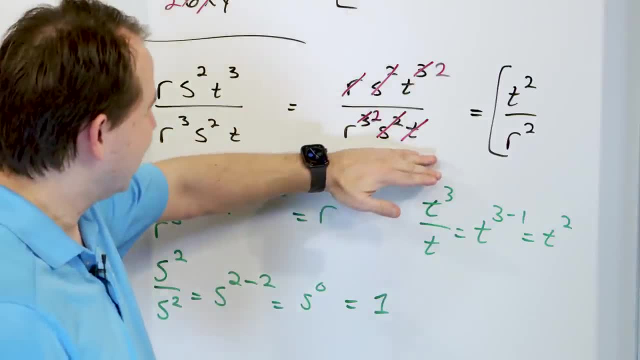 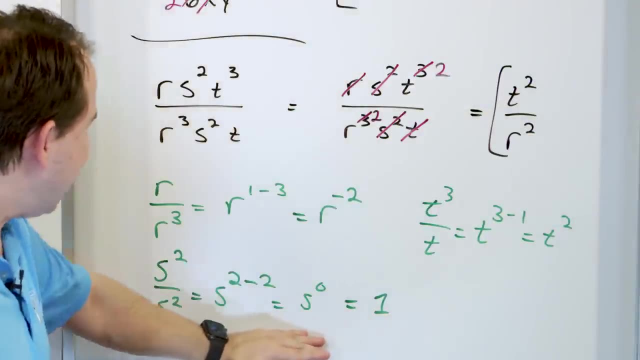 And we have t squared in our final answer. So if we did not do this, canceling what we would get for the t terms? we would get t squared, which means he lives in the numerator. We would get one for the s terms, which means he disappears completely. 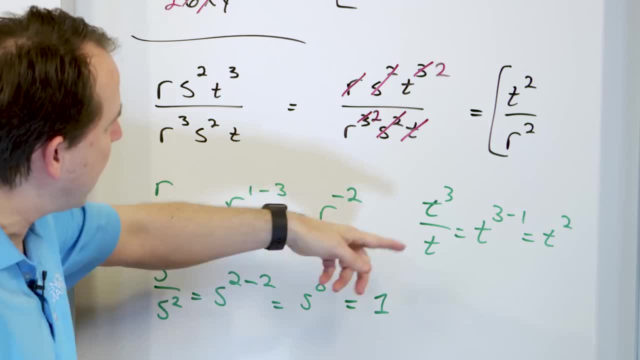 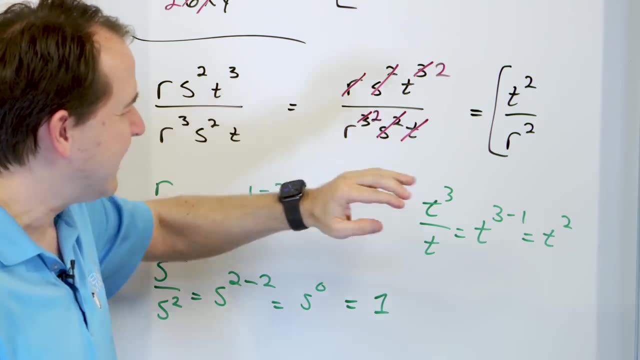 And for the r terms, we would have an r to the negative two, which means he lives in the bottom as r squared, which is exactly what we've gotten here by using the cancellation method. I prefer for you to do things like this, by canceling initially. 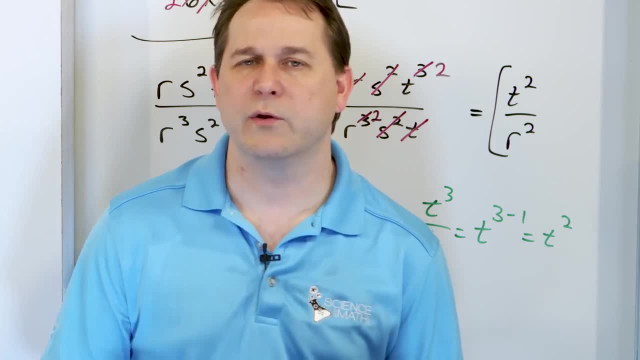 and then as we get a little more practice down the road with negative exponents, then you can do it any way you want. So make sure you understand this. It's very important for you to get paper out and not just watch me do these problems. 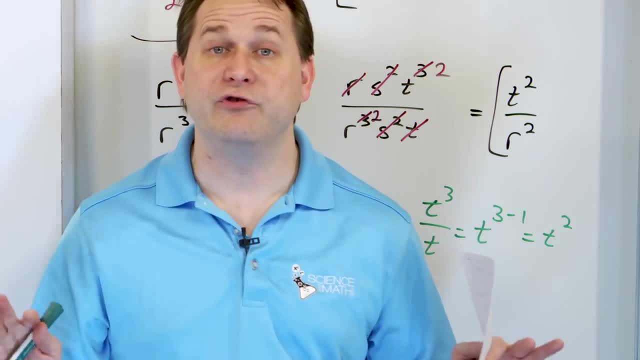 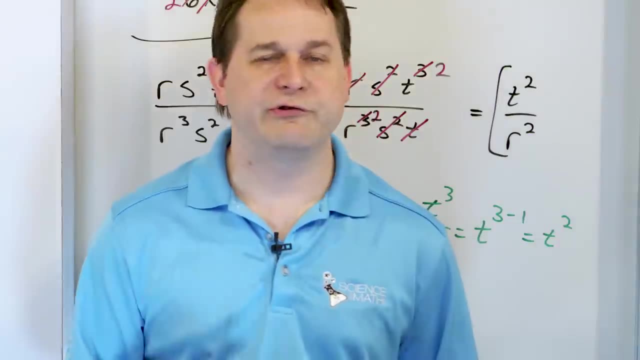 This is my own paper. Go back through these problems, write them down yourself and do them yourself. When you have confidence in what's going on, then follow me on to the next lesson. We're going to do more problems with quotients of monomials in algebra.